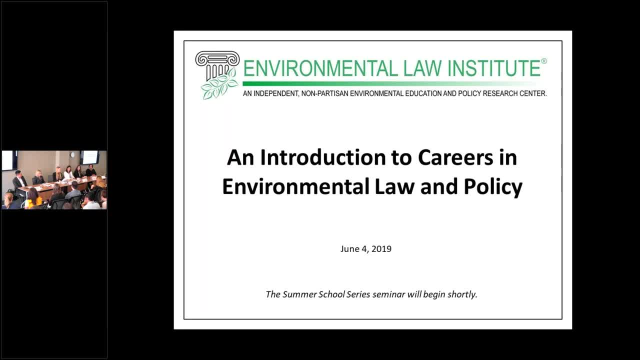 Kathleen is the senior manager of environmental policy and wholesale market development at Exelon. She focuses on energy, electricity, climate and environmental policy as a specialist with vast experience in regulatory and legislative strategy development and implementation. Kathleen, we're glad to have you here. Rachel is an attorney advisor in the Office of Environmental Policy and Development and is a senior partner at the US Department of State on the Environmental Policy and Development. She is also a senior manager of the US Department of State on the Environmental Policy and Development. 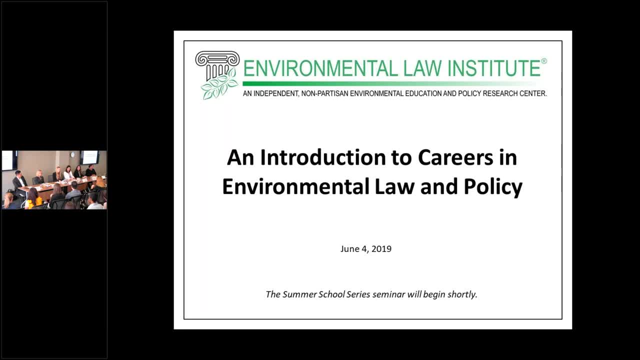 of General Counsel at NOAA. Prior to working as attorney advisor, she was the student attorney at the Georgetown Law Institute for Public Representation Environment Section and a law clerk with the Environment and Natural Resource Division at the Department of Justice. Welcome Rachel Kendra is the chief of staff for Congressman Butterfield in the House of. 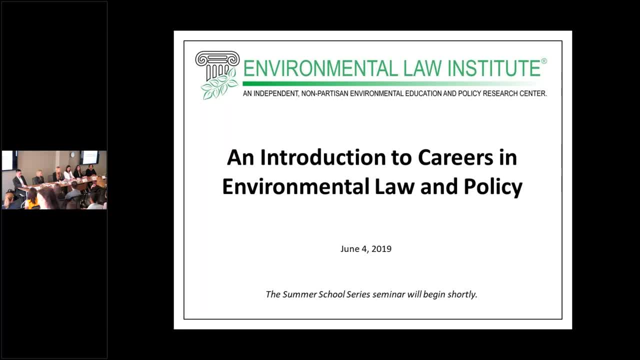 Representatives With an extensive educational and professional background. we have also been delighted to have Kendra previously lend her expertise to ELI's annual Eastern Boot Camp and help plan a public program on environmental justice. Thanks for being such a great part of ELI, Kendra. So, as you can see, we have really fantastic panelists with a wonderful variety of 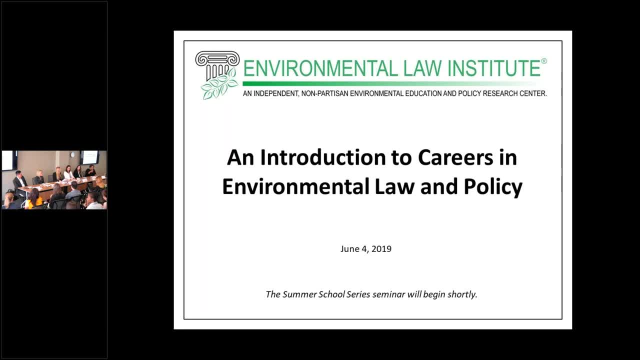 backgrounds, experiences and expertise. Thank you all for kicking off the 2019 Summer School Series With that. I would like to warmly turn things over to Toby to get us started. Great Thanks, Caitlin, for having me on this panel. I was telling Caitlin a little bit earlier. 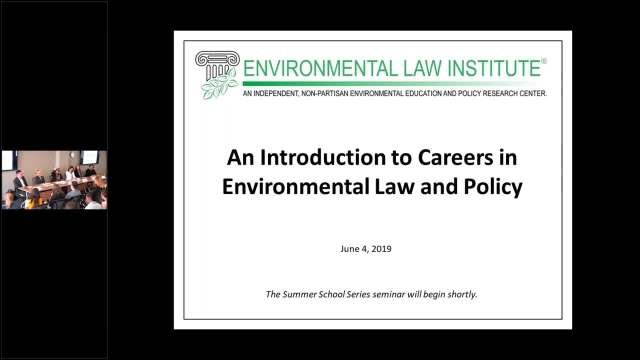 that I can't really remember for how long I've been on this panel, but I'm going to tell you how long. but it's been a personal goal of mine to be on this panel, so I'm feeling very validated today, But I think primarily to help raise awareness of this particular 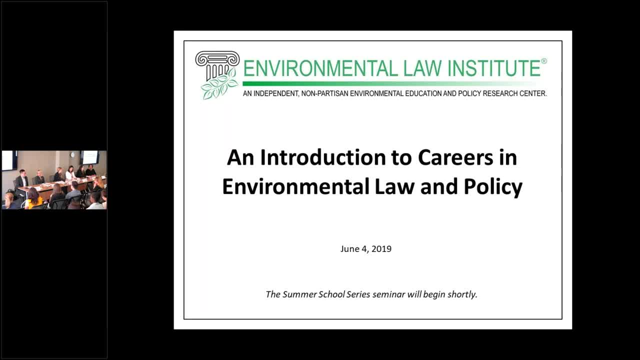 career that I stumbled upon, transactions-focused environmental practice, which I don't think a lot of people really think about when they think about going to law school and when they think about pursuing a career in environmental law. And then I'll also probably just talk a little. 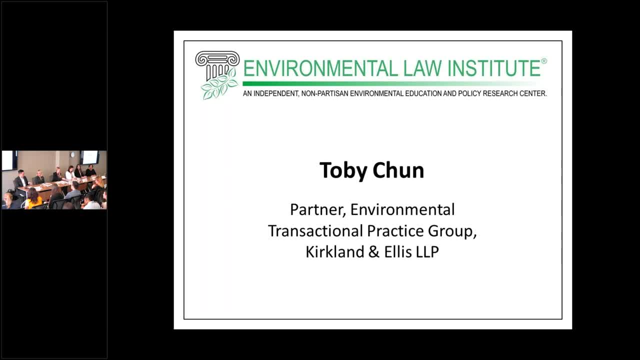 bit about my career path, because I guess my other goal is to sort of, to the extent that you can, you know, learn from how I sort of tried a bunch of different things and eventually found the career that I found to be the best fit for me, hopefully to help you know, if you can like. 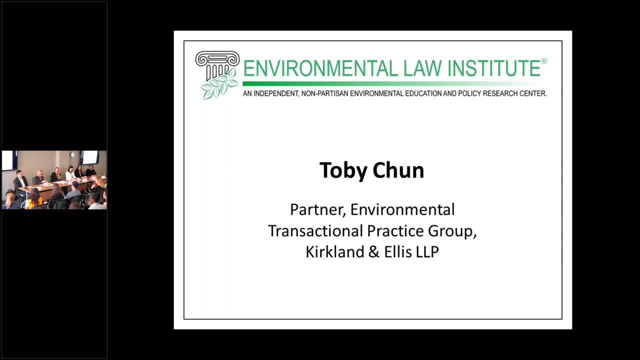 not repeat some of the mistakes that I've made. that would be good too. So the job is: we have a group at Kirkland & Ellis. It's the Environmental Transactions Practice Group, and it is a group of about 21 attorneys now in four different offices- DC, San Francisco, Houston and Dallas- and we 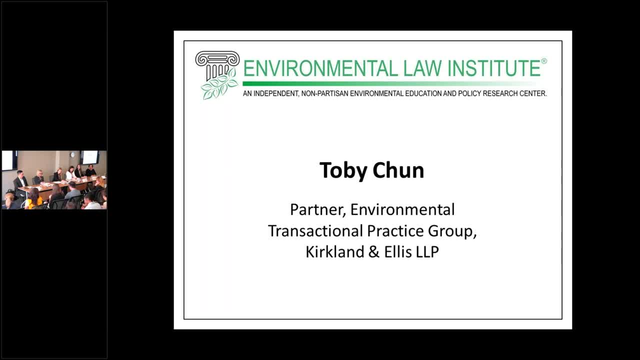 are a group of environmental lawyers who primarily support, provide environmental support for transactions from our various transactions-based practices. So private equity, mergers and acquisitions. that's probably the biggest portion of what certainly I do and probably my current the group. we also do M&A work for public companies. we do. we provide support to 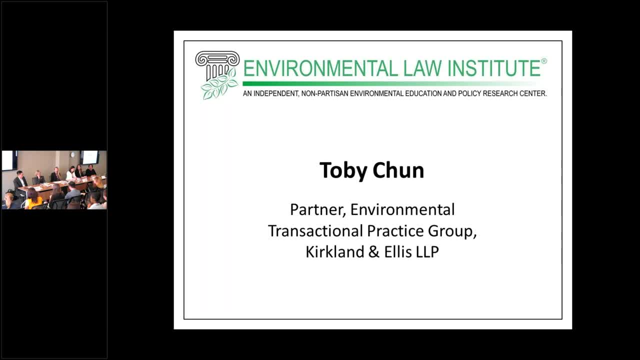 our real estate group for their real estate transactions. we've to a lesser extent what we have. other people have different specializations, but we have people who support our bankruptcy and restructuring practice. and then when Kirkland added its oil and gas practice down in Texas several years ago, our 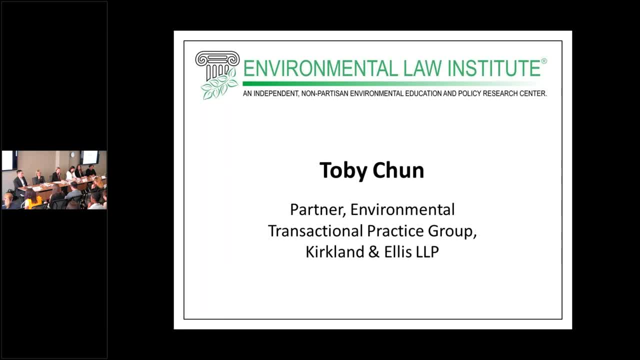 group expanded to provide support to that and actually with Kirkland's growth we find ourselves being stretched in a lot of different directions. we have a project finance group that has come on board so we're providing environmental support in that area as well. so you know, as as narrow as this career of 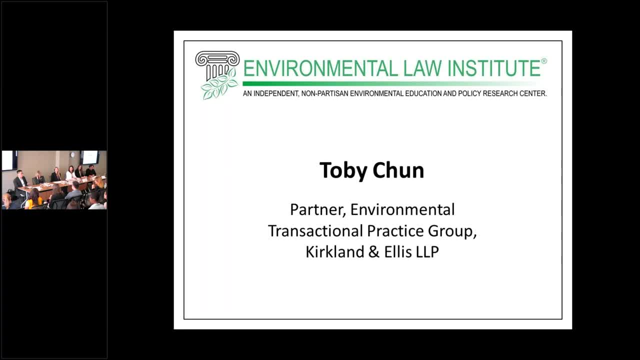 environmental transactions might seem. there's a huge variety of work within that space and you know, I would say the nuts and bolts of what we do is most of our clients are buying and selling businesses in the same way that an individual might buy and then later flip a house. you buy something, you look. 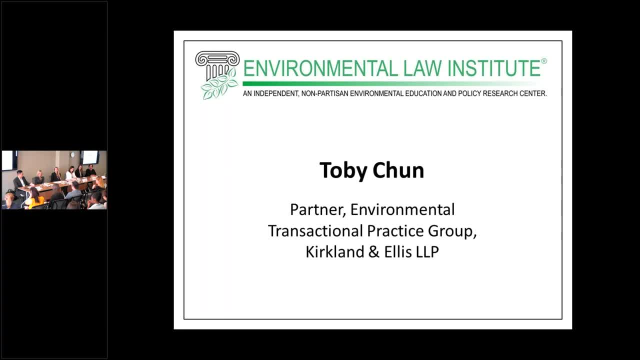 to improve its value, and then you look to sell it in a certain number of years for profit, and so they are the experts at doing that, but they're not necessarily experts in environmental risks and liabilities. so that's where we come in. that's our job is to sort of diligence. the target business or the 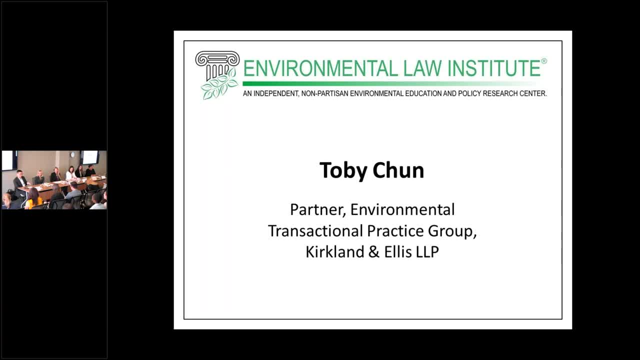 target properties, evaluate its environmental risk profile, identify the environmental risks and liabilities associated with their business, their facilities, oftentimes their history. sometimes you have targets that do something now, but they did something very different back in the past and something with a much higher level of environmental risk associated with it. 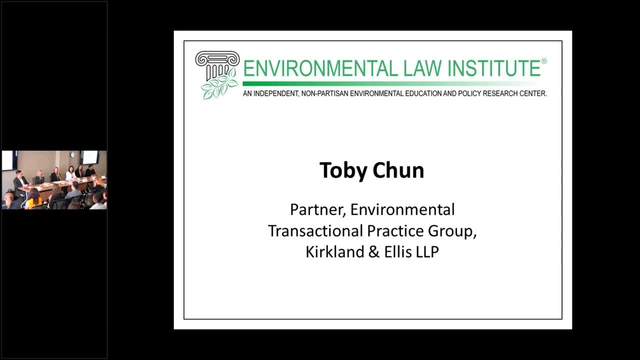 and then so we. we advise our clients on what these environmental risks and liabilities are. we give them advice on how to manage that, whether that's getting an indemnity from the seller or if it's getting environmental insurance. I would say you know a lot of the key value that we bring to the table is one being that. 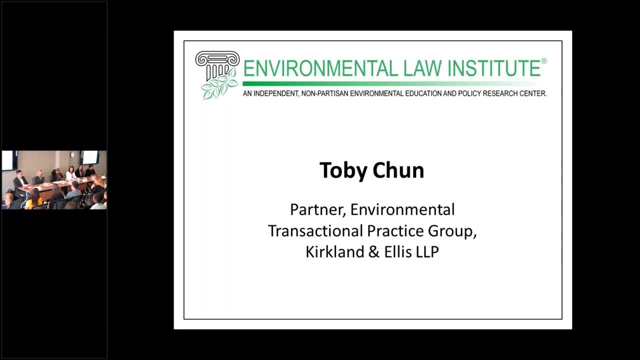 bridge between the scientists or the consultants and these business folks who are, you know, doing transactions, because in any deal that has, let's say, a heavy environmental component, like manufacturing or hazardous waste management, you are undoubtedly going to be retaining an environmental consultant to do a more technical review of the operations and 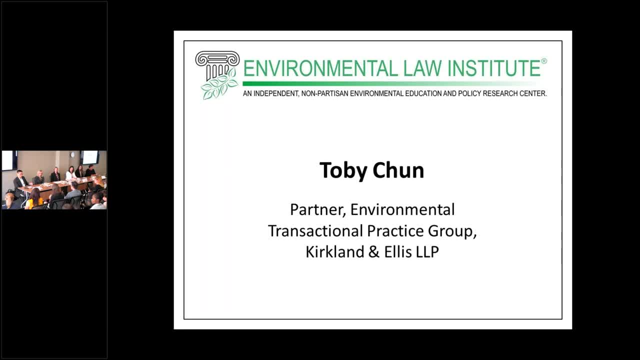 the facilities, but they are scientists and they have a certain lens and they do a lot of different work, not all of which is necessarily related to transactions, but there are consultants who specialize in coming into this transactional space and doing like a transaction level review of the 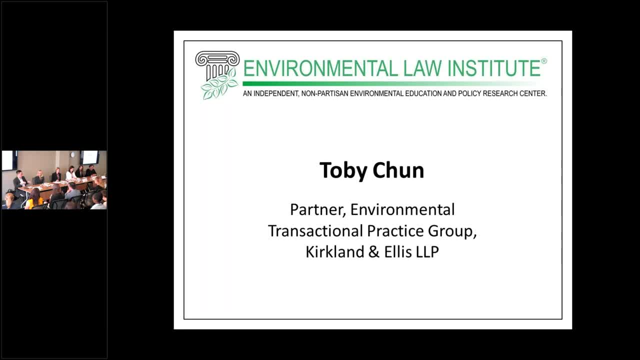 environmental risks and liabilities. so not necessarily the deep dive that you'd have if they were doing like a two-week comprehensive multimedia audit of a company and their compliance, but it's sort of more high-level and big-picture focused and so they present their findings. but we, it's, it's, it's our. 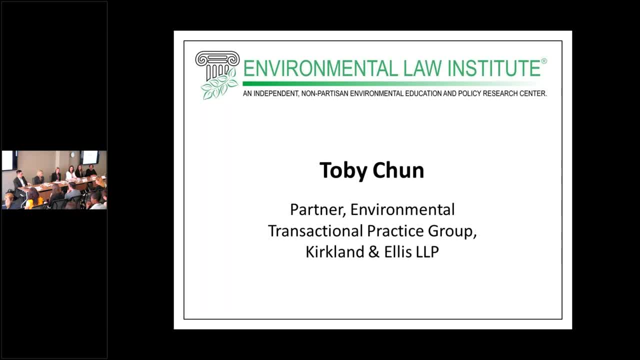 primary job to take those findings and to translate it and present it for a variety of audiences. so there's your client, who are business folks and they have to sort of like a very business focus. they're not interested in the science. they won't thank you for explaining the science, they just want to. 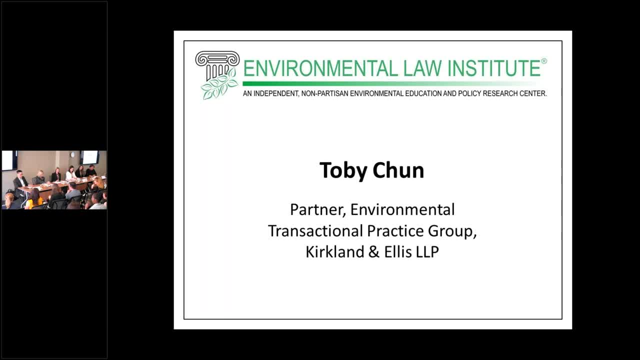 know what it means and how do they make their decisions and how do they protect their interests, then you have- oftentimes you have- a lender. so in the transaction, your client is borrowing money from a lender in order to finance the purchase. so you are then speaking with the lender and, whereas when you're talking to your 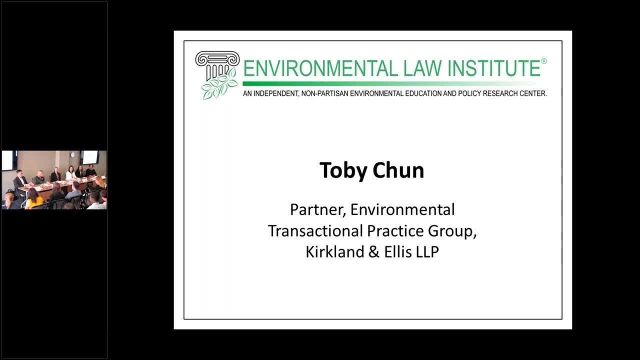 client and you're trying to make sure that they understand the risks associated with the business that they're acquiring. when you go to the lender, the focus shifts and you are sort of more getting them, bringing them up to speed on the diligence that you've done on the target and getting them comfortable. 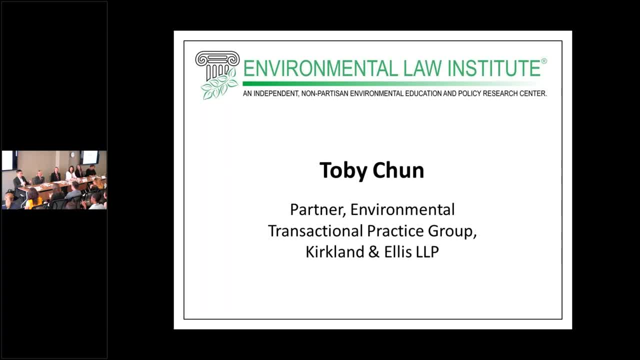 that you've sufficiently diligence that and that there's nothing big out there that's going to potentially cause the target business to go bankrupt and to for them to default on their loan. we're dealing with a lot of insurance these days and not the traditional environmental pollution legal liability. 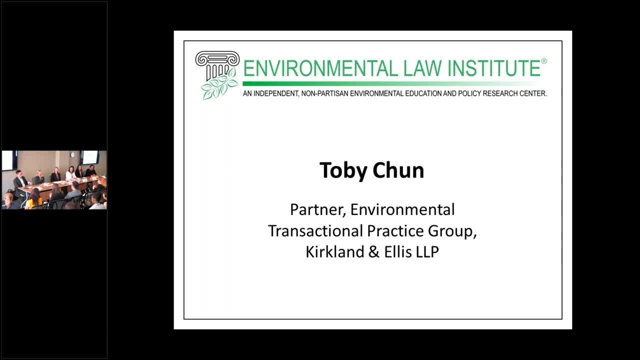 insurance. the really hot thing these days is called representations and warranties insurance. so whenever a seller is selling a business, they'll make a variety of environmental representations and warranties. the target business is in compliance with all environmental laws and regulations. they haven't received notice of any environmental violations or liabilities. they haven't released or exposed anyone. 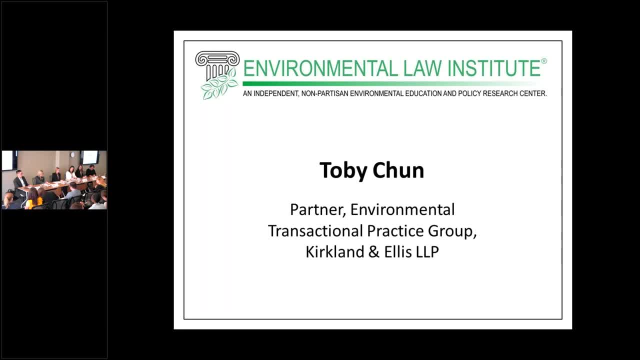 to any hazardous substances in a matter that is given rise to liability. so rep and warranty insurance is very different, and I guess I'll make a long story short. rep and warranty insurance used to just exclude environmental, environmental matters. they just wouldn't cover it. but that's shifted significantly in the last five or 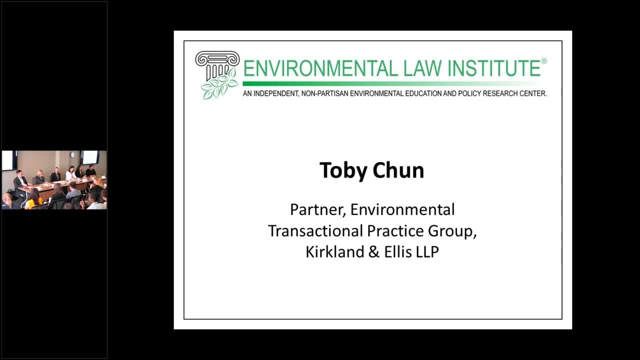 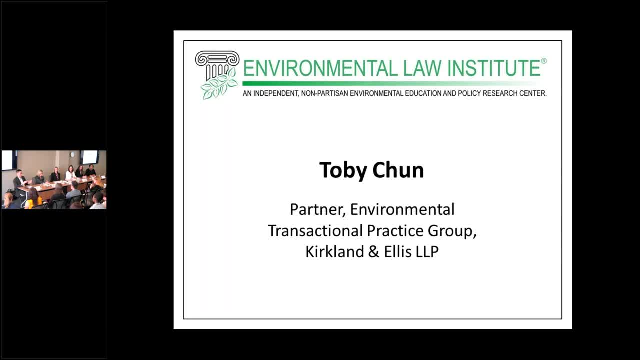 what's market. that's what you'll hear a lot of clients ask. well, you know, we don't need to understand it. we just need to know that what we're getting is market for what everyone else is getting. so that's, that's what we, that's what we do in a nutshell. I'll say a little bit, just sort. 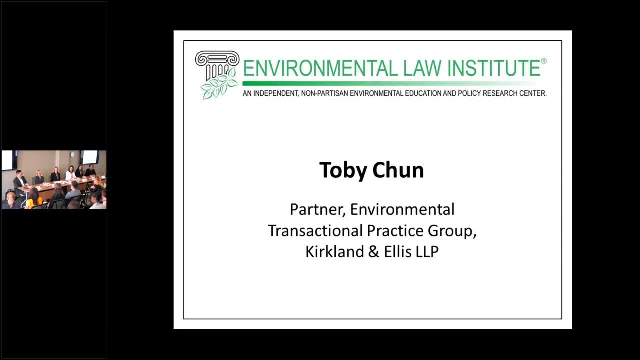 of pop up my path and how I started working in this area. I actually because I've been at Kirkland DC since 2004 doing this work. but I've been at Kirkland DC since 2004 doing this work. but I actually started off at Kirkland's Chicago office out of law school in 1996. 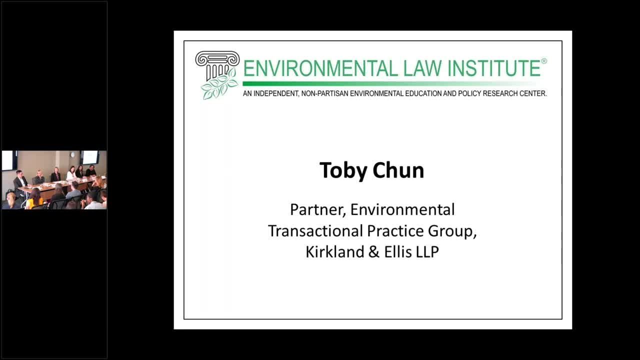 as a patent litigator and you know, after a couple of years I realized that because I wasn't crazy about research or writing or arguing, perhaps litigation wasn't the best fit for me. so I then moved to Wilson Sun Senior University in California and I joined their biotech licensing group and I worked there for. 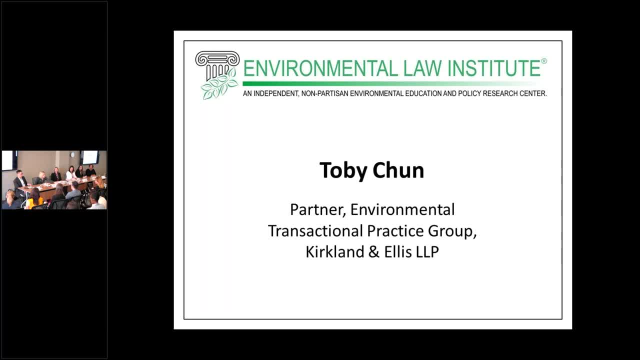 a few years and again, super, super interesting work, very cutting edge, working with great people. but I just really didn't like the the biotech aspect, and I think the trap that I fell into coming out of law school is that I pursued the career path that I thought I should pursue, as opposed to the one that 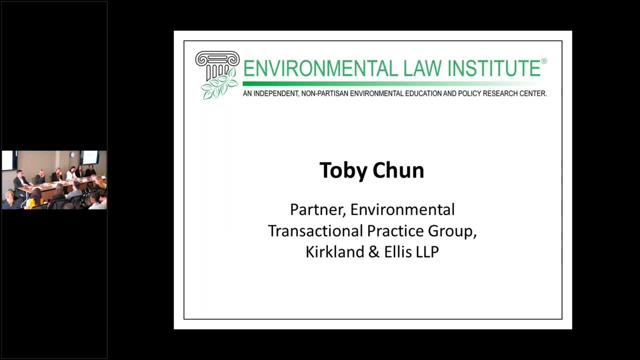 most interested me. I went with the one that was like the highest profile and the most perceived upside, which was patent litigation, which is probably still patent litigation, but the you know, working in a private practice, the uh, it can be stressful, it can be time intensive and you just 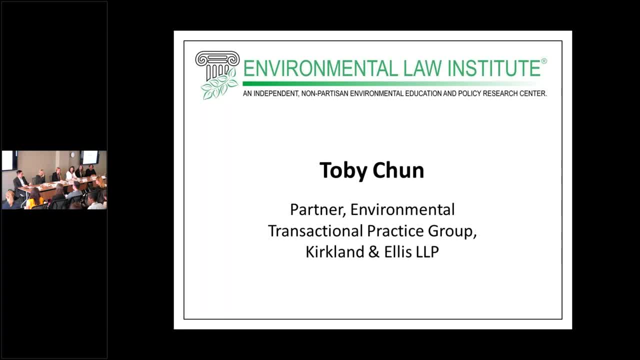 you, I couldn't afford to not be really interested in the work that I was doing. yes, I could force myself to do that, but why? why deal with that cognitive dissonance? so I ended up moving to DC in 2001 and eventually joining Chad. born and Park, a general technology transactions based practice. 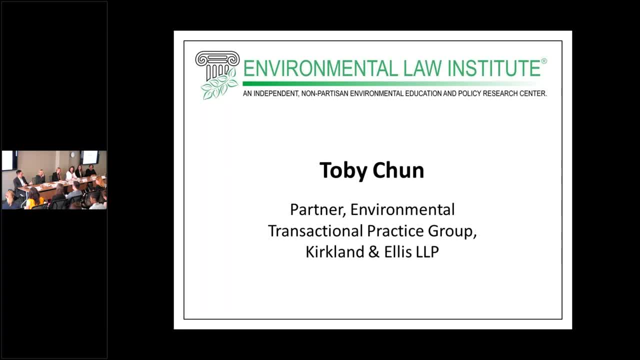 group again still not the greatest fit. I guess I should explain. my background is in science, I had a biology bachelor's and I did a master's in environmental engineering, which is why I thought I could and should do the the IP work. but- and I guess fortunately for me, this is a bit happenstance- but the group that I 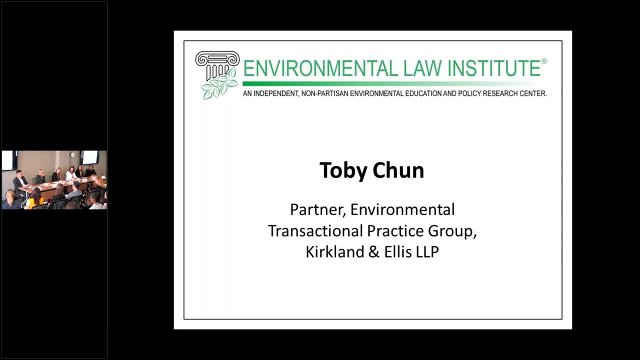 joined was slow. the managing partner of that DC office was an environmental lawyer and he put me on my first transaction, a sale of 36 power plants doing the environmental sell-side diligence. and that's how I discovered that I enjoyed the transactional work and I was able to get my first transaction. and I was able to get my first. 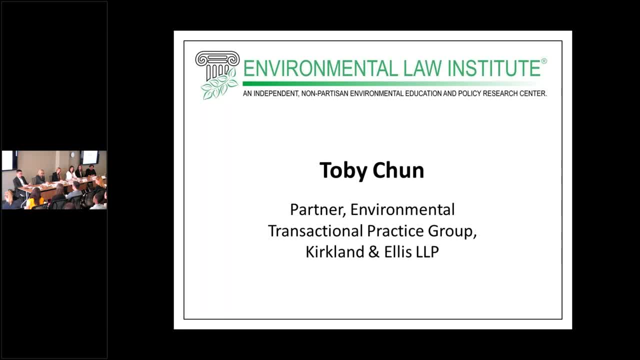 and I enjoyed returning to my environmental roots and and one of the bidders in that auction process was represented by Kirkland, my old firm. so that's how I discovered. it's amazing. I worked in the Chicago office for two years and didn't even realize they had this environmental transactional. 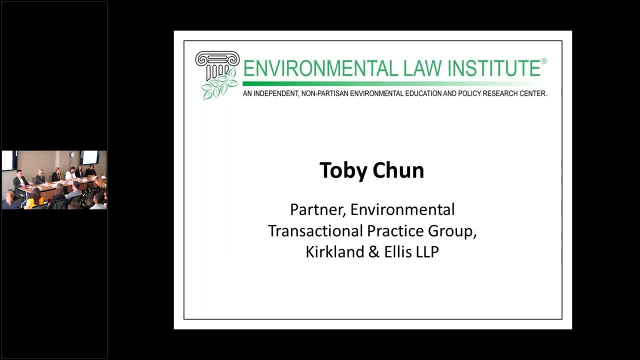 practice here in the DC office, although in fairness I'm not sure I would have known then. but that's what I wanted to do. I had to just sort of figure that out on my own. so I came back and I was a little bit, you know, nervous because again for the 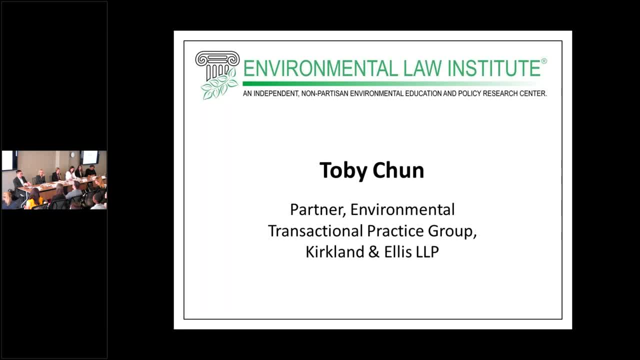 same reasons that I sort of mentioned before, that it seemed very niche and very specialized and I was thinking I probably don't have many more moves left. I need to. I need to really think that I'm going to enjoy it, but I had enough of a basis to think that this was a much better fit for me and that's and that's. 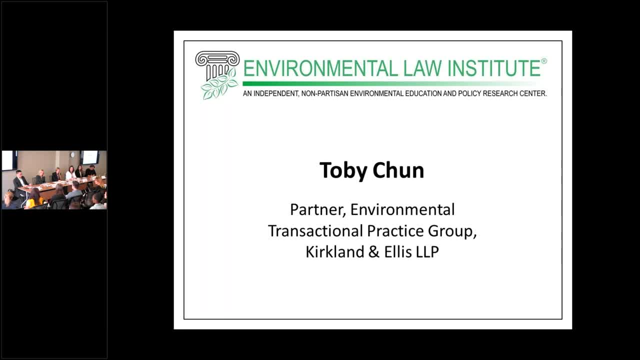 definitely panned out. I really do enjoy. you know what I do. I'll say a few more things about sort of why I like the job and and why as compared to the other jobs that I had, but that will be like a illustration of the things to consider there are. ultimately, it's going to come. 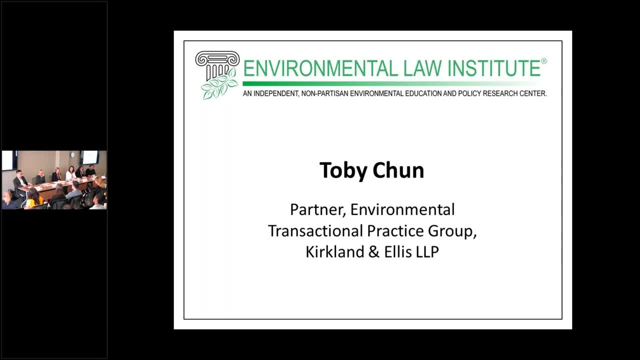 down to fit. and what do you? what do you like? because I have, you know, like my college law school roommate was born to litigate. he just loves it. you know, he. I was a little bit confused about what things would be right for him, and I think you know, you know I'm not going to be the only person who goes to sleep. 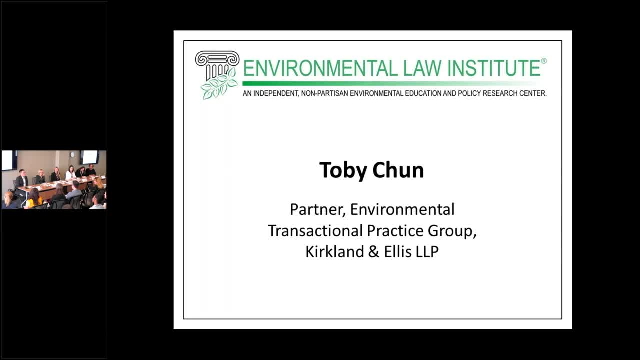 thinking about how he's going to get the other side and wakes up in the morning thinking the same exact thing, and that's why that's a great job for him. it I didn't enjoy it. you know. I always had a feeling that even my client when I was a litigator didn't particularly like me because I 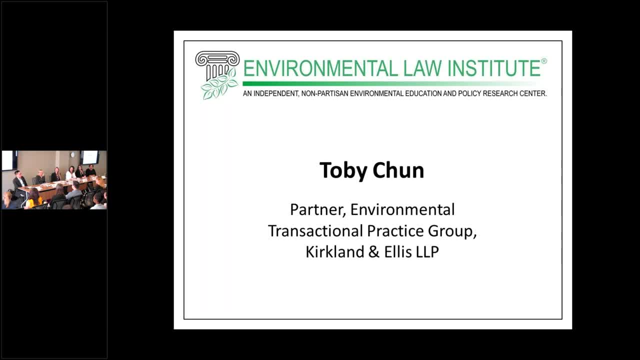 was a constant reminder that they were being sued for something. working on transactions concept, you know both the buyer and seller have to want to do the deal or the deal is not going to happen. They both have to feel like they're winning. So, really, you know what I really enjoy. 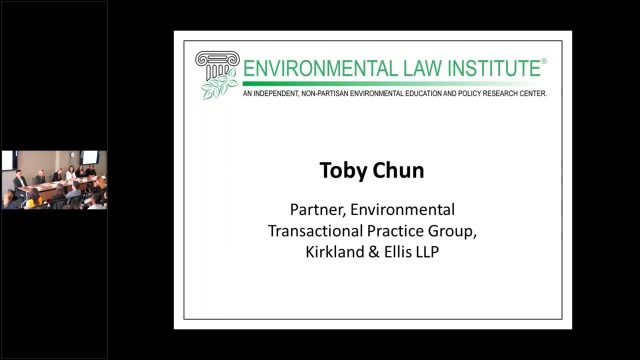 also because I can't compartmentalize. when I argue like I get upset just ruins my day. So you know, what I really enjoy is that my job is to facilitate, to facilitate a transaction And when there is a big environmental issue and it's kind of it's in the early stages. 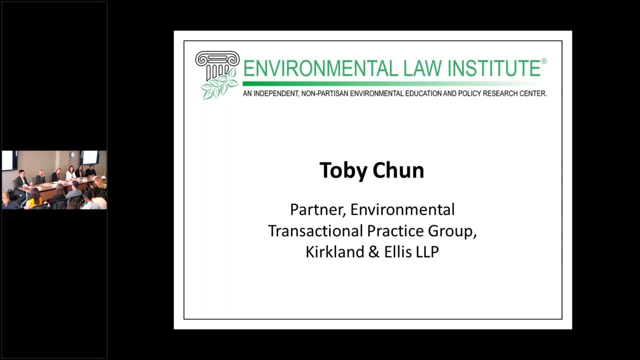 and no one knows how much it's going to cost. that's really tricky. Those are the types of issues that will really impede a deal if you can't figure out how you're going to allocate that risk between the buyer and the seller in a way that both sides find to be acceptable. 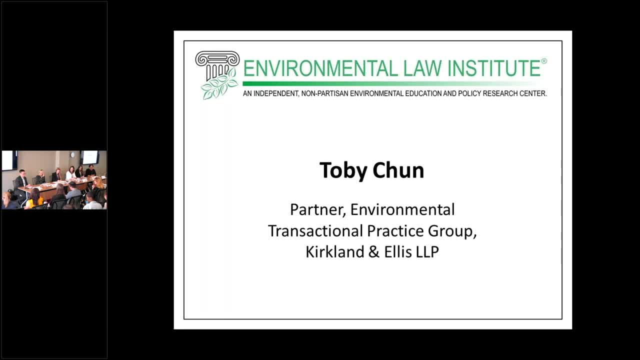 So I enjoy that I also. these are going to be a little bit more sort of like mundane considerations, But I enjoy the. I enjoy the variety and also kind of like the much quicker turnover. So when I was on a lawsuit and as a litigator it was a great, super interesting case. 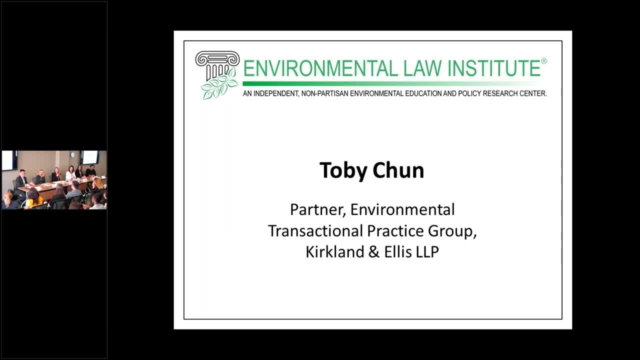 But it lasted the entire time that I was at Kirkland and Atlas Chicago. I mean they go on for years, Whereas transactions you work on those, those occur on a timeline of like weeks Or at most months. So there's just a lot of turnover, a lot of variety. you see a lot of. 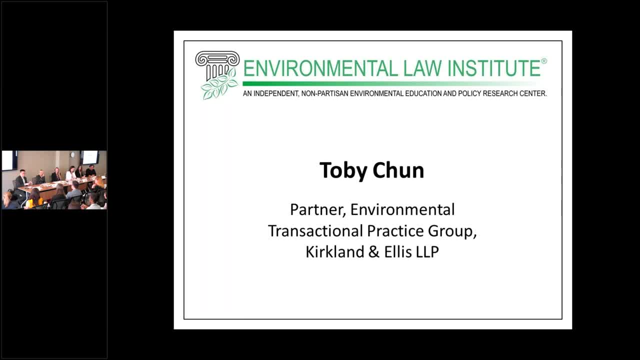 different, a lot of different industries. I mean I work on deals from software companies to hazardous waste management companies and everything in between and in all different kinds of jurisdictions. So it requires an ability to multitask and to juggle. So that's some people. 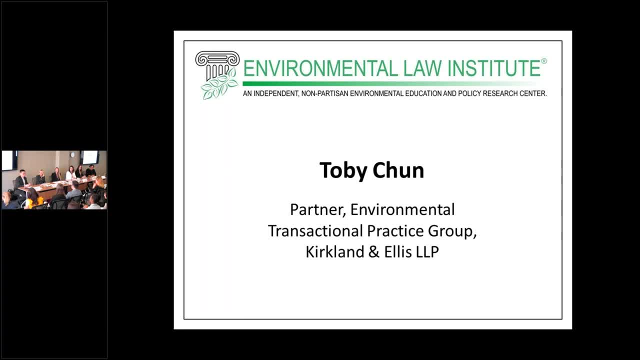 might like that, some people might not like that, But that's what I find super interesting. And then the other plug I'll make is that it doesn't really require any travel, Because when I started working on this in 2004, data rooms used to be physical data rooms where everyone, all the, all the reports and everything. 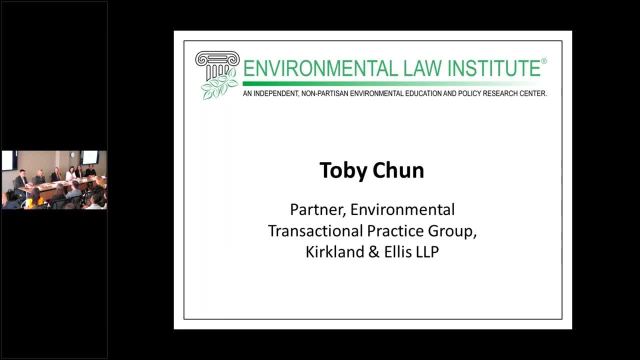 were gathered and you had to go out and sit in a room with other people. All of that went online, So all the documents are reviewed online now. all the negotiations occurred online. So probably the number of business trips that I've had to take because of work, because of a deal, in the 15 years- 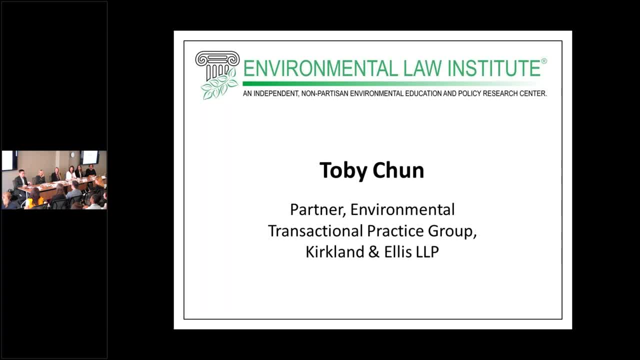 that I've been doing is less than 10.. So I sort of enjoy not having to travel, or if I'm going to travel, I'd like to do it for a reason other than work. Anyway, thanks for letting me share My next. 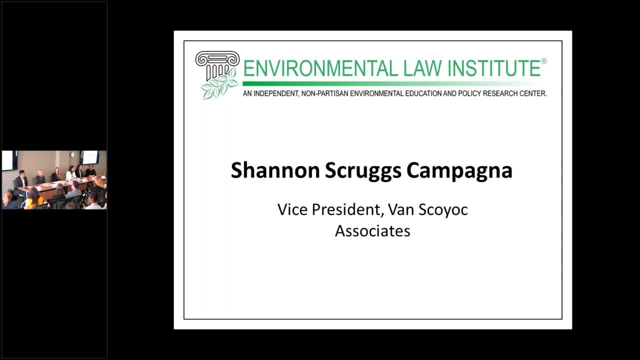 I'm Shannon Campagna. I'm a lobbyist at VanSkoik Associates And thank you for inviting me. I'm really honored to be here And I looked at the background of my fellow panelists and I'm not sure my name must be similar to some other. really, 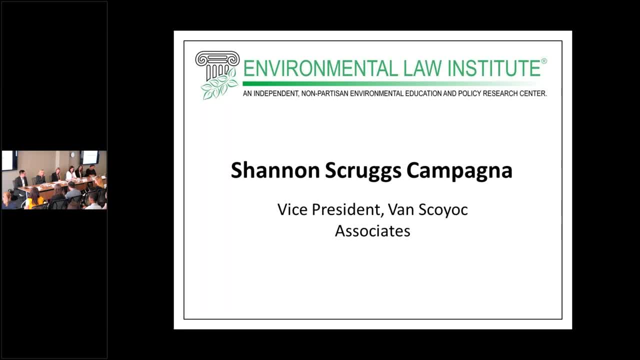 accomplished lawyers, But I'm really happy to be here. I'm the non lawyer. I think I'm the only non lawyer on the panel. You're not a lawyer- Not that there's anything wrong with that- But so I'll be focusing more on that sort of policy side. 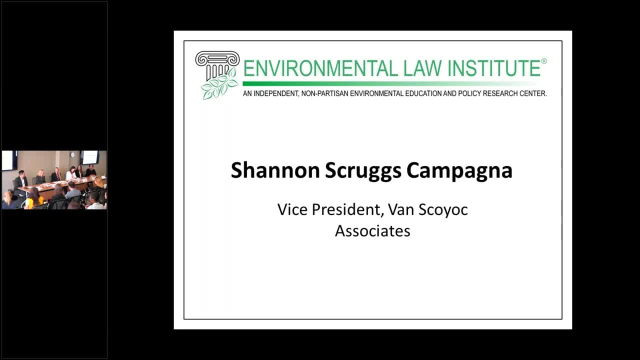 And I think first I'll sort of give you the trajectory of my career such as it is. I went to the University of Alabama and I graduated in 1990 and decided I wanted to move to Washington. I really had not really a clear idea of what I wanted to do or how I wanted to do that. 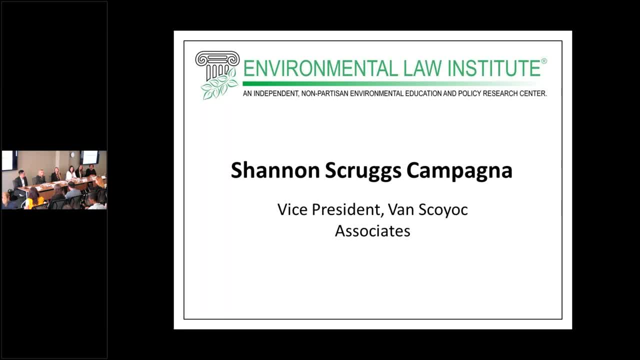 So I commend you all for being so proactive and being here to kind of look at what you're going to do in your careers. So I moved up here and just sort of you know, felt like okay, Washington DC, I've arrived. 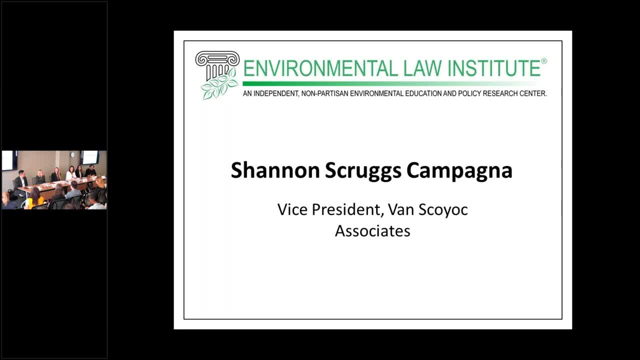 And I had an internship on Capitol Hill. I needed a couple more hours to graduate, So I did an internship for credit with a member of Congress from Alabama And then I had talked my way into and it was talking because there was no email. 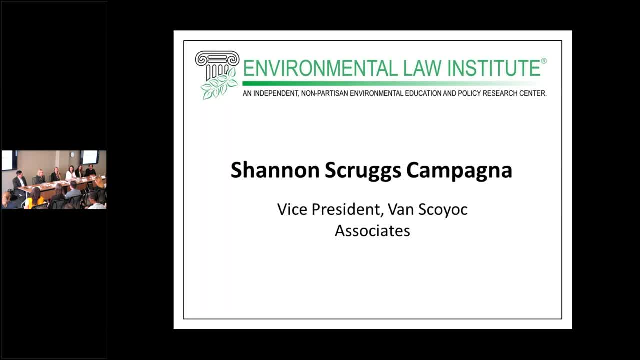 so I was on the phone with this woman. I had talked my way into an internship at the Republican National Committee. There is a very sort of prestigious internship program there called the Eisenhower Internship at the Republican National Committee, which is for children of donors primarily and other sort of high-level Republicans. 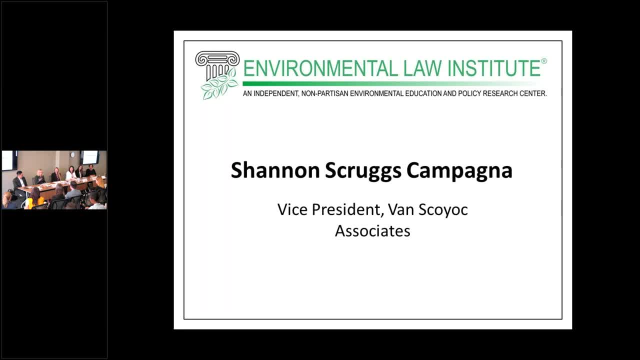 I was not one of those, I was in the back. Lee Atwater was the chair of the RNC at the time And we used to have these big auto pen- And Kendra may remember the auto pens where to sign, But, Matt, you still have one. 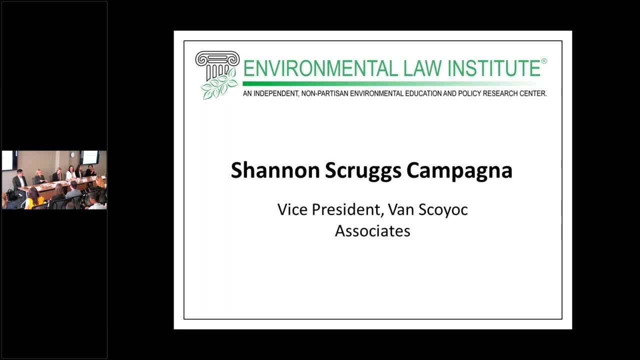 Not in my office. So there were these big things that would sign the member of Congress or other sort of influential person's name on pictures. So that was my job, So I did that and that was a great experience. And then I was able to get a job on Capitol Hill for a member of Congress from Missouri. 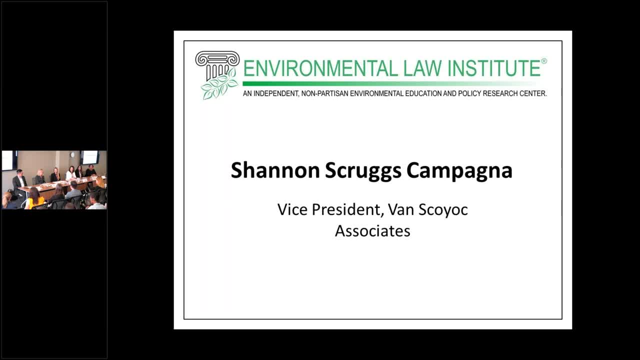 I'm from Alabama As a Republican. at the time there were only two Republicans in the Alabama delegation in 1990.. So times have changed, And so I had interned for one. My roommate worked for the other member, so I got a job with a member from Missouri. 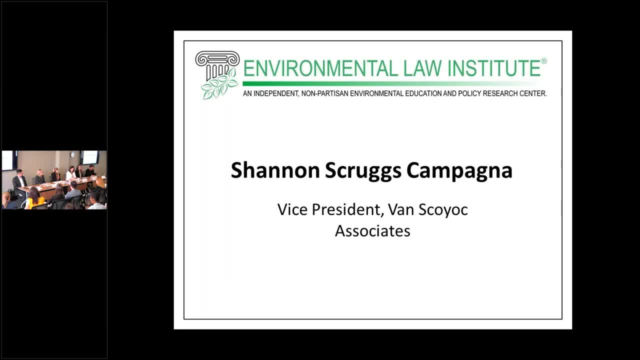 And ended up working for him for seven years. He was a great guy. He was a lot more conservative than I was And I didn't really get you know. I was sort of like a conservative Democrat from Alabama who called myself a Republican at that point. frankly, 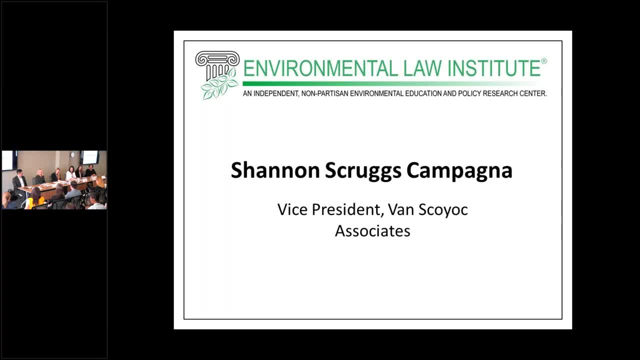 And then I got here and I met, you know, like real Republicans, I was like, oh wait. So my boss was kind of- he was, I say he was kind of Tea Party before there was such a thing. He voted no on everything. 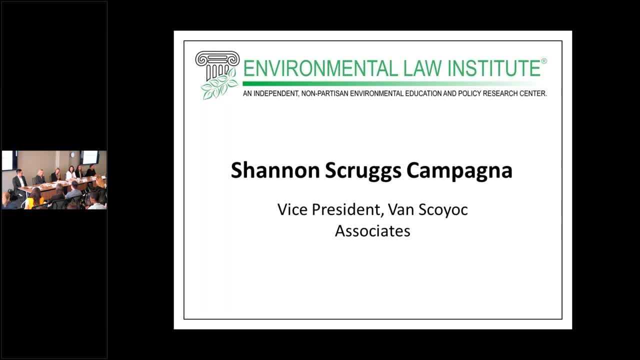 He was very. He was very pure, idealistically pure, ideologically pure, but a great guy. So I ended up working for him for seven years. He was on the Transportation and Infrastructure Committee at the time And then he got on the Ways and Means Committee while I worked there, which is an influential committee, tax writing committee and very important for Social Security, health care, taxes, trade. 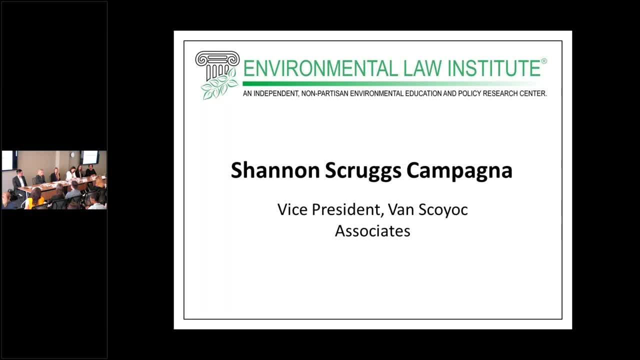 It's a great committee. But again, hearken back, Mel is very conservative And so he let me do the girl issues, which happily was welfare reform. So I got to do welfare reform in 1996, which was a big landmark piece of legislation under Speaker Gingrich. 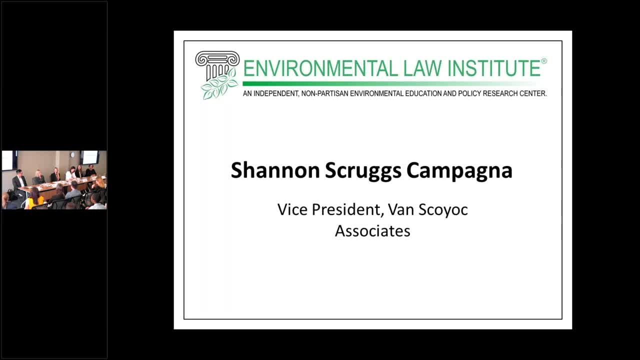 So that was a fun and kind of high profile issue I got to work on When he retired. he was a term limits advocate and actually was one of the few who left when he said he would after four terms. So after I spent seven years with him, he retired, went back to Missouri and I ended up working, went to a law firm as a non lawyer, went to Aiken Gump for about five years, which was a great experience. 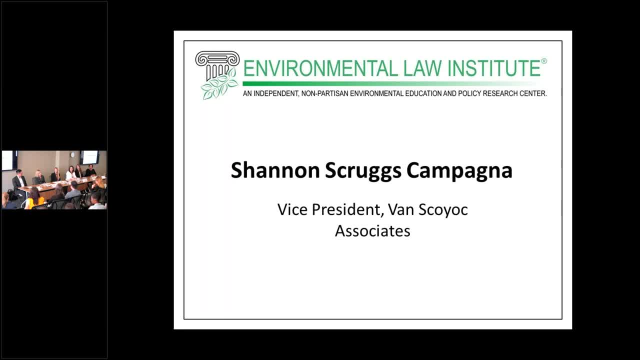 It makes me seem so old, but in so Politico Pro. you're all probably pretty familiar with Politico Pro and you get those sort of whiteboard alerts and this is happening and that's happening. So at that time there was no, There was an Internet, but it was just in, you know, wherever it was in a big room. it was not widely used. 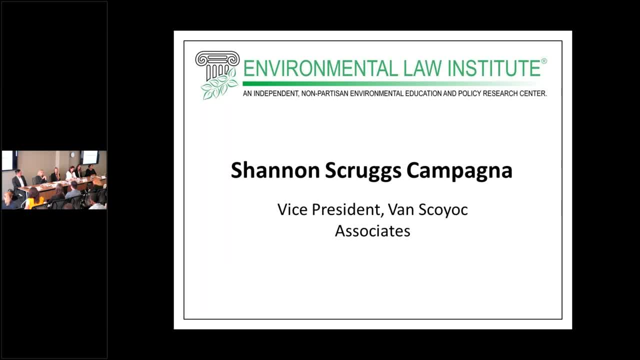 So we, there were a group of us who were not actually lobbyists, but we were sort of like reporters for our firm and we would go to the hearings And then, if something really big happened, we would run out in the hallway And if you've ever been in Longworth, there is this, here's this row of elevators, or elevators, a row of phone booths. 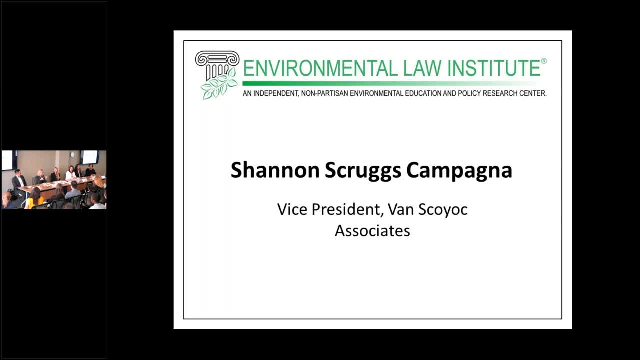 Are there Used to be in a part of the hallway called Gucci Gulch where all the lobbyists would hang out. There's a really good book from nineteen. eighty six called about that And we would run out and call our colleagues at the firm and tell them that they needed to call our client and say that something was happening on our issue. 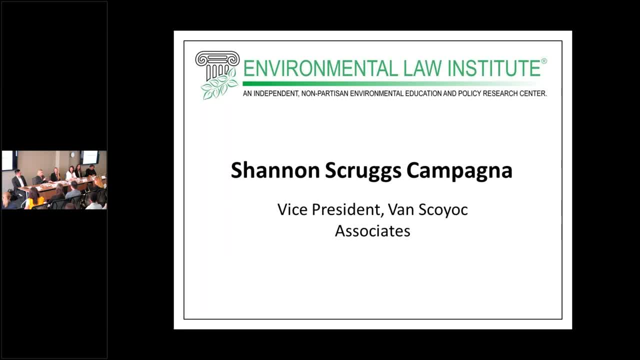 And you had to actually have a friend who could give you a hard copy of the amendment or the chairman's mark so you could take it to your office and copy it at two o'clock in the morning and then take a And have it to your identity to give it to you. 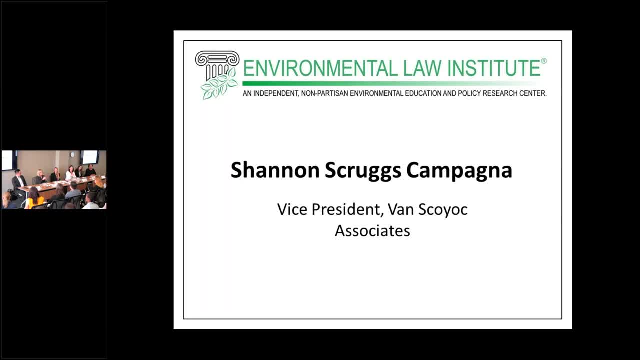 So you guys have it really easy. So you know, PDF Documents were not a thing, So, but it was great training ground because you have to be first with the information, which is harder to do now because it's a matter of minutes rather than hours that you, if you're plugged into your network, you get information earlier. 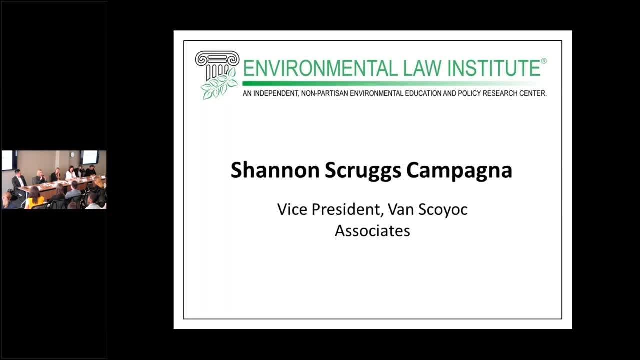 And then it was when, with the advent of PDF Documents, we all in the kind of lobbyists and policy world figured out that we had to add value. It's not just having information first, but the analysis and adding value and context. 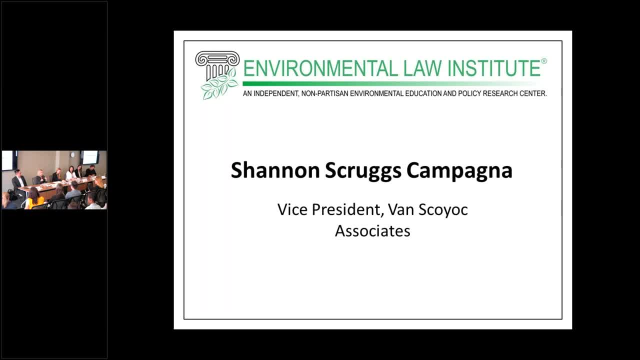 to the information is what's important, not just being the first to hand them a piece of paper. So I went from there. That was a great experience. Those of us who did what we did at our firm at that time did not actually lobby. 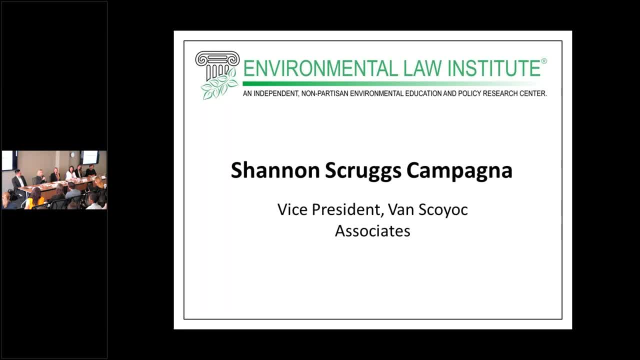 So we were not lobbyists per se, We were not registered lobbyists, But it was great training for that. I did that for a number of years and loved it. But I thought, you know, I want to kind of take an issue from inception to the advocacy. 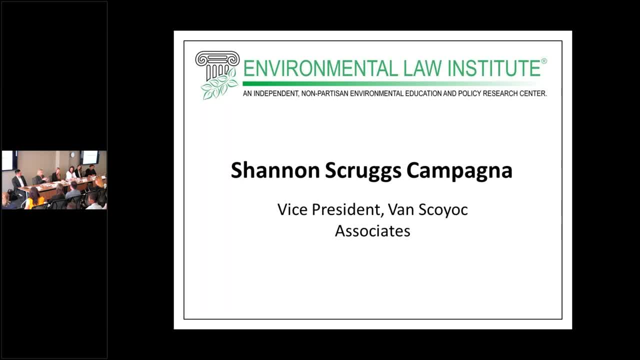 part. I don't want to just sort of talk to the client and tell them what they should do. I actually want to do that work for them as well. So, Akin Gump now I think, lets non-lawyers lobby. but they did not at the time. 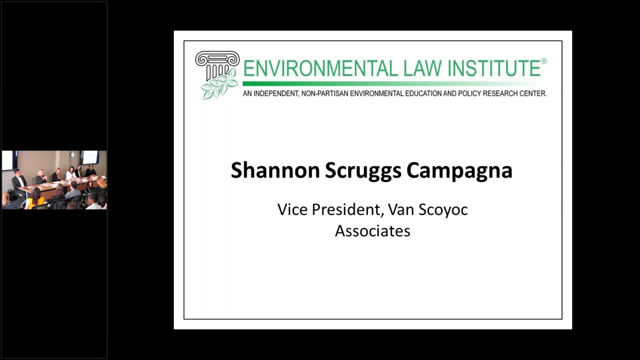 So I decided to go elsewhere And I went to a trade association that represents the beer wholesaling industry. And yes, the beer industry is super fun And you know people always say: why did you ever leave? So most of the people who work there when I was there are still there. 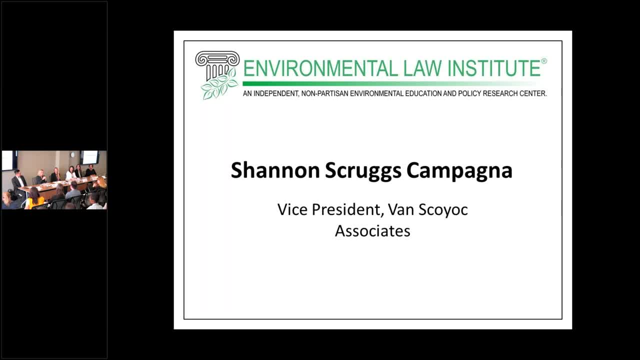 It was a great job. Again. that was a great training ground because you get to meet lots of members of Congress. They have a large political action committee, So you know you can make lots of friends. Frankly, we didn't have to ask very much of members at that point. 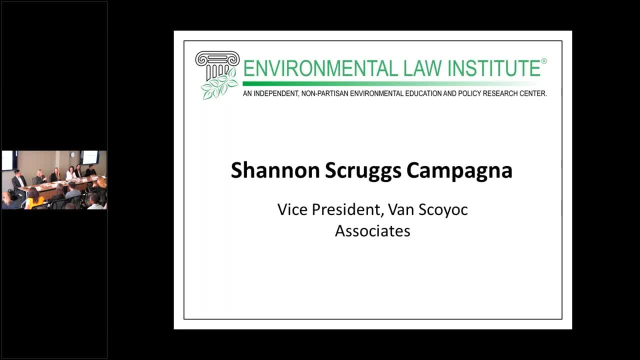 There was not a lot of. they were like you know. there was tax legislation impacting beer wholesalers, Um, but for them, Most part, it was just sort of a very a great opportunity to build relationships on the hill, get to know lots of members. 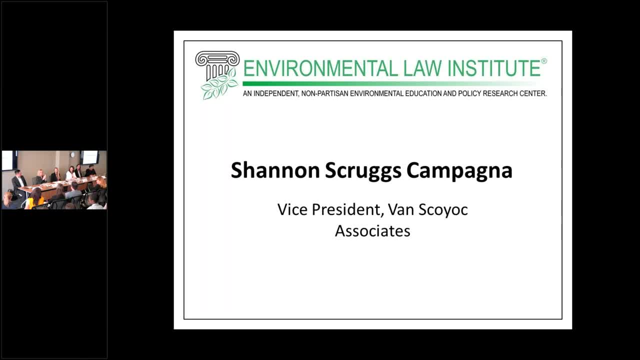 And you didn't have to ask a lot of really hard asks of of your members of Congress for your, for your employer. I went from there to the Retail Industry Leaders Association, which was great fun That was. that's all the sort of large format retailers like Target, Wal-Mart, Home Depot. 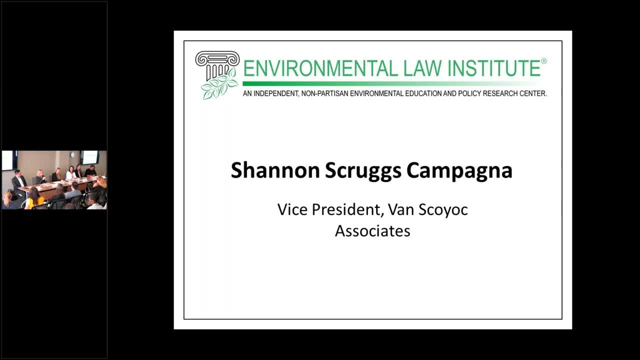 those guys And I enjoyed that a lot. You know I've been very fortunate to kind of work for a lot of brands and sort of being able to walk into a room and say I work for, you know, beer, or I work for who doesn't love. 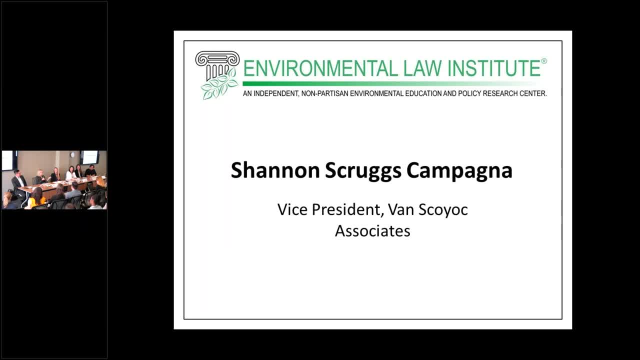 that or I work for, you know, large format retail. So people I was, I've been fortunate in many instances to work for kind of iconic brands that people really understood and could relate to and, for the most part, had good feelings about. Um I went from 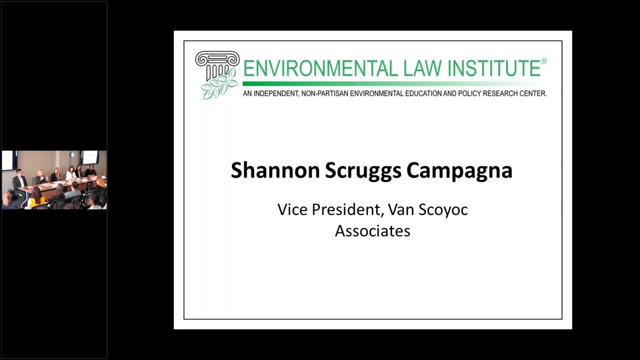 There to Safeway stores And again, that was great because even members of Congress who don't have them in their hometowns shop at a Safeway here locally and hopefully had good experiences And if they don't, they would let us know about it and how long the line was or they were. 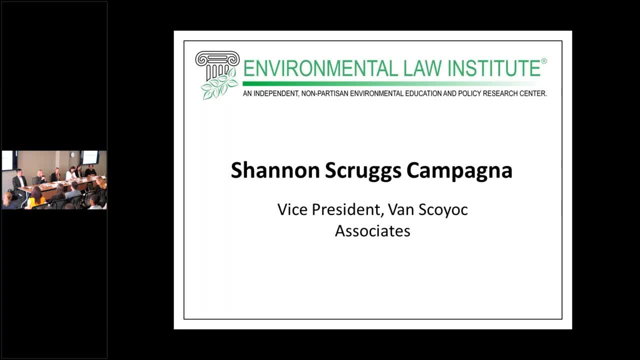 out of their favorite product or whatever. And that was a terrific opportunity to do corporate lobbying, because I had done trade association but I'd sort of started with a law firm to trade associations and corporate. they're based in California so I would go out from time to time but I did not really. 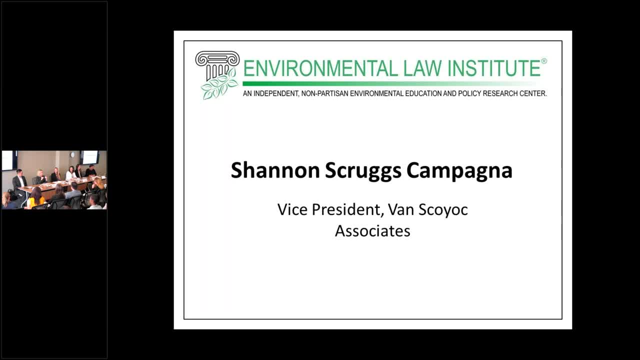 understand being integrated into a corporate culture until I went to a large global family owned food company where they are located here in McLean, And so I really was able to totally integrate into a corporate environment And really understand how to work within that framework, when you know, it's not just about. 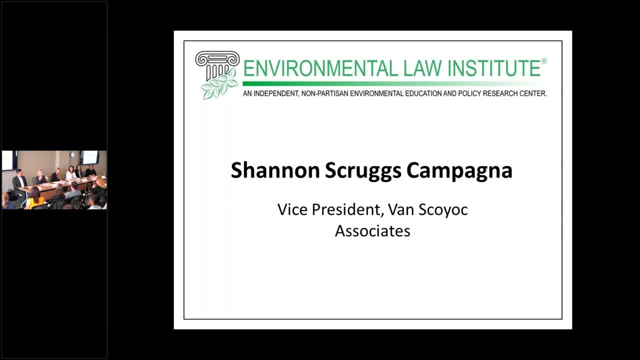 the US market and lobbying the House and Senate, but we're looking at legislative and regulatory bodies all over the world And that was kind of humbling to realize that the US is one, just you know one- market in the world and not everything revolves around that place over there which is, which is. 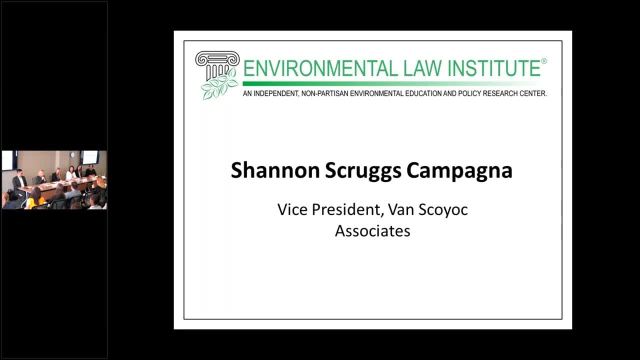 a good, a good thing to realize. That was a great experience. But then it was kind of time to go back to my roots and I went back to a law firm- a different firm this time and as a non-lawyer lobbyist, and we were called senior policy. 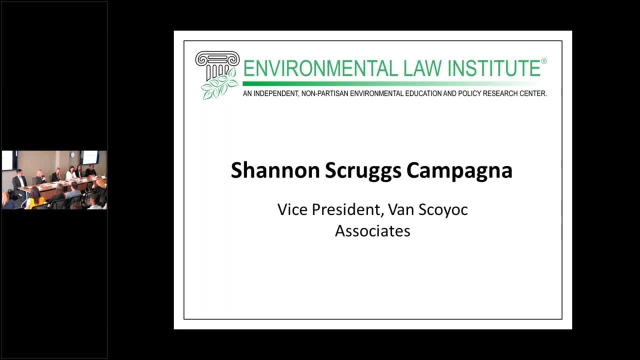 advisors at the firm Alston and Byrd, which is a terrific experience that I enjoyed thoroughly. I got to develop my own portfolio and book of business there, which was not as difficult as I thought it would be. It's still scary. 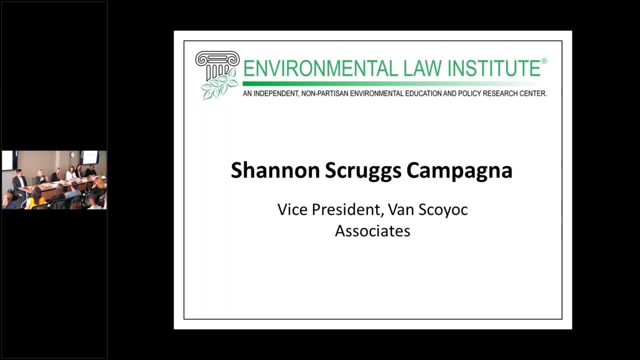 When I think about the fact that I'm a law firm, I think about the fact that you know I'm solely responsible for identifying and bringing in business and keeping those folks happy. but you know, so far so good. And at the firm I was able to also work on other clients of the firm. 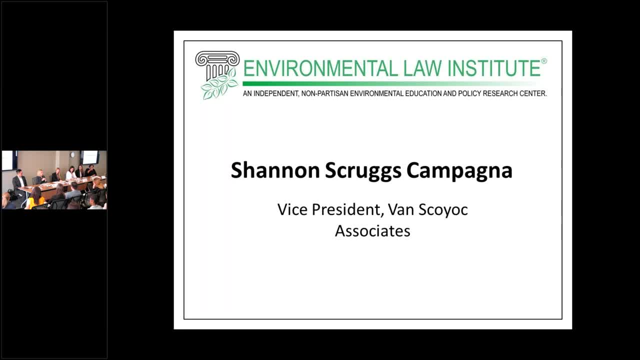 So we would get these sort of over the transom emergency calls because a client of the firm suddenly has a legislative issue that they didn't know they had, or they've identified it or for whatever reason. they're just figuring out that they've got an issue and they're here. 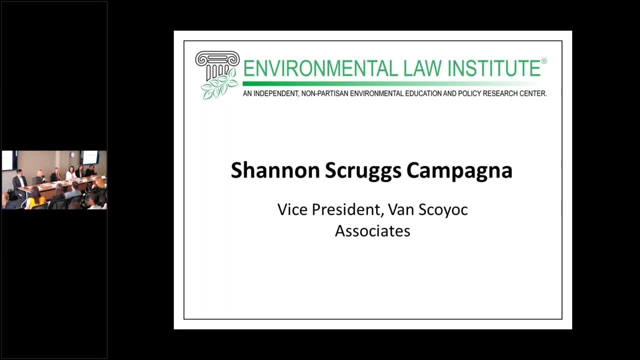 Yeah, So you can't just have the workers on fire and you have to help them fix it. and working with the attorneys at the firm We were talking earlier, especially at a law firm, it's kind of nice not to be burdened with the law degree, because then you can just sort of say and do things that you know. 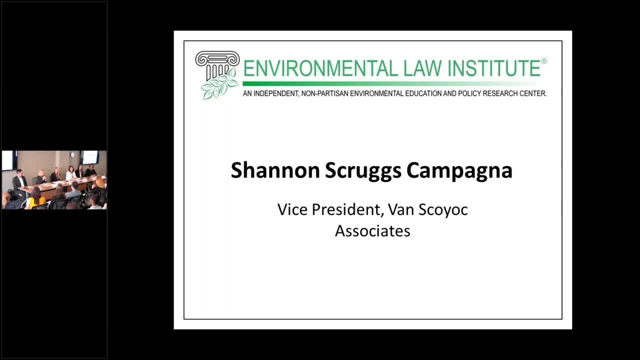 lawyers would not do So, that's. I've found that I have at some points wished I had a law degree and other times been grateful that I didn't, because I don't have to. I'm not burdened by that. 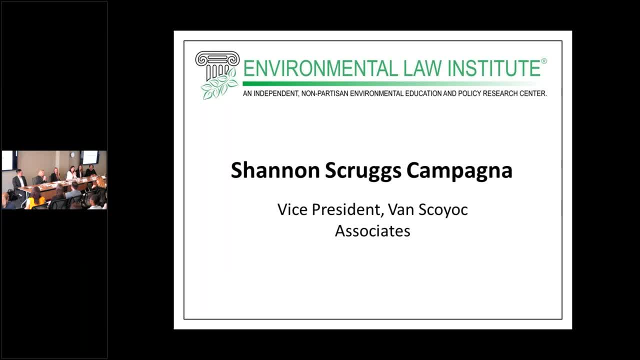 So, yeah, I'm a lawyer, I'm a lawyer, I've always been a lawyer. I've had a lot of fun with my clients. I've really enjoyed my time at Austin a lot. I was recruited away by a non law firm lobbying firm just at the beginning of the year and 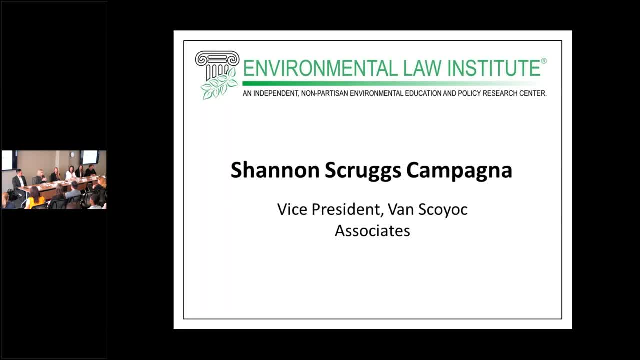 whenever they're in February. So I was fortunate to be able to bring my clients with me and that's been a great, a great fit. I've had additional clients there. It is nice not to have to bill hours. I will say that's something that I do not miss. 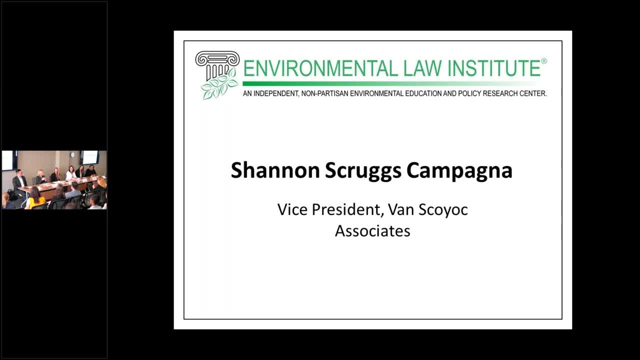 I didn't mind it at the time, but then sort of not doing it for a while, it for a while has been really, really great. So I think you know my sort of advice is: it's all a lot of these opportunities have just sort of unfolded and I, when I went to undergraduate, 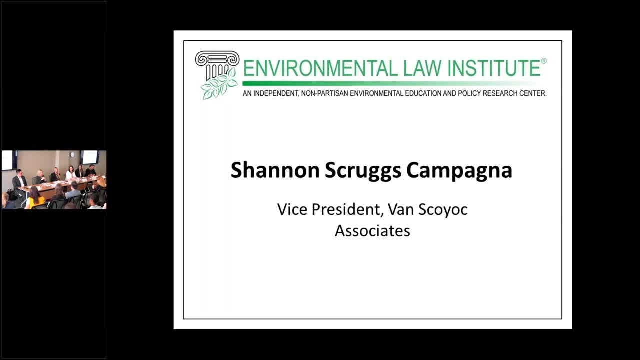 I really thought I wanted to work in international relations. The Berlin Wall fell right as I was graduating, so kind of everything I knew was obsolete and really belonged more in a history book than in a sort of current policy, and everything was new and exciting, but also 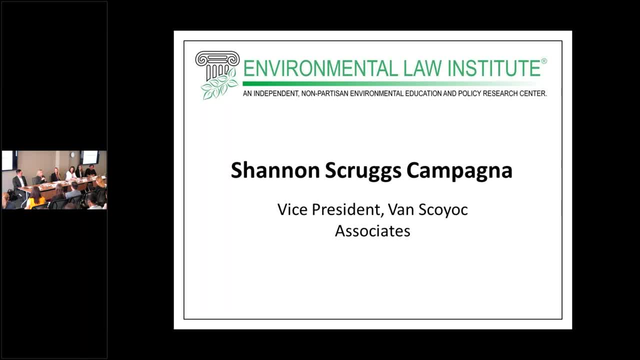 different and uncertain. so when I started working on the hill it was- it was really more in the vein of sort of domestic tax and those kinds of policy issues, and that's okay. I mean I, you know, I enjoy opportunities to work in the areas that I thought I would work in and 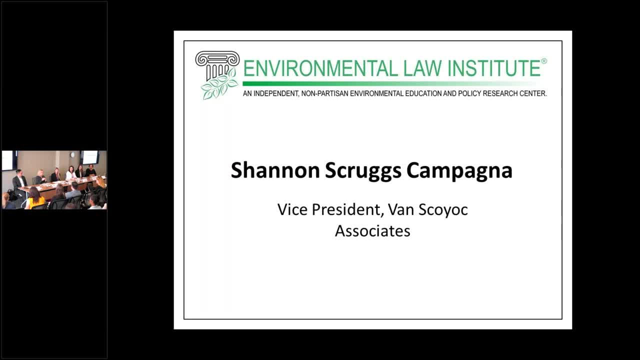 initially, I've had the opportunity to do, you know, global travel with one of my employers and really get an insight into some additional ways of thinking about business and culture and things like that, and that I'm really grateful for all those opportunities. but you know, had I gone down, 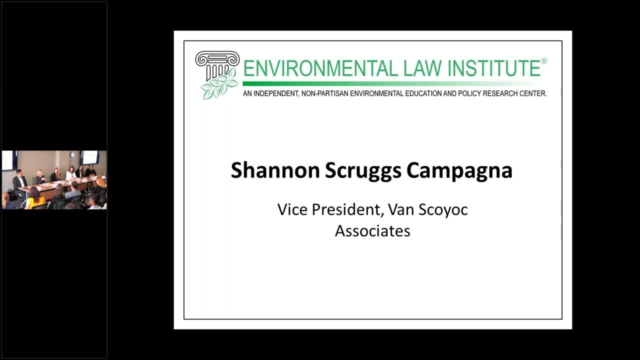 the path I thought I would have, I would likely not have gotten to do that. So you know, I think a lot of younger people are so driven and you know we've had parents have kind of ruined you all to some extent because we're we sort of push people. I'm a mom of a 20 and 17 year old but, and I think that's- 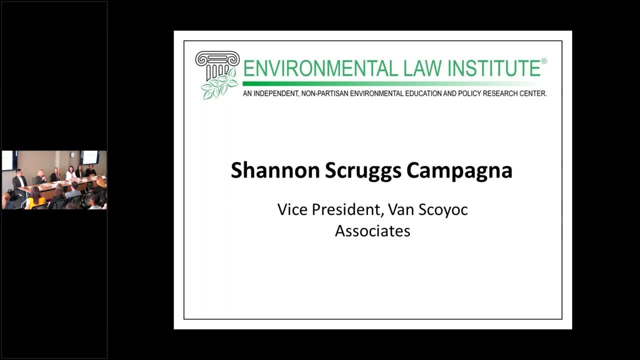 great. but I think there also is a lot of benefit to just sort of letting things unfold and taking opportunities and saying yes as often as you can, even if it seems like something that's not quite what you thought it would be. but you know, you can always change your mind and do something. 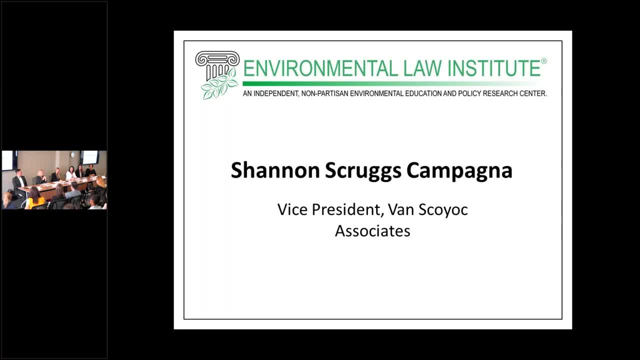 different, but my career has been one born of a lot of luck, I think, and some you know what I make up. what I lack in education, I think I make up for in tenacity and scrappiness, and just you know, I've been around a long time so, but I commend you all for 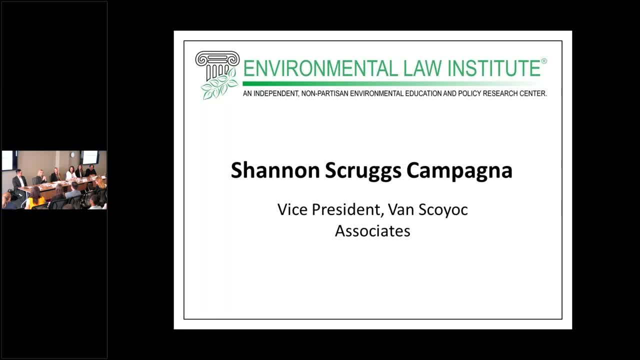 for being here and look forward to questions you might have and any additional insights I can add. Thank you so much, Shannon Kathleen, we'll turn things over to you. Thanks, well, as the other non-lawyer in the room, possibly, I'm really glad we're taking over ELI. you know law and policy are. 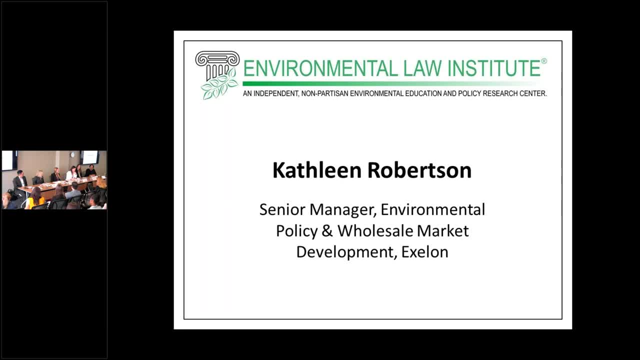 so much bigger than just legal profession. I'm very excited. everyone else is noticing that. So first of all, before I get started, what is Exelon besides a really hard company to spell, so kudos to Caitlin who has gotten it right. every time that never happens. we're a large publicly 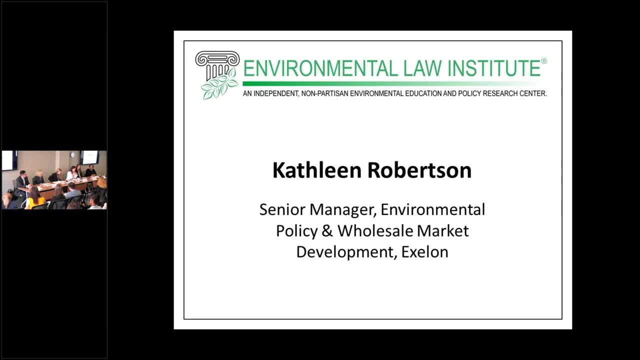 held energy company, so we have a couple different wings. so we have six electric and gas utilities, including Pepco, which is providing the electricity right here in this room right now. please don't go out- a large generation fleet. we're actually the largest clean energy generator in the in the 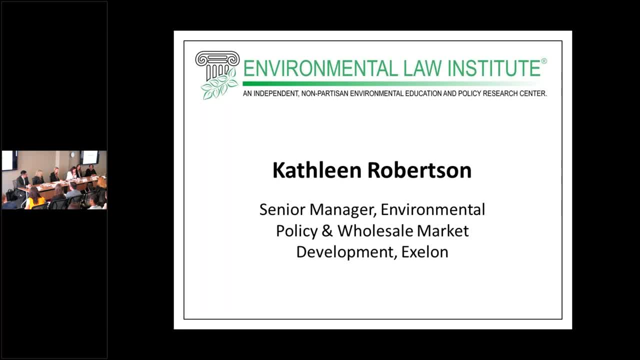 country we make more than twice as many clean electrons as everyone else as well, as we also have a large commercial and an industrial that does energy efficiency, remove some, you know, on-site renewables and some electrification solutions. so we're basically an energy monstrosity. so that's just the overview of where I'm coming. 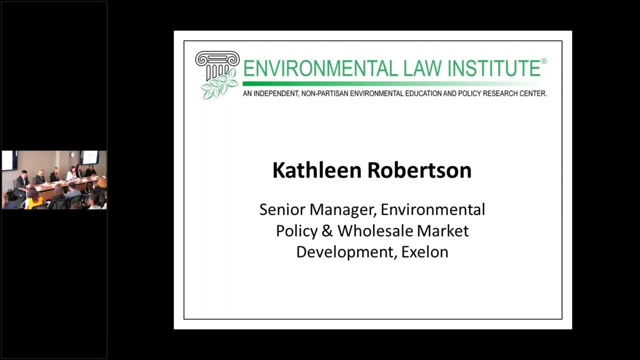 from currently, So I think that hits on. I think the theme that we're going to have throughout this panel is my TLDR for today, is their environmental careers everywhere doing everything. so just don't feel like. I think there used to be this idea that, if you wanted, 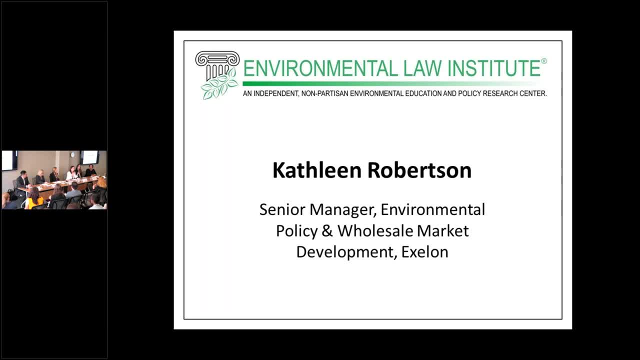 that you were interested in the environment, you had to either be a scientist or an advocate, and that's where it stopped and it got siloed like that, and I think that that's well a shame, because the environment should be woven through everything, but also it really 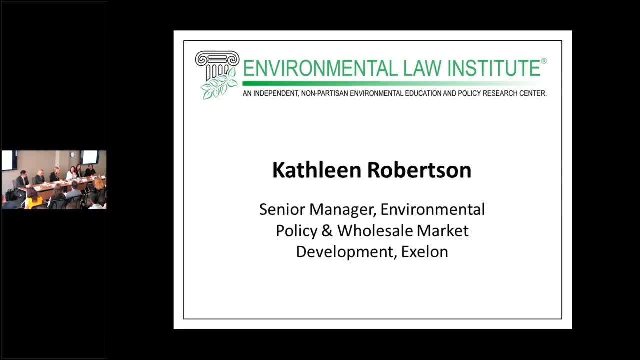 does kind of pigeonhole you like. you know Toby's thought, you know if you like science, and this is what you should do. so I think that that's. I am really excited to see how broad that is becoming and I think this panel has really gotten to that point. myself, I went, I went to college and I got. 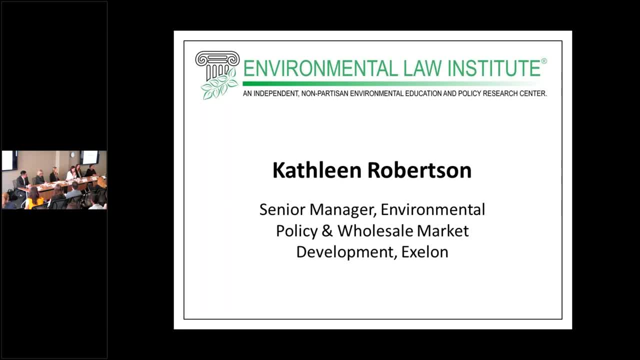 a degree in urban and environmental planning, and you guys are very, very young, but I graduated about six months after September 11th, so I went to grad school, where I then got a master's in environmental science and policy, and I think that that is going to be a theme through my experiences: the fact that both of my degrees have an and in 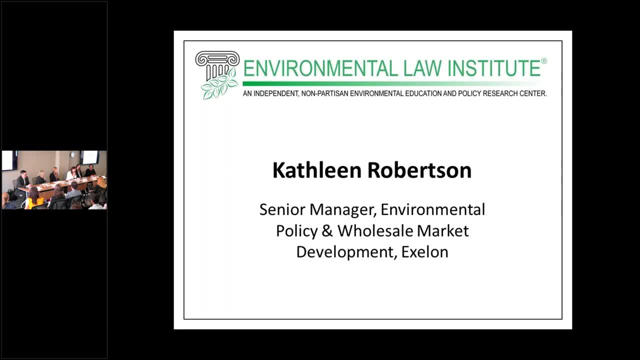 them, tells you. I had real trouble picking a lane, and so it was initially weird to kind of straddle the science and policy world for so long, but it really gave me the fluency to comfortably move between silos, as this energy was going to be. 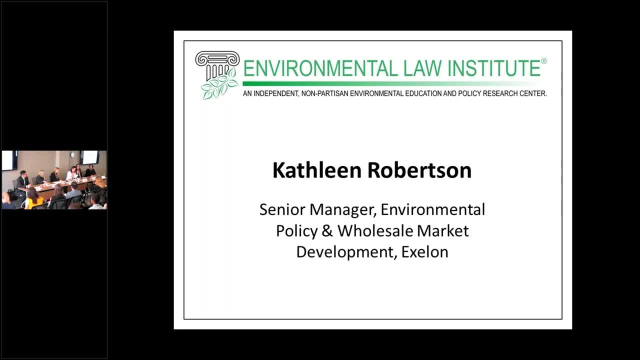 I think that I think that's one of the ways I've been able to be a part of the community, and not just as a part of the community, but as a part of the community as a whole and as a part of the world in particular, got a lot more, you know, integrated and, as things kept changing, I was used. 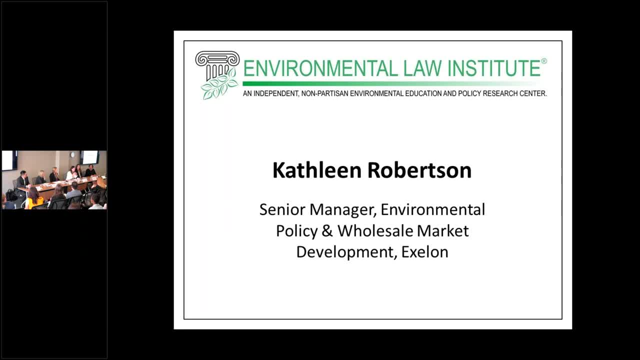 to being kind of the odd girl out in a conversation, either knowing a lot more environment than the energy people or knowing a lot more energy than the environment people. I got comfortable in that space really early. so as these things become more integrated, I think that gave me an advantage of you. 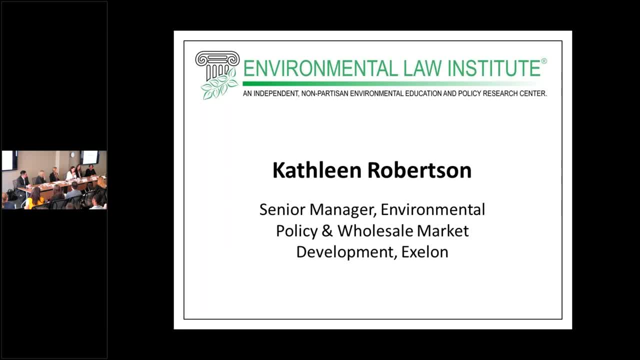 know, not picking a lane once everything got muddled of, gets to the you know kind of role of dumb luck. but um, my first job out of col or out of grad school, um, after all my ang degrees, um, i was working for an environmental consulting firm. um, i'm sure. 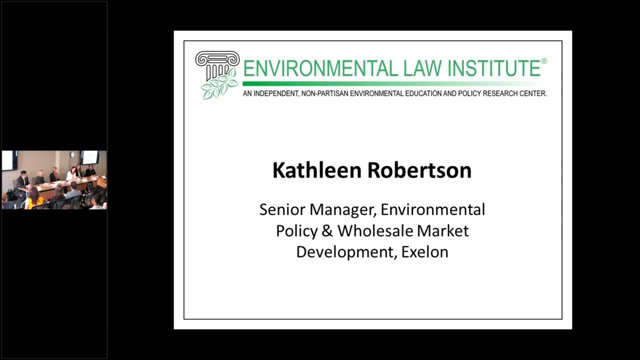 you work with those a lot. um, writing environmental impact reports was just super boring, but we were working for a lot. just happenstance it was. i still thought i wanted to be an essentially an environmental policy, environmental science person. um, but we were working for a lot of energy. 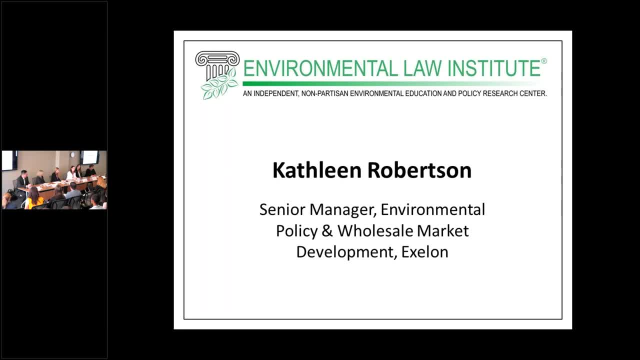 companies, thank goodness. um, and after about two years, my boss took me aside and was like: you are the only person that has ever read the energy documents that come in this door. you know, maybe just think about that as you move forward in your career, um, so i think that is one one thing to keep an eye out is like: what do you like to do that? nobody. 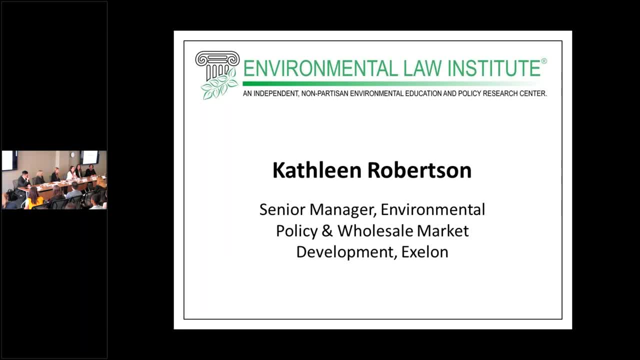 else does and bring your environmental, bring your environment sensibility to that. um, i took a few- there are a few missteps in between there- um, until i really thought about what she had said, of i really that there was just something about energy and everything that was very. 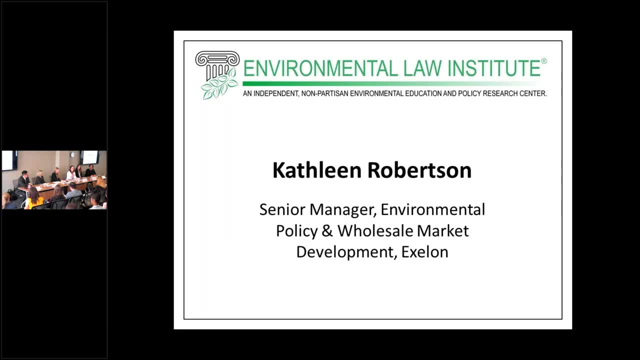 exciting in the middle. you know, middle 2000s, post enron- like, oh, climate is a real thing. what is the biggest contributor? energy is huge. energy is reforming. energy is the best, the most important thing you can do to actually fight climate change. um, so, bringing that excite sense. 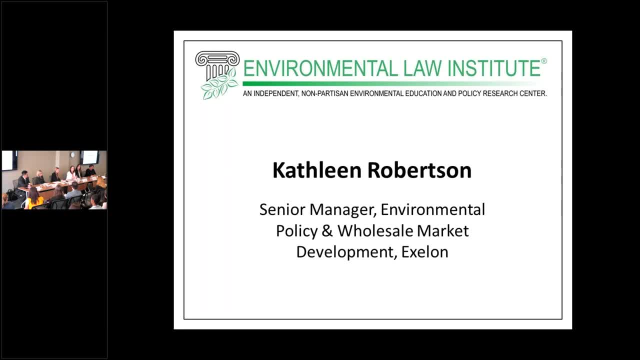 of excitement and sense of to, to an taking my interest in energy company but bringing in a little bit more of an environment sensibility to it, of knowing that you know i could do something for the climate. that wasn't just working at sierra club- not that those people are wonderful, but i 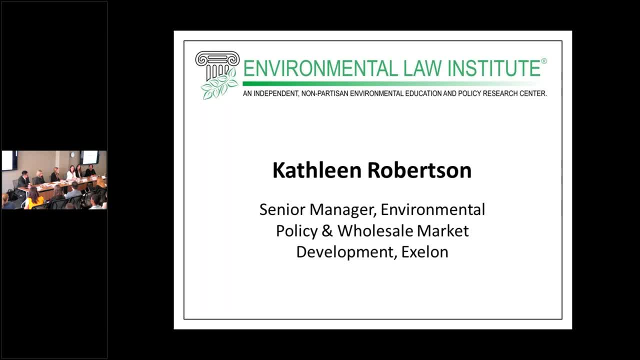 think it's awfully limiting, when you start thinking about it, of you have to work for an environmental group or an environmental science organization in order to do this kind of work. um, so then i was very lucky and landed a gig with um, an environmental- essentially environmental- policy. 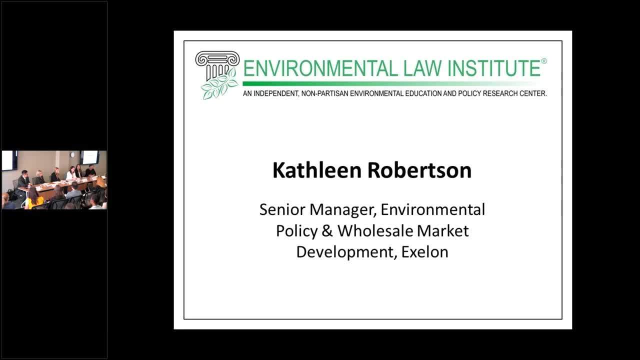 and energy policy consulting firm and i was very lucky to be part of the environmental겠�ery group. my background equity sector was in energy industry and it was a great experience. it was great experience and i got to work with the industry. it was a great experience and then i ended up. 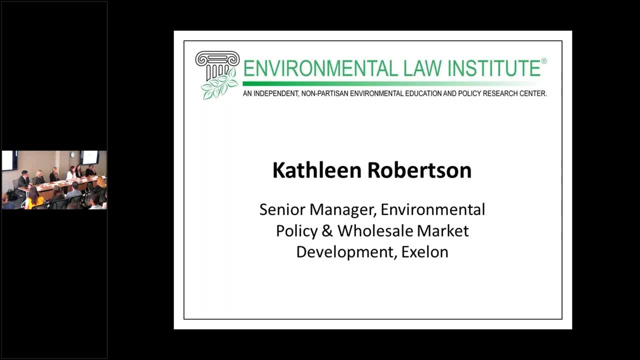 working for the dc um, the townhouse group, and then i started working with the direct association, who's a fantastic partner, and so i'm going to talk a little bit bit about the project and the project itself. i talked about it earlier, and so i'm going to talk a little bit. 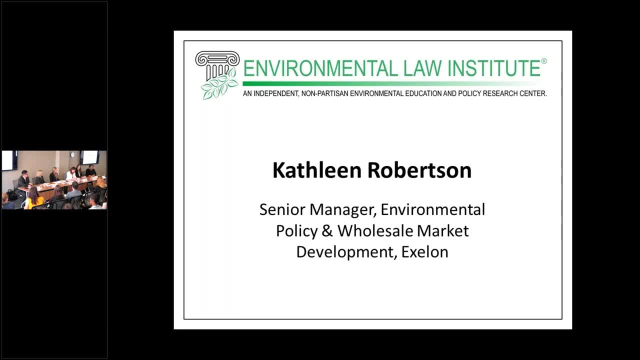 bit about the project and the project itself and i also have a very good relationship with. So it's not a traditional environmental career like I think I would have thought about it at your age, but it is. I think one of the more environmentally minded things I could do is help reform energy. 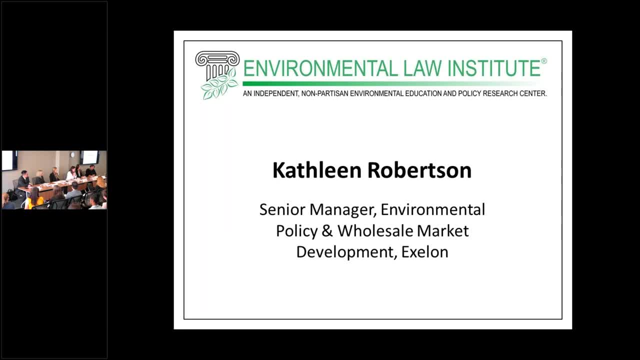 So what do I actually do at Exelon? It's the world's longest title And it's either exactly that or it's incredibly vague. But essentially my job is to change the rules. So sometimes not having a law degree is helpful, because I don't always know what the rules are. to begin with, to seek value in environmental performance. 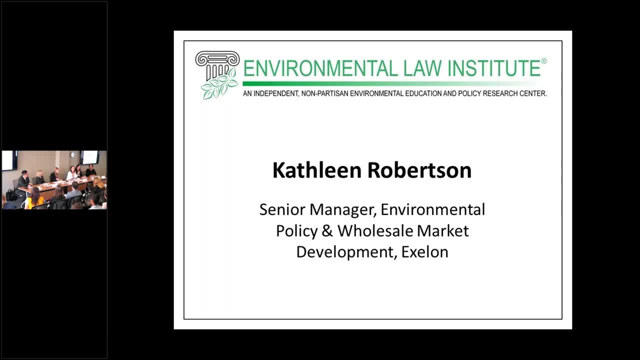 So how do I help change the rules so companies like Exelon and, you know, our other energy brethren, so that the incentives are lined up with where we want the world to go? You know, do you incentivize dirtier technologies or do you incentivize cleaner technologies? 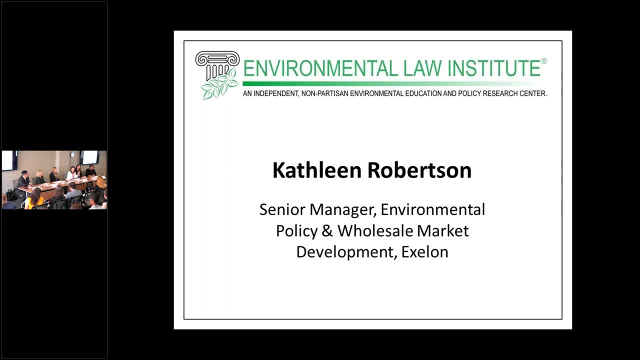 That's all policy Most businesses understand Are in it for the money and for the shareholders, frankly. So how do you change the rules so that that aligns with where we want policy to go? And that's essentially my job. It's a lot of skills that I'm sure you all have. 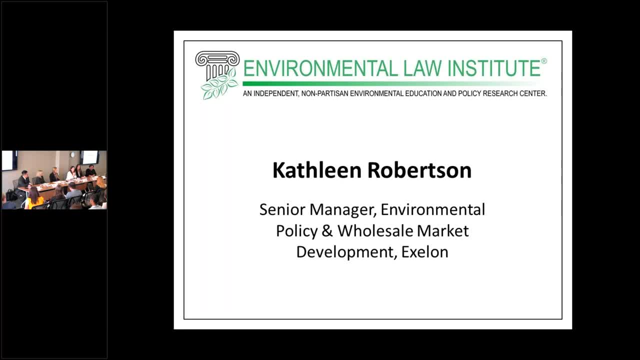 It's writing, it's presentations, it's comment letters and it's also just straight invention. It's, you know, inventing. you know what, what, what sort of incentives would cause the outcome that we want, or you know as rules or laws are proposed of, you know bringing to the table. 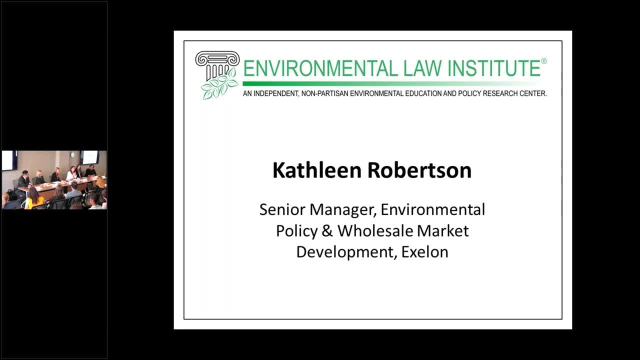 What, how, how, of course, How would corporations react to that? I have a lot of friends and environmental groups and other kind of more traditional environmental policy world And I think one of the things that I bring that's rather invaluable in some of those conversations is explaining exactly how the energy and electricity markets do work and how they will immediately pull apart that really well intended environmental rules. 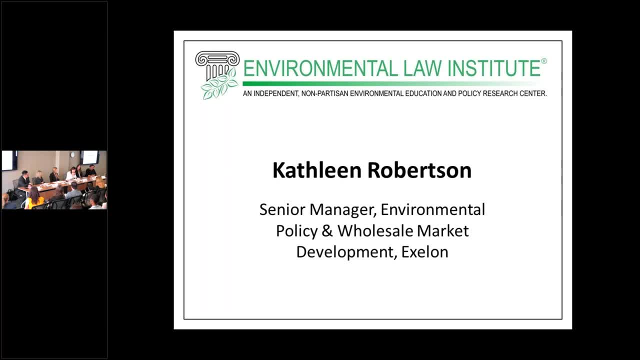 And it won't have the outcome that they expect. So I think I will shorten it there because I know we have a time crunch on some things. One thing that, And then sort of There were some instructions, we wanted to identify an obstacle. that I think we will be more Q&A. but I think really important thing to think about is particularly 10, 15 years ago environment was seen as a soft skill and it wasn't as big as science or business or law. 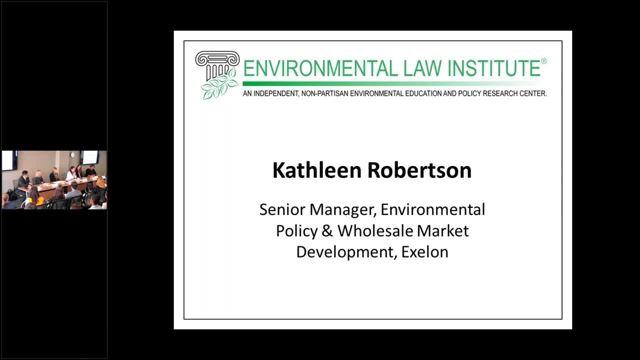 Like raw or hard stuff, but I think it's becoming more integrated in how businesses make decisions. I can't think of a Fortune 500 company that doesn't have a sustainability officer right now, But the question is, is it their actual integrated decision making? I think there's still some ways to go on thinking. 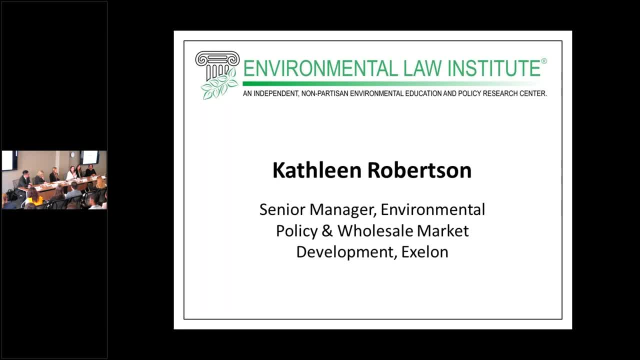 of environment as a you know, a primary factor in a merger and acquisition, not an afterthought or a oh. how extensive could that Superfund site end up being? I think that we do have some ways to go across sectors on integrating environment more holistically. 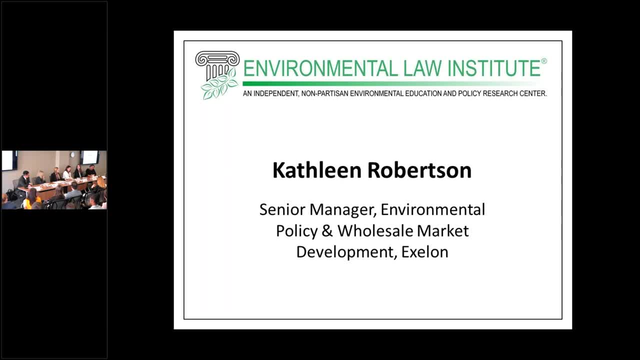 Great. Thank you so much, Kathleen. We will jump ahead to Kendra, and then it's your turn, Kathleen. Hello everybody. So, as you know, I'm Kendra Brown and I'm the Chief of Staff to Congressman GK Butterfield. I apologize, I was texting a little bit. We are voting today, so the 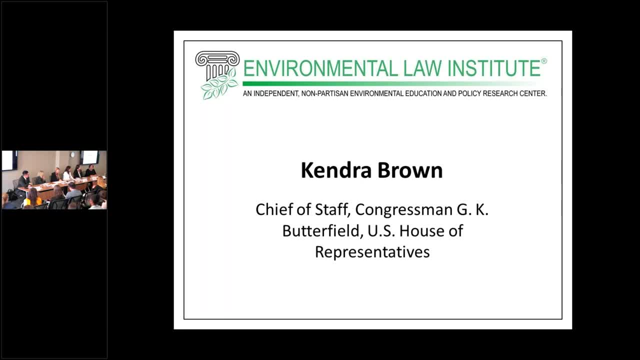 members are very active And my boss is in two hearings at the same time. right now He's on energy and commerce. So you know, just a little committee with a little bit of drama. So literally some members say that 50% of the bills that come before the House of Representatives. 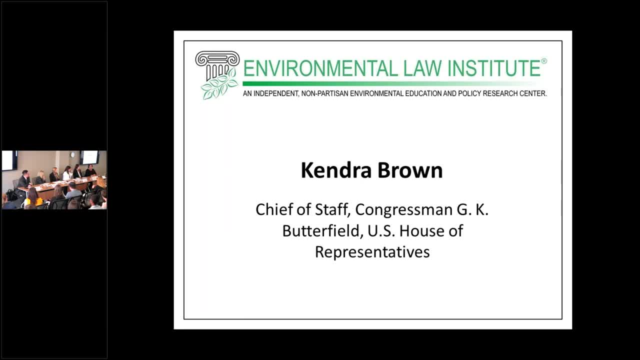 are referred to the Energy and Commerce Committee. So there's something there. There's so much there, from energy and the environment to health care, a little thing called privacy, data protection, et cetera. So just lots of things happening right now. 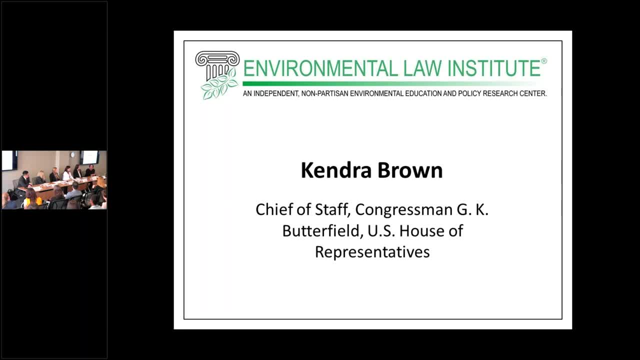 on the Hill. So I am going to be speaking with you very briefly about roles within the government and on the political side And what I did. I just kind of mapped out the committees within the House and the Senate And I'm going to give you a little bit of an overview of the roles that touch on or 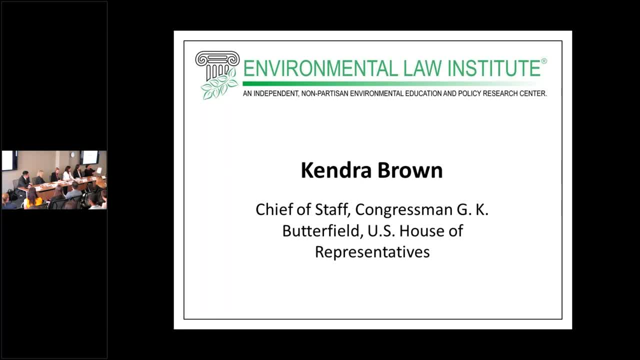 have jurisdiction of the environment, And there are more than you think. So, if you can see, this I'm trying to show on this is just the House, right? The Senate starts down here and goes over this side, And I didn't even list the Senate subcommittees. So when you 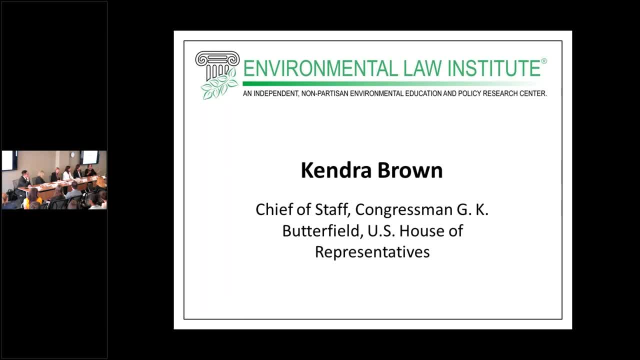 think about roles within energy or the environment. there are so many roles on the Hill that any number of you, all You know, are able to be considered for, And there are attorneys on the Hill. There are non-attorneys on the Hill, As she was saying earlier. I mean, just you name it, and 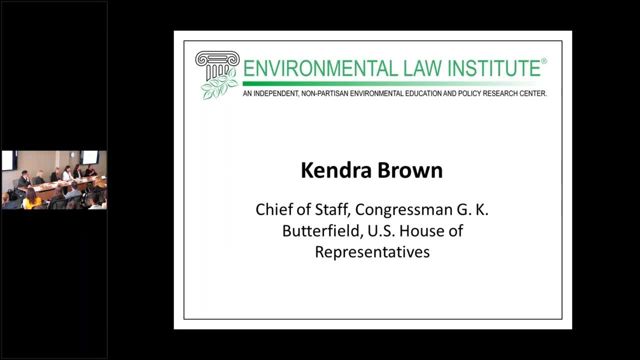 they are there. So the congressional structure within the Senate and the House is that you have something like me. I'm the chief of staff, So I advise the member literally on everything. So most chiefs of staff serve as the chief advisor to their member. 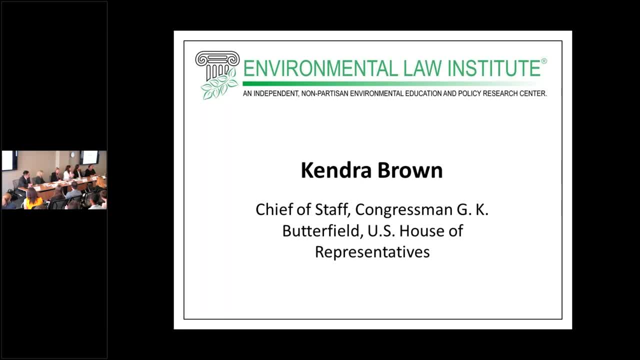 Sometimes that role is held by the LD, where they act as the chief advisor, But oftentimes it is the chief of staff. under the chief staff, You'll have either a deputy chief of staff or a legislative director, And then from there you have legislative assistance policy advisers. 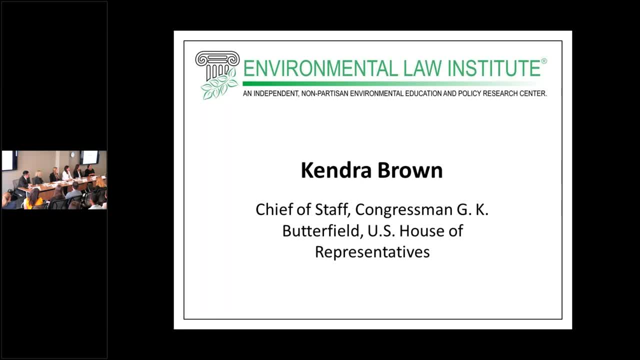 senior policy advisers, counsel, legislative assistants, legislative correspondents, staff assistants, communications directors and schedulers, So So the federal office has some type of blend of those roles in the Senate and on the House side. Within the House you, and in the Senate there are committees Right, So every member sits. 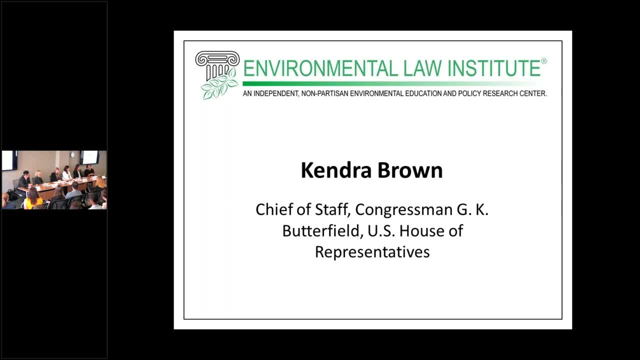 on at least one committee If it's an exclusive committee where there is jurisdiction, such as the Energy and Commerce Committee. So my boss only he sat on energy and commerce for a long time, But then he's also now in house admin, And so the committees that I've listed that touch on the environment in some way shape. 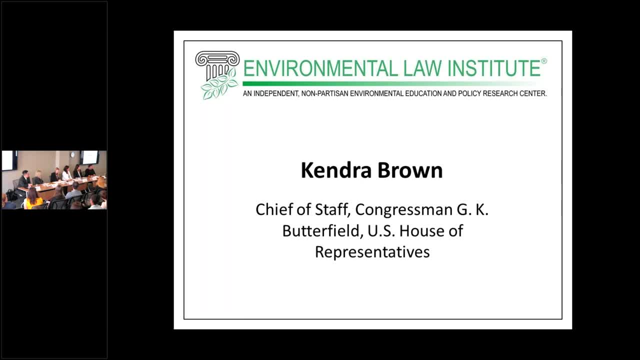 or form, are the Committee on Natural Resources, Agriculture, Appropriations, Energy and Commerce, Oversight and Reform, Science, Race and Technology, Transportation and Infrastructure and the Select Committee on the Climate Crisis. Those are just a few, And those are the full committees. 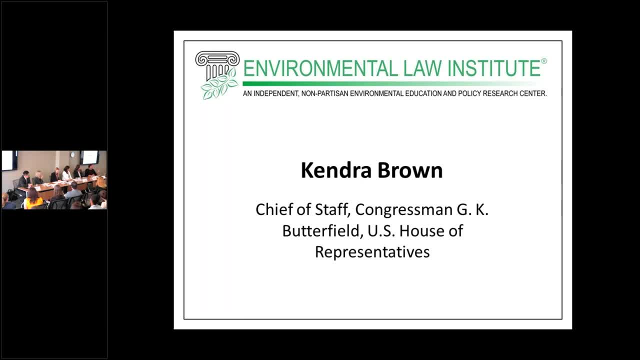 except for the select committee, Some of the underlying subcommittees. under natural resources, we have Energy and Mineral Resources, National Parks, Forests and Public Lands, Water, Oceans and Wildlife. Under AG, you have the Biotechnology, Horticulture and Research, Livestock and Foreign. 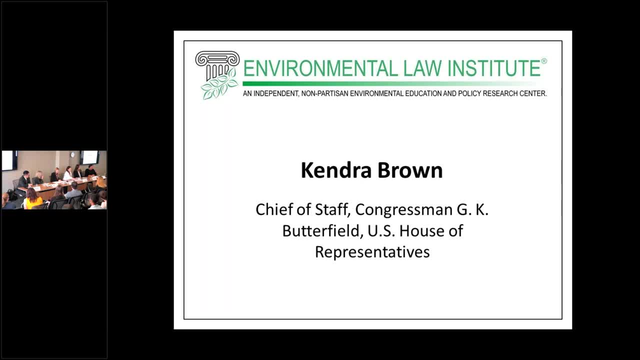 Agriculture Subcommittee on Nutrition. Under Appropriations you have the Interior, Environment and Related Agencies. That's where all the funding is Energy and Commerce. of course there's the Energy Subcommittee and the Environment and Climate Change Subcommittee. Oversight has the Subcommittee on Energy. 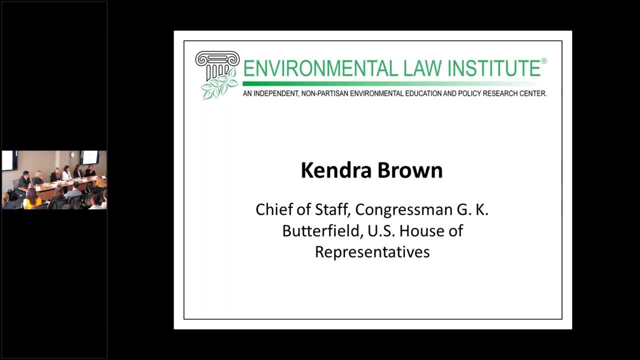 Subcommittee on the Environment Within the Senate you have Agriculture, Nutrition and Forestry Committee, Appropriations Committee, Armed Services. even touches on environment, Commerce, Science and Transportation, Energy and Natural Resources, Environment and Public Works, Finance and Foreign Relations- also Foreign Affairs on the House side. So I say: 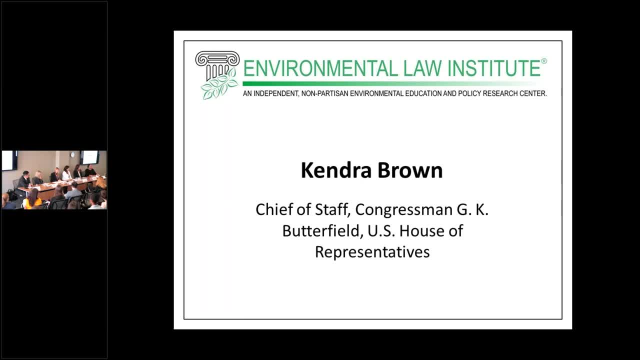 all that to say there are so many opportunities for individuals within our government structure, and that's not even counting the agencies which I know are not right now. So that's the subcommittee which i know rachel will talk about um, but within congress, um within the committees also. so i've 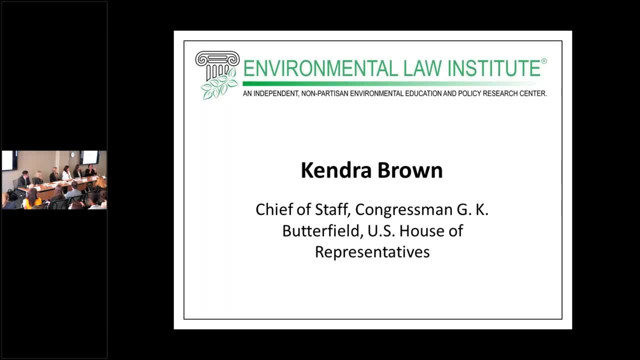 spoken about the house and senate. uh, personal offices. but within each committee there is a staff director. this is a minority and the majority. there's a staff director who is like the chief of staff for the committee, then you have a chief counsel, and so what? the chief counsel's role? 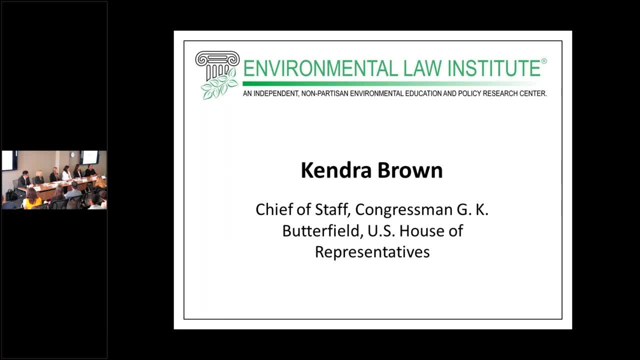 is. they are the individual who is essentially um, when there is a markup and there are questions about the bills. they are the ones who sit in front of the committee and actually ask the questions of each side so that they can flesh out a piece of legislation and mark it up. it's very fascinating. 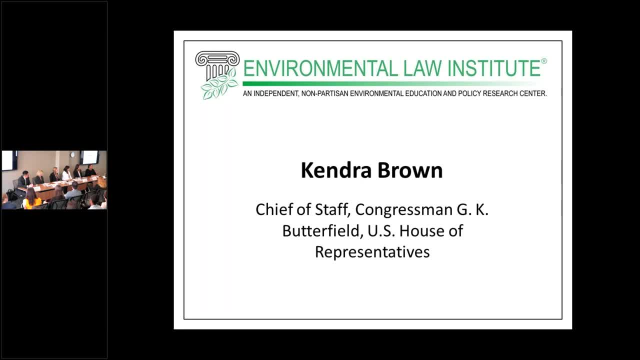 to watch. so i encourage you to watch that. um, so you have the chief councils, you have councils. you have subcommittees, staff directors, you have clerks. you have legislative officials: you have staff directors- you have staff directors, you have clerks. you have legislative assistance. so, with so many, so many different roles, you have professional staff and there are 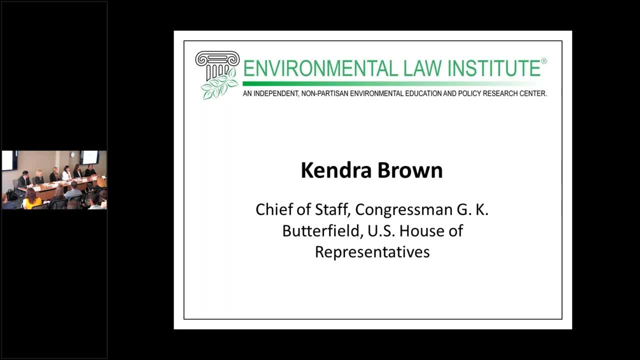 attorneys and non-attorneys, right? so the professional staff, i would say, tend to be non-attorneys. in the council roles tend to be the attorneys, so there really are roles for everyone within the committee. you really are showing an expertise in a particular area, right? so if you 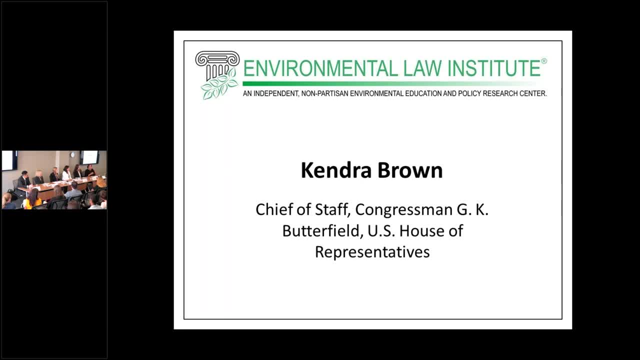 have expertise in nutrition and forestry. you're not going to be on the small business committee, you're just not. so you're going to go where your expertise leads you, and so that's just a little bit about how things operate within the personal offices, within the committees and on the senate. 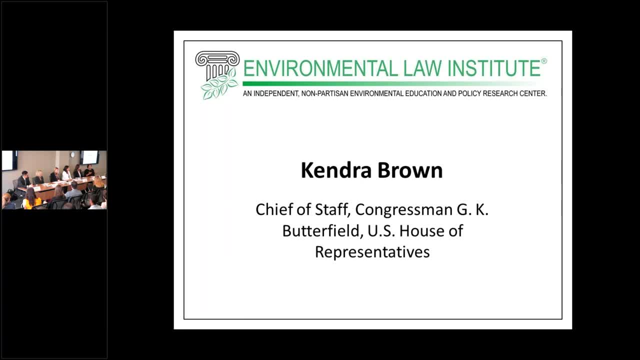 side. so a personal office will have maybe, maybe 30 people and above. on the house side a personal office has about 15, i would say max, maybe 15 to 18, you know, like individuals. and then the committee staff can range um from 30 people and up to even 15 and up. it just really depends on the size of the 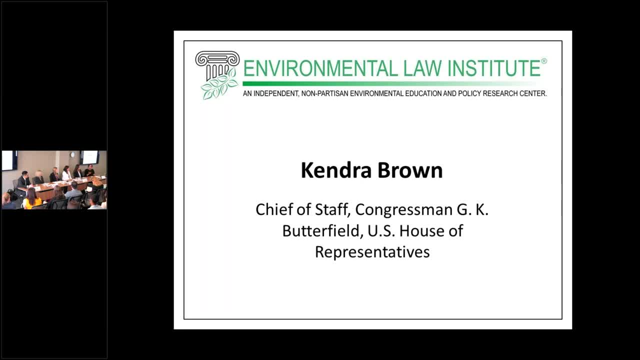 committee. so there are just so many opportunities for individuals to really work on issues that they are passionate um. as far as where the vacancies are listed, you know where they are um you know you're always welcome to reach out to each office to see um you know if, if, if they're hiring. but on 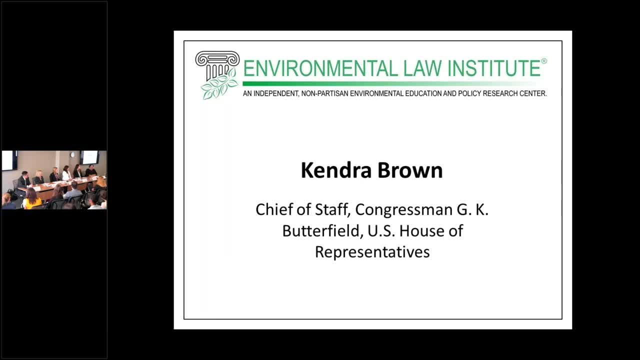 the house side there's the house vacancy office and that is um. so they have a listing that you have to subscribe to and all those vacancies come to you every week. on the city side, under visitors page, there's an ongoing listing that is updated, um, i think, every tuesday. it's once a week. 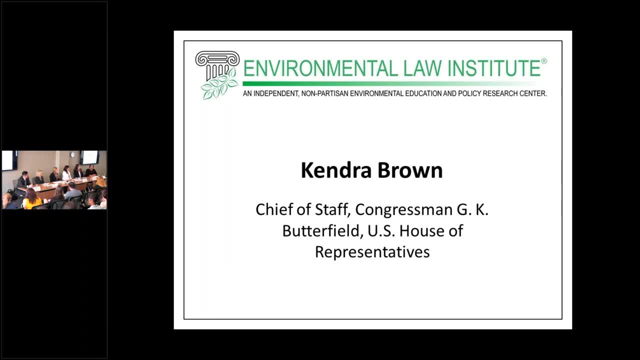 where they list all of the current um openings and they have the senate placement office um on the senate side and then the house side and the senate side both have diversity um but offices. so senator schumer has a diversity initiative that he has started. there's also, i believe, a 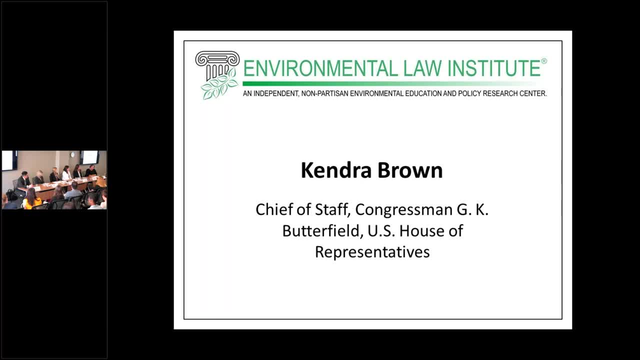 diversity initiative. now that, um, the republican offices have started um, and then on the house side, there is a diversity officer, kimba um, she's wonderful. she is housed within the house admin committee, but she is employed by speaker pelosi, so there are just lots of different. 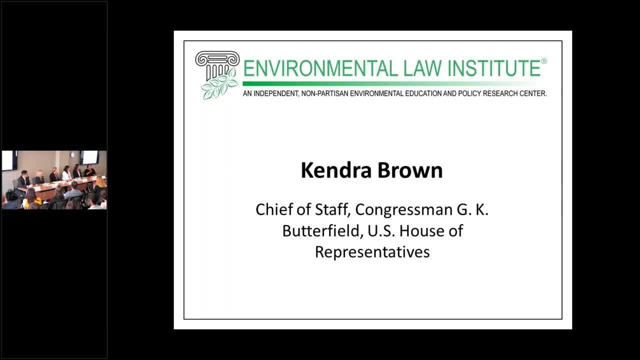 things happening to diversify the environmental world on this side. so i speak about- i speak oftentimes about diversifying the field of environmental law, but also now we are trying to ensure that we are diversifying um capitol hill staff as well. but i think that, as far as you, 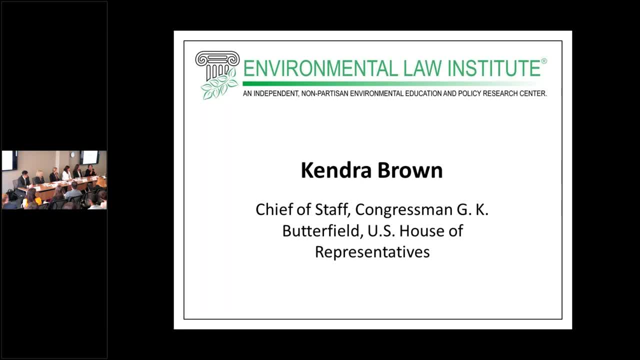 all are concerned within your areas of expertise, as far as you know, the environment and energy space- there are opportunities for everyone and i've shared the structure with you just to show the amount of opportunities that do exist. um, and it really is based on your expertise, it's based on the opportunities, um, and while i do have to go back because we're going to be, 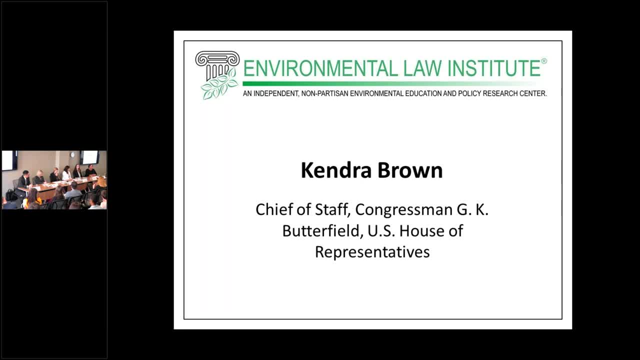 you know we're going to have votes shortly, um, i, if anybody has any questions, um, feel free to send me an email. so i'll leave some of my cards with you so that, if any of you have any questions, if you would like to come and have coffee, if you want to just talk, uh, i, i'm available. um, but i'm. 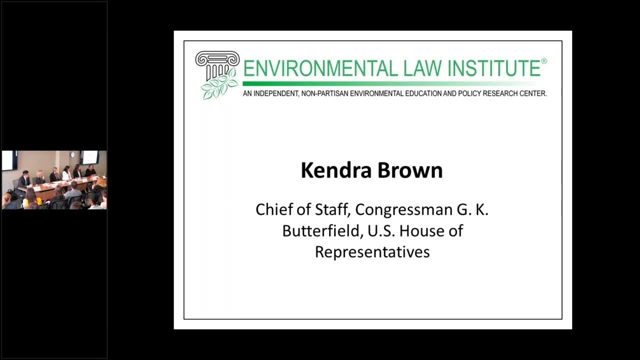 going to have to go back to you. i probably should share just a little bit about my background. i'm supposed to do that first. so, um, i hail from chandler valley, um, winchester, virginia. it's in the chandler valley just a few miles past, uh, fairfax. so i i love the mountains, i'm an outdoorsy. 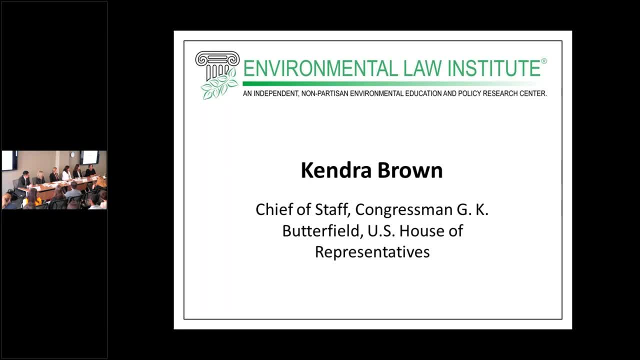 type of person. i went to hampton university and then, um, i went to howard for my master's of divinity, and then i went to vermont law school up in vermont, because, again, i like the outdoors. so i got my lom from george washington, um, so i began working on the hill while i was actually 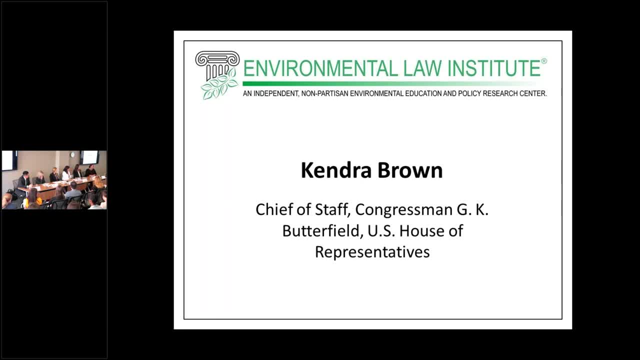 um in school at howard. so i started um on the staff of congresswoman maxine waters um and i was there in her office. um became her special assistant and then i went to law school and when i came back it was the summer of the bp oil accident, um, and so there was a lot happening um and uh. it kind of. 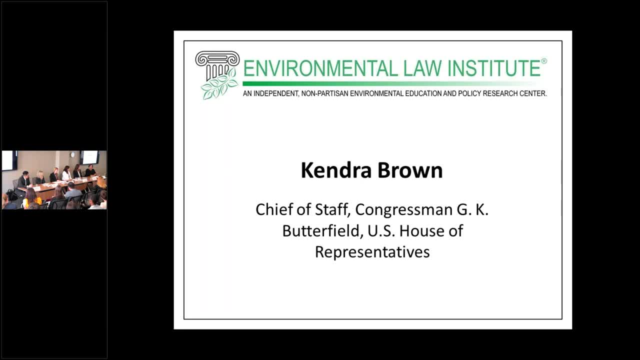 i learned very quickly what multi-district litigation was. that summer um, just really looking at, you know where the liability stood um, and after that i went on within law school to become the national chair of the national black law students association. so i did a lot of advocacy work um, and then from 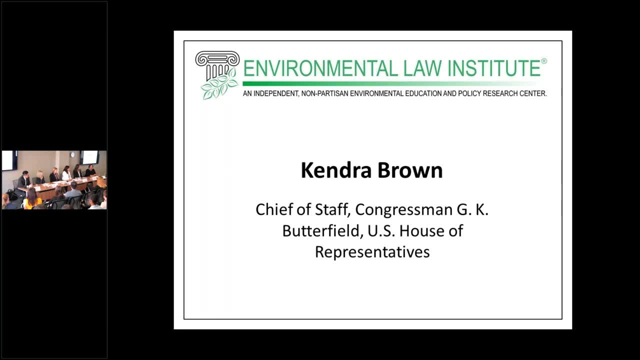 there after i graduated, um, i went on, i came back to dc, um, and i came back to congresswoman waters staff, um, and then i actually left to go to earth justice. so actually the office was a block away. i know they've moved now, they're a little closer to the hill, um, but i was at earth justice as legislative. 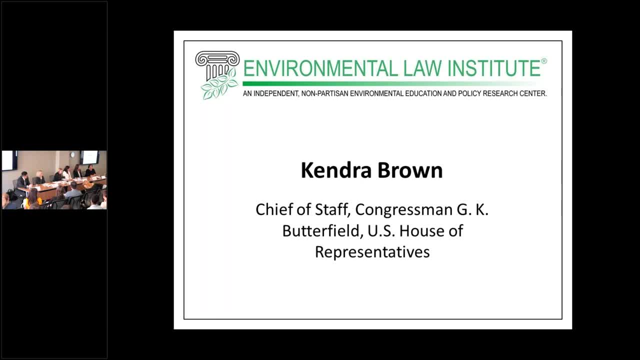 council? um, really enjoyed my time there. it's a wonderful, um wonderful organization. i still love the work that they do, um, but i left to go back to the hill. i got a call that there was a policy advisor opening, so i went back to be the policy director. 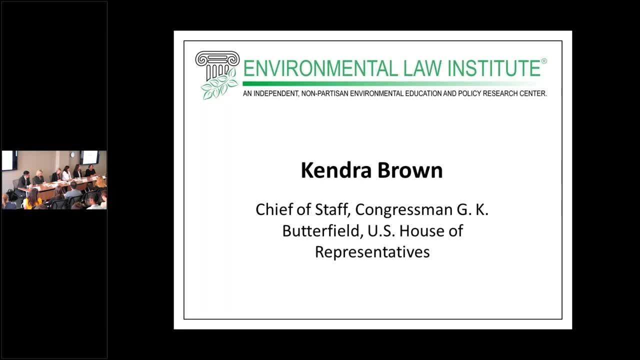 for the congressional black caucus, um, and so i was there for two years in the 115th and then i became the deputy chief of staff for a member from philadelphia, congressman, dwight evans. um, and then you know, i love the hill, but sometimes you just need to get away a little. 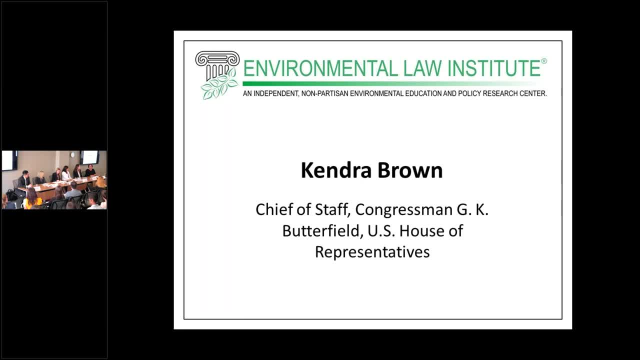 bit. so i went on to be the senior director for diversity at american university, washington college of law all of last year and tremendously enjoyed the work there, working with students, working with individuals within the profession, um and, you know, with the faculty. they have an amazing dean. dean canoe nelson is wonderful, so really enjoyed my time there, but i did get a call. 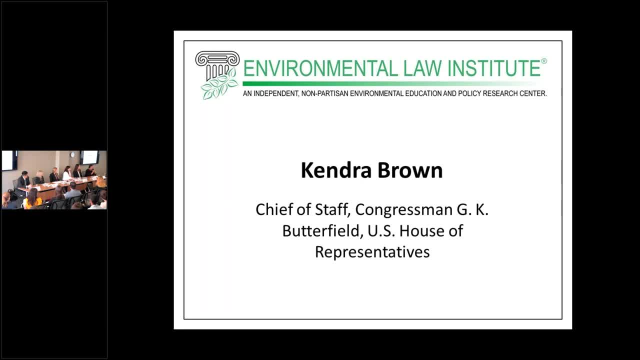 at the end of the year that congressman butterfield, um, needed a chief of staff because, uh, his chief was transitioning to um, you know, to a company, and so i came back in december and it has just been wonderful being back, just really helping people, you know, get placed in offices and 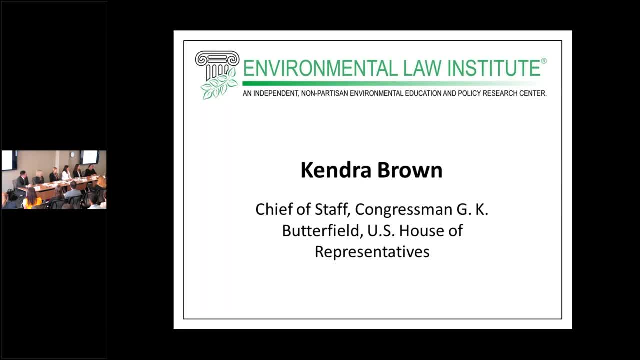 understanding where the opportunities are um and looking at the legislation that we are able to move forward. that is what all of the members and the senators are there to do. they are there to represent their constituents and to represent them well, and we're there to pass legislation. 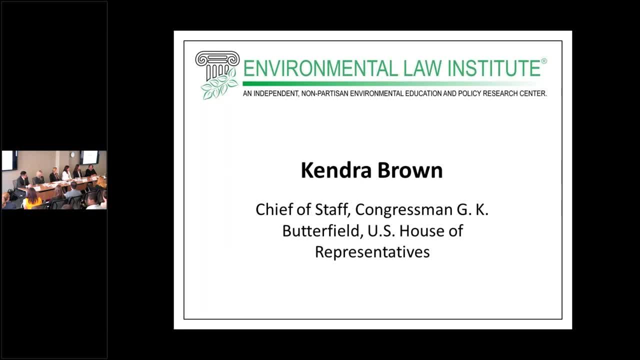 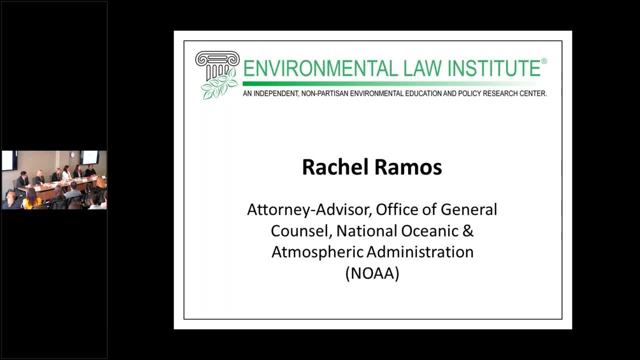 2017.. um, so i went to undergrad for environmental science and sociology and knew i wanted to go to law school to practice, specifically, environmental law. so i moved across the country to dc to go to georgetown, because i knew dc would be a great place to give me a lot of different experiences. 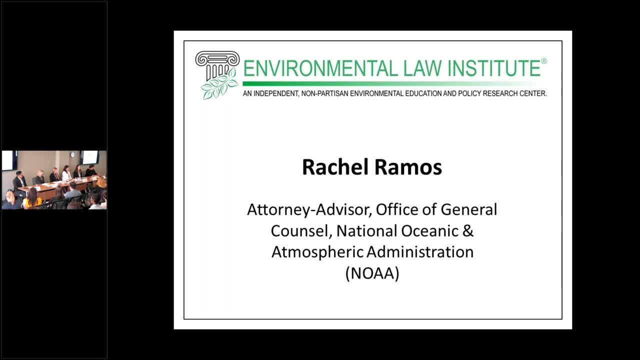 during the school year, since it's such a hub of federal agencies and non-profits, and so i all- basically everything i did in law school- was all very environmental law focused. i was very tunnel vision, i was obsessed with the clean water act and i interned at epa and i knew that i really liked. 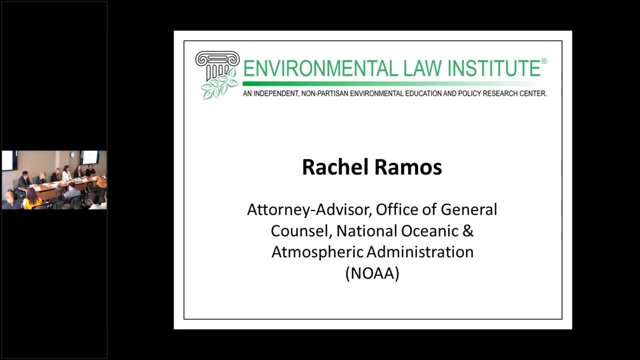 the role as a agency attorney for an environmental and scientific agency, and so i knew that upon graduation i was interested in entering the federal government. but i really did not know a lot about noaa, which is the national oceanic and atmospheric administration. noaa is how? 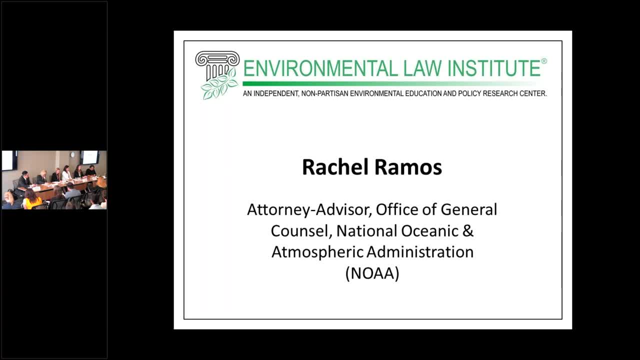 it all works in the israelian depart of commerce. um, i don't know if this is a joke, but it's just my joke. but then they're the agency that has the largest jurisdiction, because you're dealing with, you know, the bottom of the ocean all the way up to the atmosphere, with like satellite permitting. 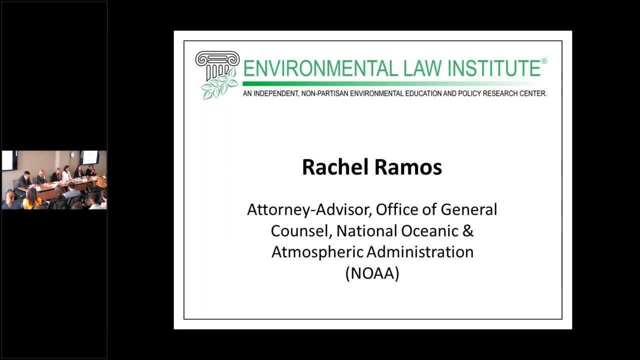 and space law and all these different really interesting, uh, privacy issues that i specifically don't deal with but that basically no one just has a really broad substantive area that it works with. um, it is an environmental scientific agency. um, i was really not very interested in the. 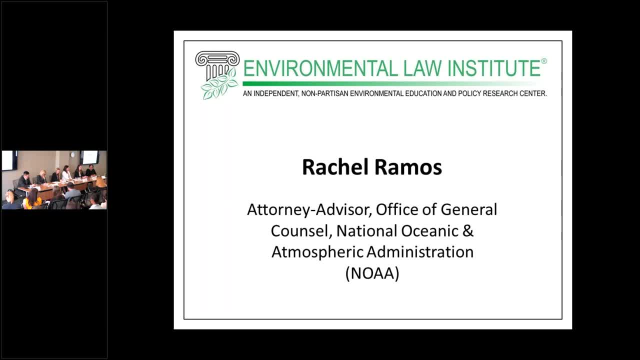 environment or in the space of them. there's no one specific area that it works within um. i was really not very interested in the space of them but i knew i wanted to do that. but it was focused on ocean and coastal issues in law school and I kind of I came into 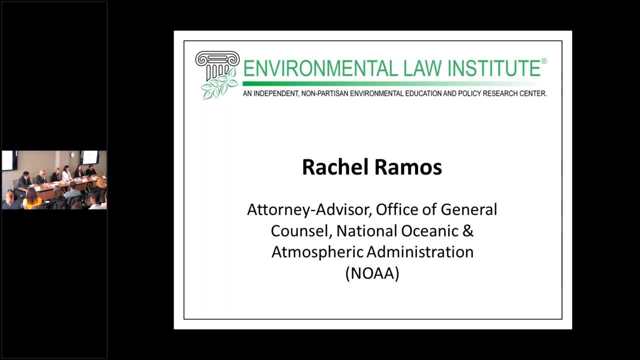 NOAA through the Honors Program. I didn't even know the Honors Program existed until like two days before applications were due and I happen to run into a NOAA attorney and a DOJ moot and an honors attorney and I talked to them and she sounded like she had a really good experience and I looked up the job. 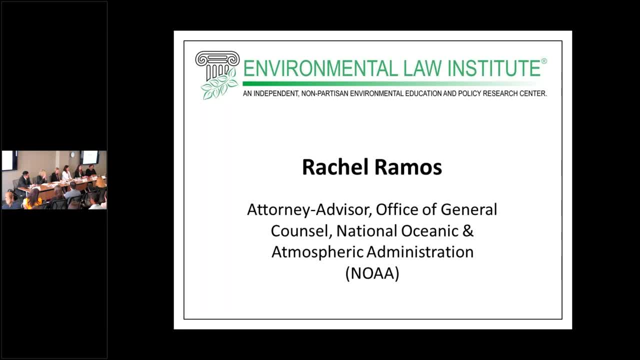 application and applied and it's been a really good experience. so I started with NOAA in. I guess it's September 2017 and the Honors Program is a newer government Honors Program. it's not as well established as like DOJ's Honors Program, which is huge. so I was in the third class of honors attorneys and every year 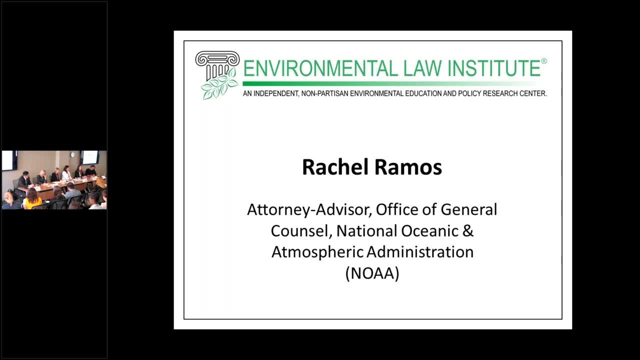 they have between one to four honors attorneys. my class is three and but it really is a neat program because you get the opportunity to rotate within NOAA General Counsel. so the way NOAA general, NOAA attorneys are set up is they're all housed within general counsel, but there are many. 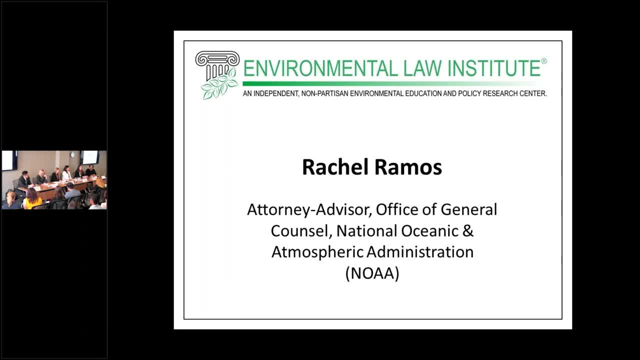 different sections and each section deals with very different substantive areas of law and also your role as an attorney is going to be very different in each of the sections. so you get to do three six-month rotations. you get to preference the sections you're most interested in. they try to match you but 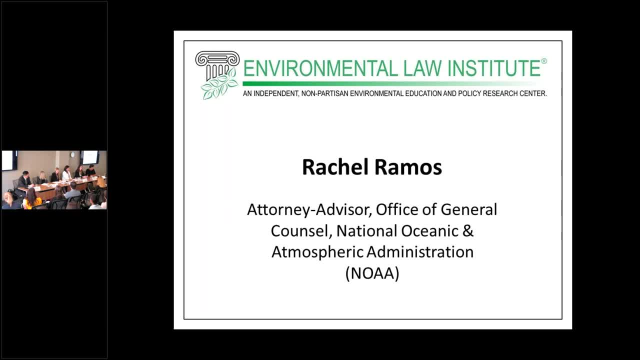 it also has to do with need and you know managers desire. so I did my three rotations and then at the end of the rotations you get a permanent placement and you're, you know, guaranteed a permanent placement. so it's a good experience as a new attorney to get learn about diverse roles within NOAA but then still know. 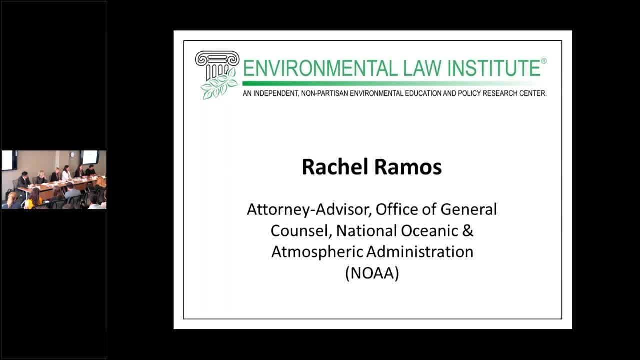 that you're going to get a permanent placement at the end and not have to job search again. so my first rotation was in the enforcement section. that was a really great experience. the NOAA enforcement section deals with the Magnuson-Stevens Act, which is the fishery management statute. so, like if I had a Magnuson-Stevens Act case, it would 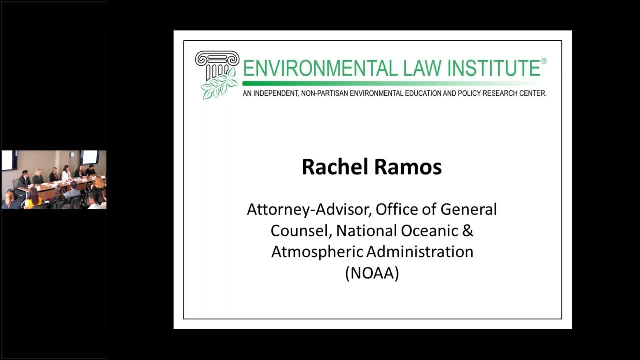 be with various types of illegal fishing, like overfishing, using illegal equipment, fishing in illegal times like the seasons closed. you also have Endangered Species Act cases, marine management, marine mammal protection act cases, National Marine Sanctuary Act cases and basically on my first day I arrived and got like a 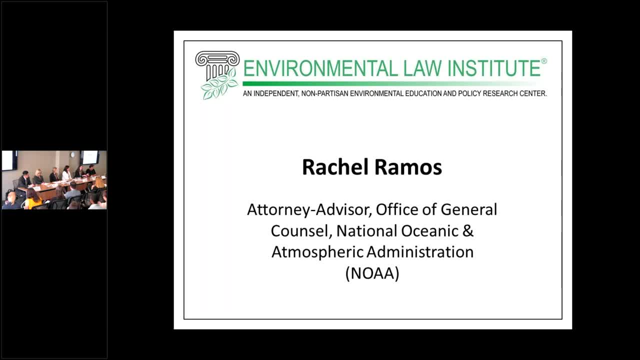 stack of folders and they were like: oh great, go ahead and you get. you have an investigating officer that puts together a file of facts and then, as an attorney, you look at it and decide: do you want to charge this person? how do you want to charge them? it's all civil cases. you're working on civil monetary penalties, but 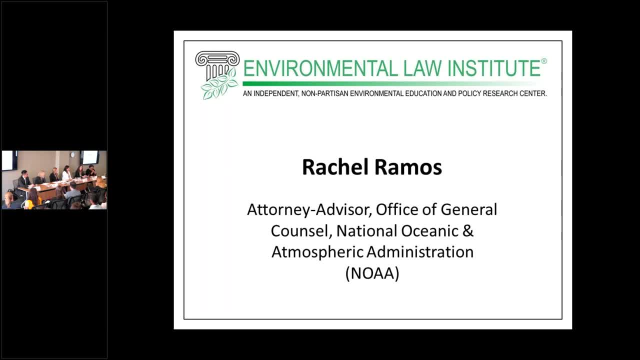 there's a lot of judgment that goes into figuring out where you are on the scale, this penalty scale, and another great aspect about this section is that you're it starts in administrative court, so you're in front of an ALJ, which means that you don't actually work with the DOJ attorney until it gets appealed into. 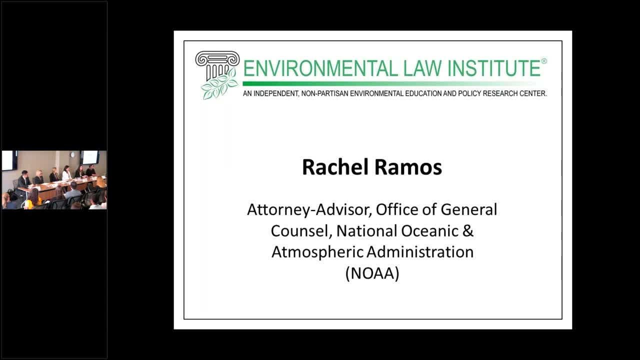 trial court, so I mean a federal district court, and so it's a really good experience as a new attorney to work on a small discreet case on your own and kind of learn some tough lessons and get to be lead attorney and you send out notice of intent to sue and you're working directly with the prison counsel. 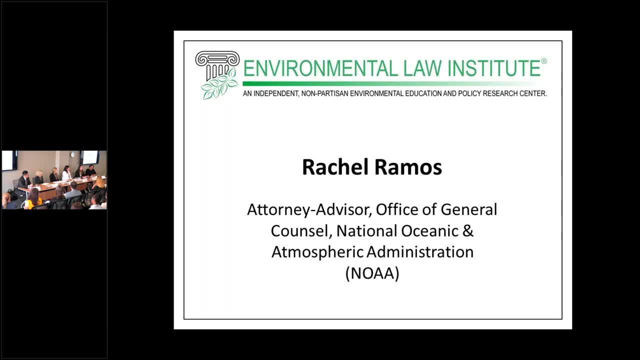 so that was really good experience. and then my next six months I was in the oceans and coasts section and that role was much more of an advisory role. so my client was the NOS. I worked with the National Marine Sanctuary office and specifically the Monterey national marine sanctuary, and helping them draft. 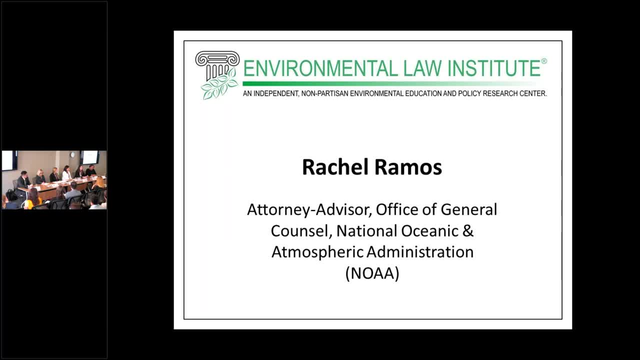 regulations and provide advice on different legal issues as they arose. and that was really fun because every day was really different and it was oftentimes kind of discrete, smaller issues. you had to be much more on your feet and i was constantly in meetings. um, i got to do some nepa work and it was a really diverse work portfolio. and then my final rotation. 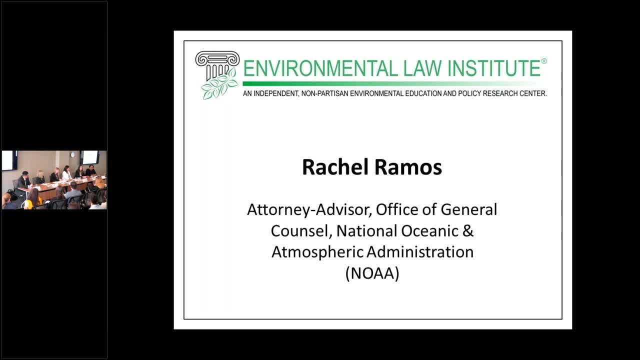 which ended up being my permanent placement, which i was really excited about, with the natural resource section, and so in that section you're doing natural resource damage cases which i didn't know anything about in law school and i really didn't know anything about until i started in the 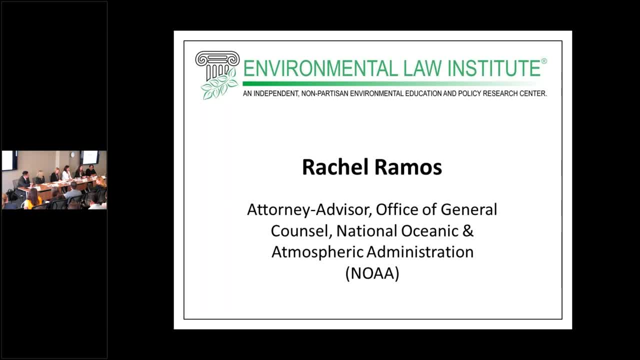 section um. so in that section you're working with circla, the oil pollution act, the national marine sanctuary act, um. in law school i learned about surplus, but i only learned about the remedial side, so the cleanup side. so that's the work that epa and the coast guard do. they are like kind of the 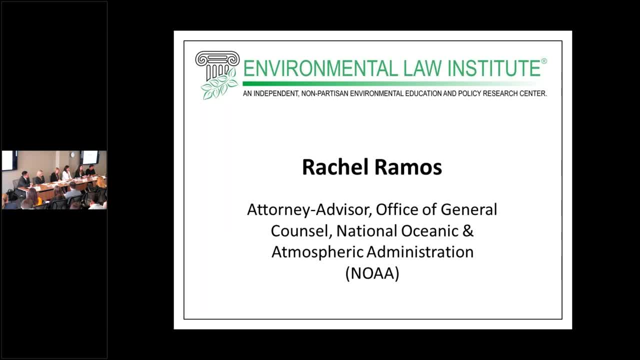 first responders and their task is to um. they have human health-based standards, basically. so they're going in and they're trying to prevent any further human health or environmental harm by removing the contaminants. and then the second phase is the restoration phase, and that's when noah comes in. 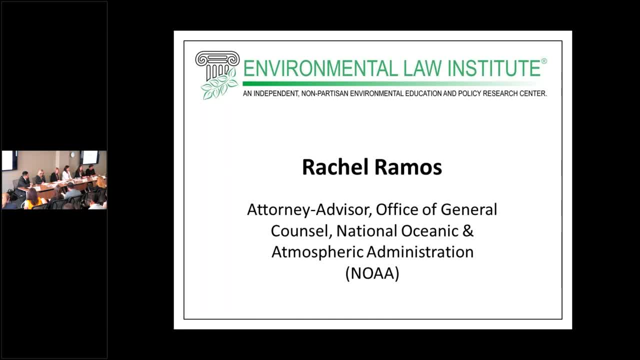 as the restoration trustee agency and their goal is they don't have these human health-based standards. their goal is to basically make the ecosystem whole again, so it's much more habitat based and you're dealing with the natural resources that noah has jurisdiction over. so, um, you're, it's- it's really fascinating, and noah is usually working on a team of other trustee. 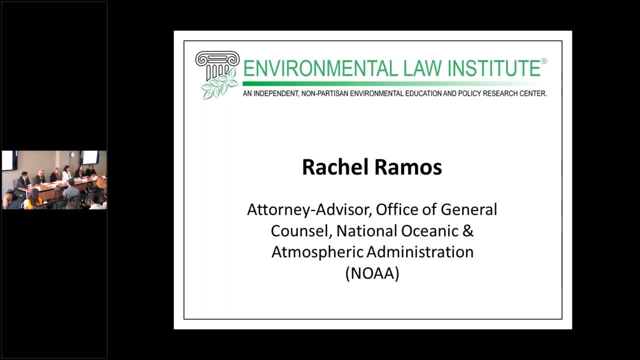 agencies. so you're getting the chance to work with department of interior. um, you're working with tribes- usually, usually there's one or two tribes on a case. you're working with state agencies and you're all coming together as part of the trustee council to basically move this. 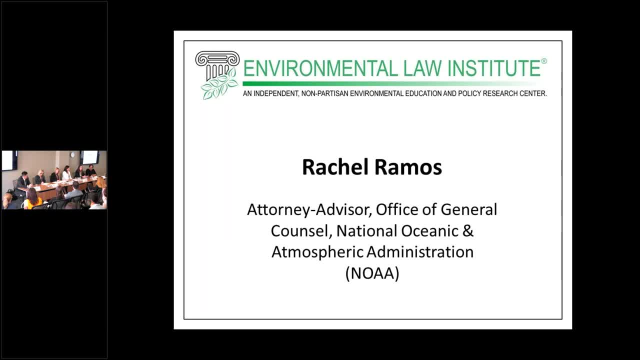 restoration uh case forward and um, each case is really different, and getting to work with different tribes is also a great experience. um so like, i have one case where this yacht grounded in a sanctuary and tore up a bunch of corals, and then i have another case which, um is an oil spill case. 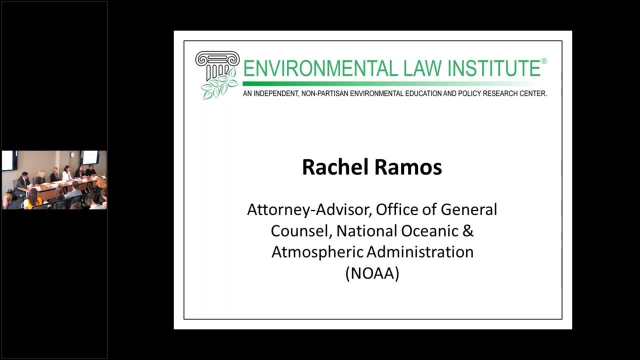 and that's, you know, just really different tempos and you're doing really different players. um, i have a few cases that are complicated, circular sites where there's been ongoing hazardous contamination for years and the epa remedial side is they're finishing up and then we come in and we 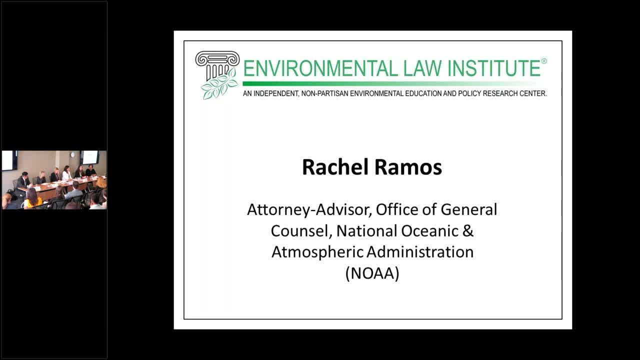 have our our assessment um, and there's, i guess, two big phases where you first are in the injury quantification phase, where you're trying to really quantify the damage that's been done to the ecosystem, and then you translate that into the restoration um, where you're um trying to figure. 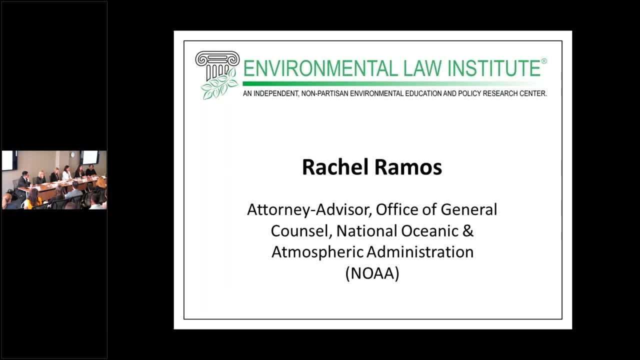 out. how do i you know what restoration is needed to make the space whole again from this specific injury? the work is also interesting because it's a lot of um like pre-litigation. most cases settle out and so you're dealing with lot of negotiations instead of the litigation, except i do have a couple of cases that are going. 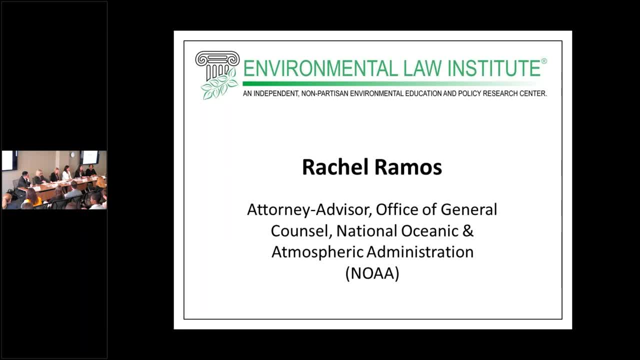 barreling straight towards litigation, but it's a great space to work in because it is very interdisciplinary and very stimulating. so every day i'm working with scientists and restoration experts and economists and, um, it's just, it's the opposite of boring, like every day is very. 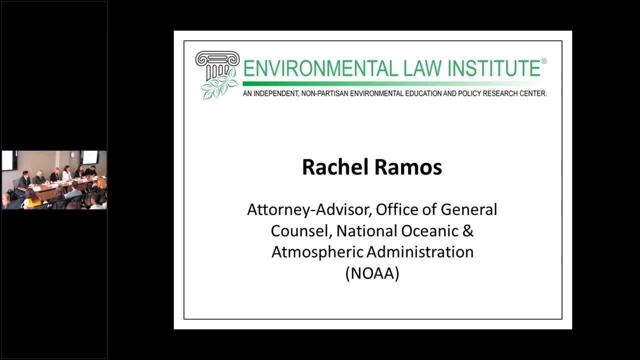 different and it's really neat as an attorney to have to issue spot in these different areas and work with these folks that are all really passionate and motivated and they all have like phds and these crazy degrees um, so it's been a really good experience so far. um i you know like 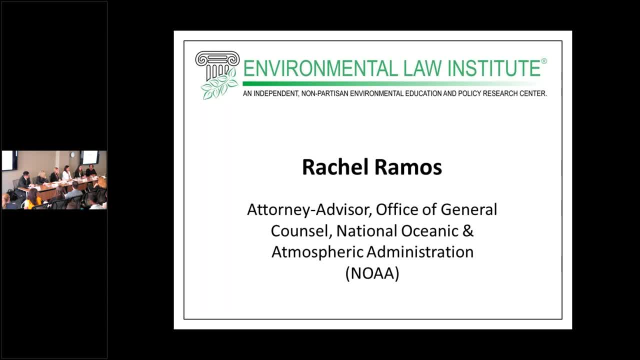 i said, i haven't been practicing for that long, but i feel like in the short amount of time i've gotten to see some really different roles that are trying to play, and that's taught me that, as a young attorney, i think it's really good to get these different experiences, like whether you're going. 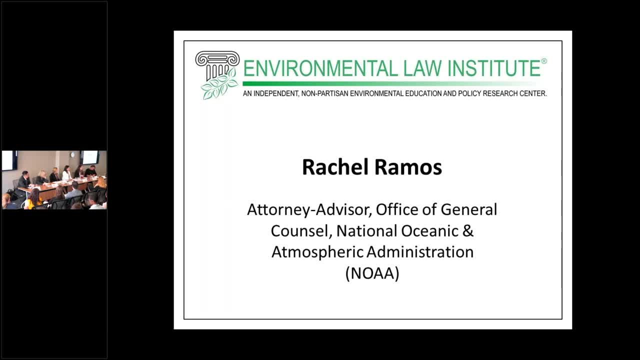 through different jobs. um, or i somehow managed to do it in a single job. um, it's good because you learn what you're actually comfortable in. um, like i think toby said, you thought you wanted to do something but you actually didn't. it took a while to learn through your career. um, and that's. 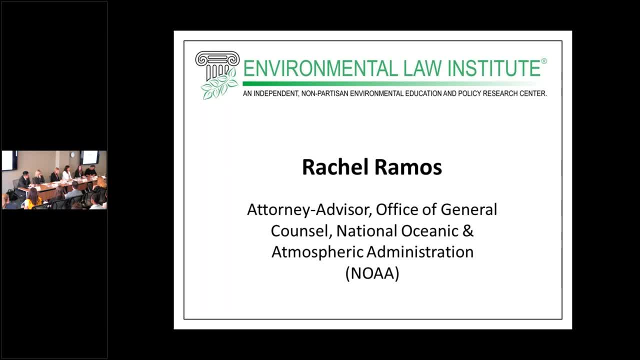 i mean, i felt the same way. i didn't even know i wanted to have this role. i didn't know i would like to be, you know, negotiating with the opposing counsel and that, and it's a different skill set. and i think the other thing that's really inspiring about it is that it's not the typical um like. 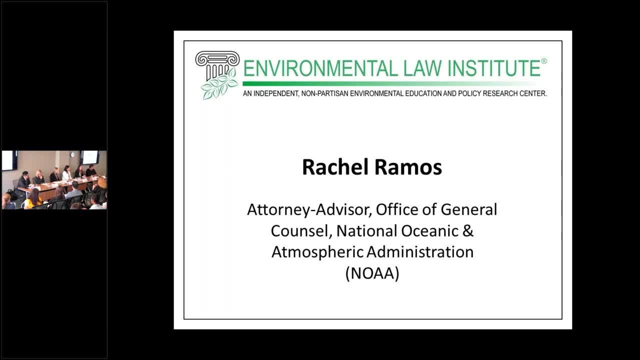 research and writing that i had previously associated with being an attorney. it's much more um talking and kind of you're working with a big case team and kind of hurting people in a way and managing and it create. it uses a lot of different skills and so i guess my takeaway is that there's 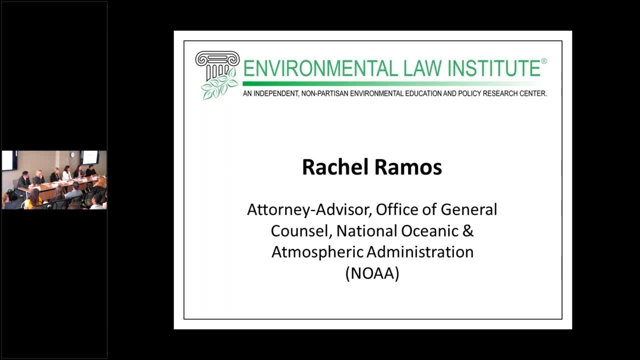 just um. you think you're in law school, i i know i wanted environmental law and i knew that i wanted. But even within that I didn't know what my future would hold and I have, I think, a really different career trajectory than I initially thought I would. 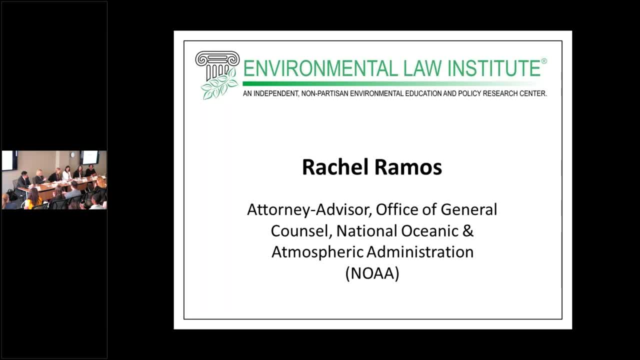 Thank you, thank you all so much. I will speak very briefly from the NGO side and then we will jump into Q&A and we'll start with Kendra so she can make it to her votes. As you all know, you are here at ELI and we are a nonpartisan environmental think tank. 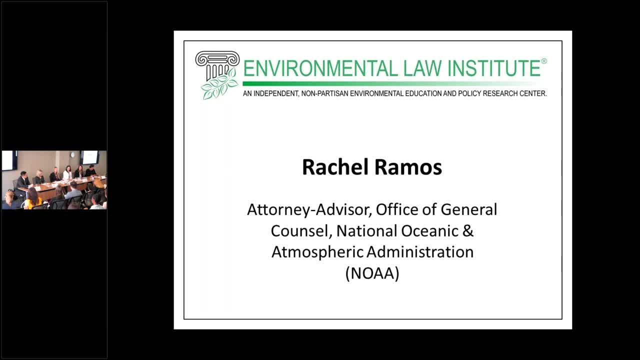 We kind of straddle an interesting space as such. So ELI's slogan is making the law work for people, places and the planet, And that kind of intersection is really where we work at across the board. So being a nonpartisan group is always interesting, and especially in recent years, as 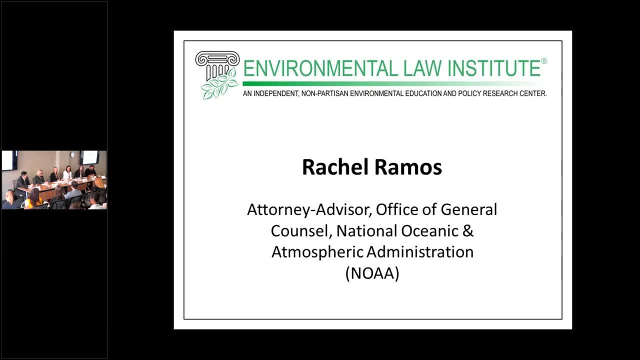 things have become increasingly politicized within a really beneficial space for us to be in, because we are really viewed as, and really strive to continue to be, this sort of big tent convening space. You see that on our panels We always have a range of members and folks involved here with ELI. 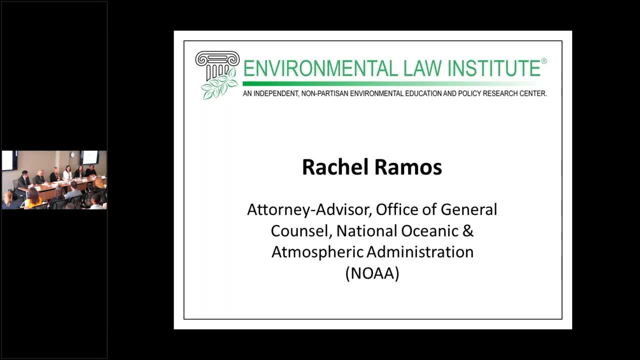 We are a publishing house. We publish various textbooks, the Environmental Law Forum, journals, articles, blog posts. We do a lot of research here. We do a lot of research throughout the United States, throughout the world. You know it's a smaller staff that just does this amazing amount of work, kind of all over. 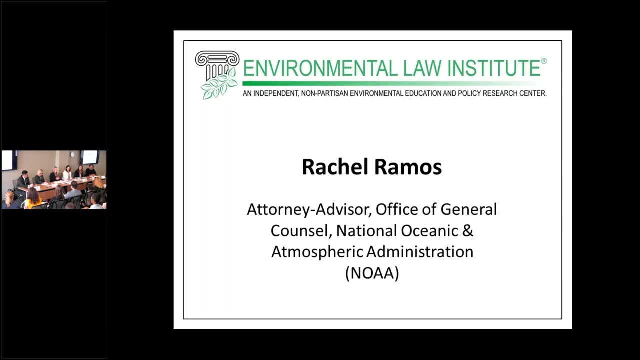 And it's really interesting to have all these different components work together, which I do think you tend to find at nonprofits is: one person never wears just a single hat ever. For me here at ELI, it's really interesting. It's really interesting. 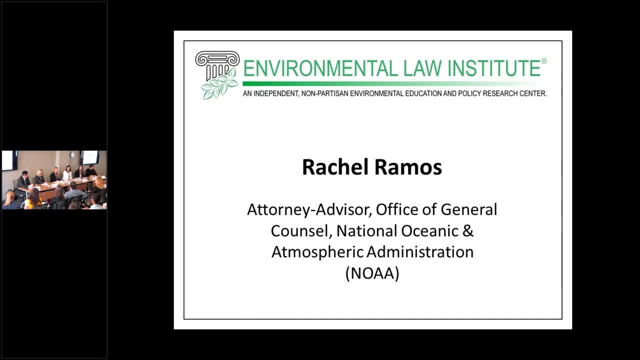 For me here at ELI that's been a really amazing experience, that every day is truly different. The Associates Department largely runs all professional education as well as the bulk of our membership. So on the professional education front, of course, we put on summer school. 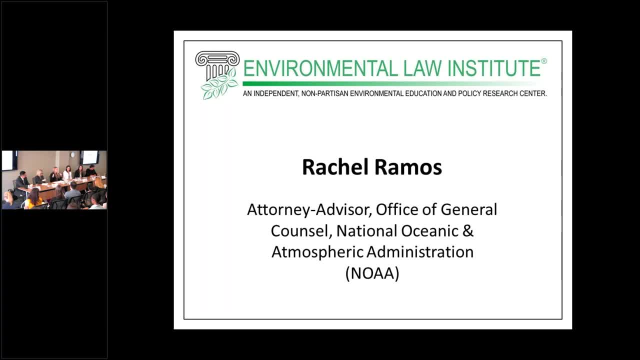 We put on two annual boot camps to really give people a deep, deep dive into environmental law. And the way that I really see and what my passion is based in here is how I can be of benefit to others, how I can help others learn more. 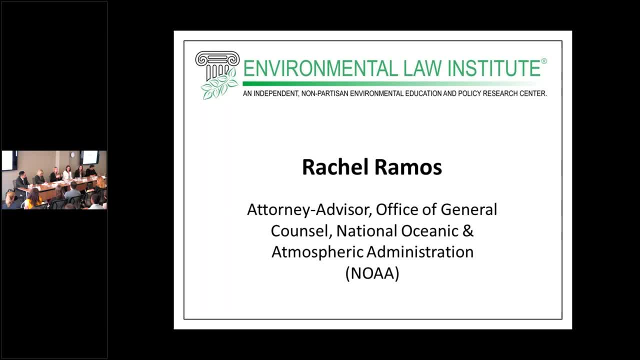 what can help their work? what can further environmental work in general? I personally am not someone who loves researching only one thing for years on end And every day. it really is something new here And it's fun to just research something, just to the extent that you can bring people together. 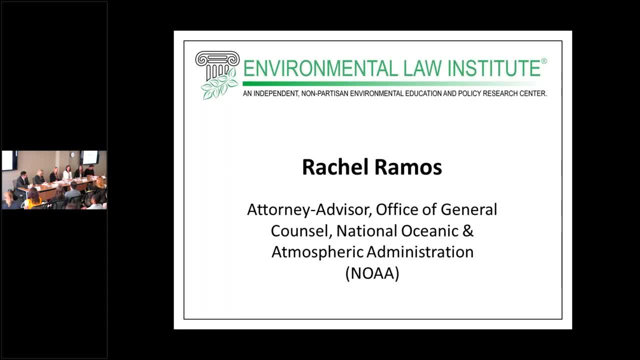 And further the conversation around that. In terms of the members of ELI, that spans from corporations to those in private practice, a lot of engineering and consulting firms, a ton of other NGOs, academics, government folks- Really across the board. we try to bring people together. 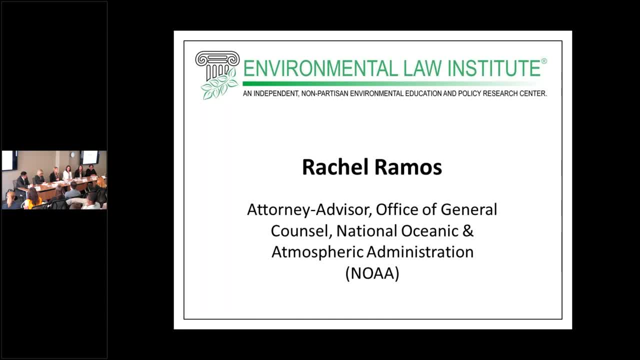 and try to see how we can further and push environmental work in a beneficial way forward that works for people, places and the planet. I know I kind of sound like a commercial right now. I do want to make one plug: that all of our student memberships are completely free. 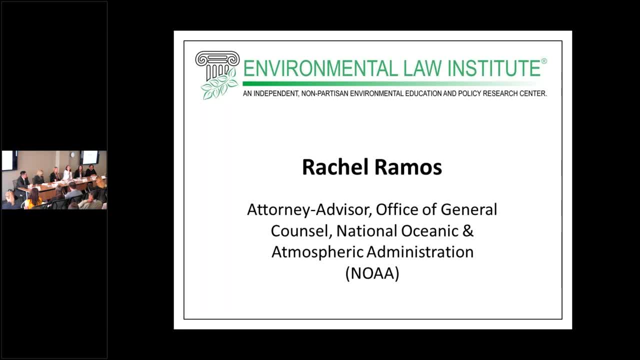 and I would encourage you to join us. We have a lot of resources that are not only readily available to you, but that we want to be of good use to you and to others. Going back to wearing different hats, I think that, as you determine what's right for you, 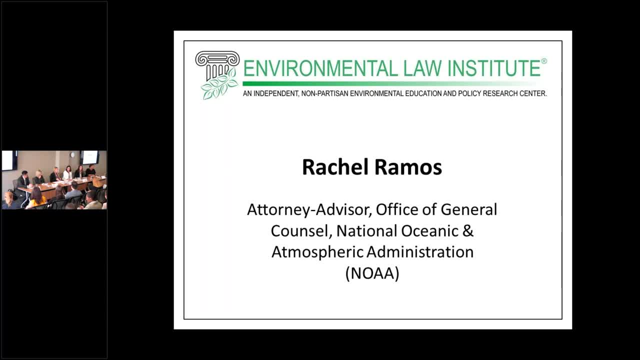 it's really important to know whether you want to take a deep, deep dive into something for weeks or months or years, or if you're someone that needs more of the constant change In any given day. here at ELI, we work on running summer school. 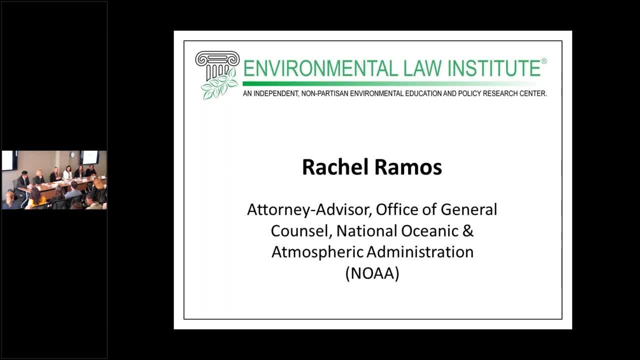 We've started a new podcast, We have a new emerging leaders initiative for younger folks to join the really emerging leaders in the environmental field space, And this year is ELI's 50th anniversary year, which has become a celebration of each month of a different environmental topic. 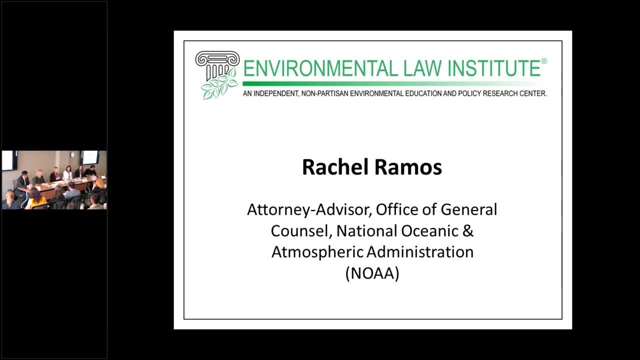 that we've based more programming and blog posts and publications around. So that kind of constant energy of what's going on here and here and the fast-paced nature of it is something that is really important. It's really not unique to NGOs, but something that you do find very prevalently there. 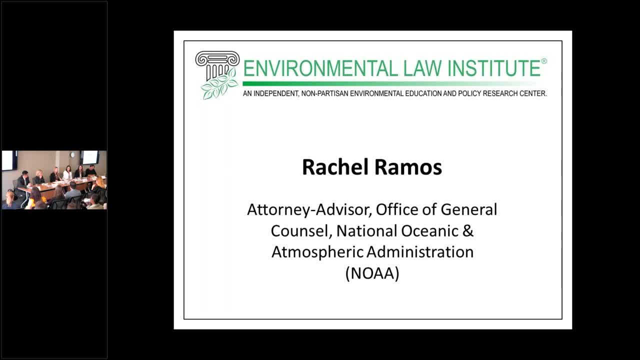 And it's also a space where you get to just be with people all the time. That's by far the best part of my work here at ELI is being with amazing expert panelists and learning from people all the time. So I think, that being said, we should jump into Q&A. 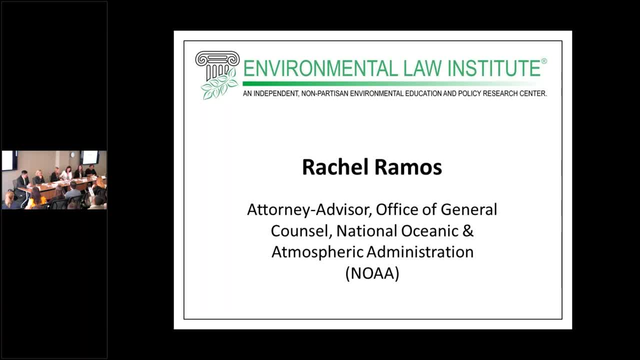 We'll start with Kendra. if you don't mind, I will start us out and warm us up with a question and then, hopefully, you all are inspired to follow suit. So, Kendra, you have worked in academia, You have multiple degrees, NGO. 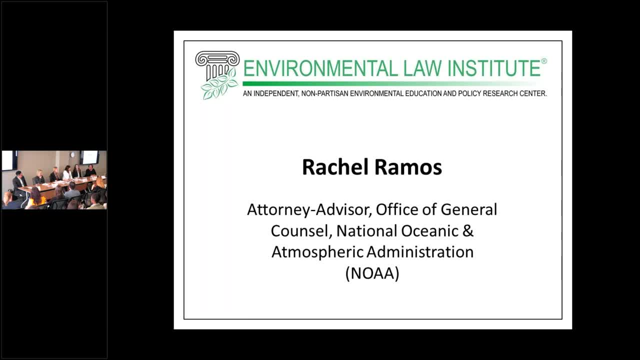 You've worked on the Hill several times. How have you faced the transition through different things? What challenges were part of those transitions when you're going from something pretty different from the next, And what were the positive parts of that as well? Yes, thank you for that question. 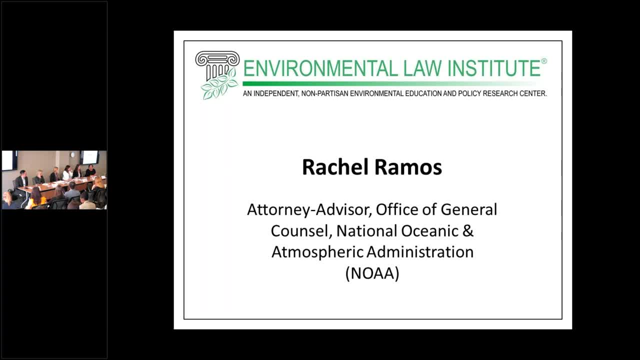 I think that one of the transitory takeaways is that one entity that always goes with you are the skills that you have, And for me, I always had just a heart for advocacy and for people, And I live by this motto that I always want to make a difference for as many people as I can. 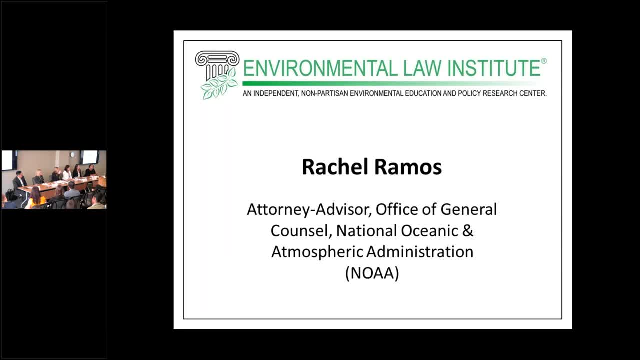 as often as I can, And so I think that for me, in every role, that's what I have always tried to do. Even when I was at Earthjustice, I was still involved in a number of boards where I was working with students on their professional development. 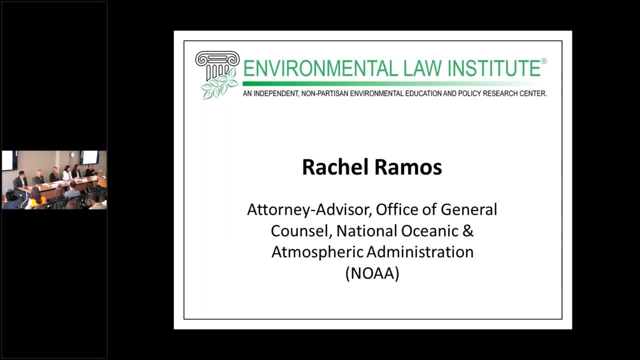 And so that naturally just helped me, Naturally just has always carried me through that commitment to student achievement and to professional development, And I have always had a heart just for people and for serving people, And so I think that for me the transition has always been about 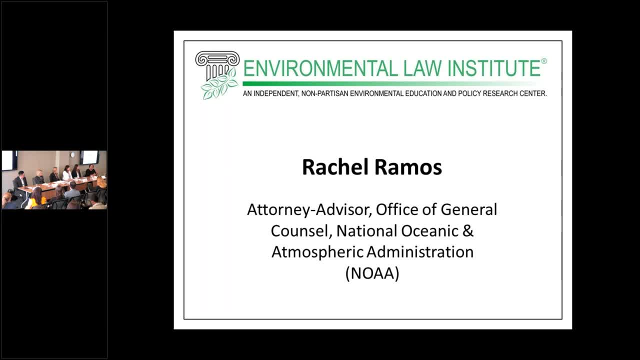 how can I be of service to those that I meet, to those who I am a part of their life? Congressman Butterfield, we have over 750,000 people within the first district of North Carolina, And so those are the people that we serve. 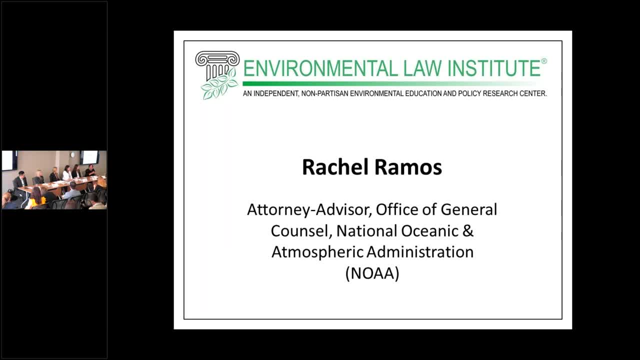 Those are the individuals that we serve And that entire area, including the environmental impacts of everything that's happening in that area. environmental justice- the birthplace of environmental justice- is right in CO1. And so there are just so many ways that 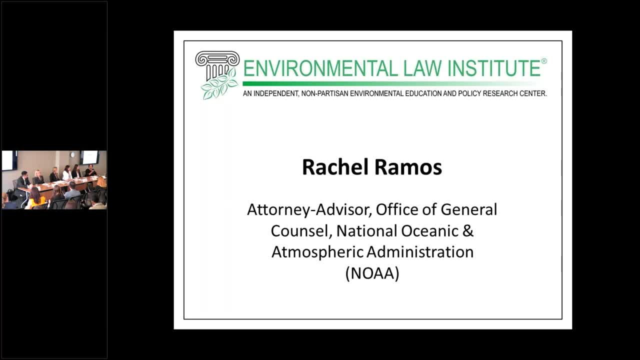 for me, the common thread has been service to others, be it students, professional development for others, ensuring that there's a pipeline of individuals who are coming onto the Hill, passing legislation that has impact on the constituencies that we represent, looking at how we can expand the base of research. 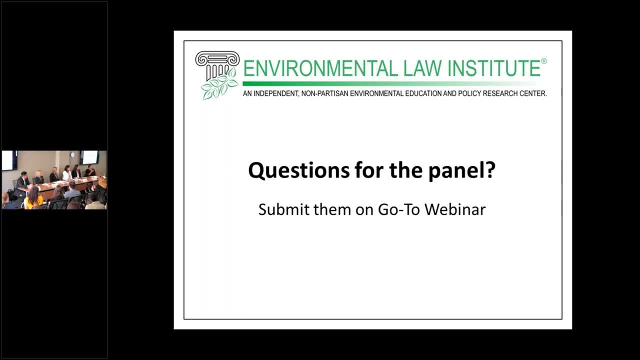 from the academic side to support the work that we're doing either on the Hill or in student affairs. so for me there are common themes that exist in all the roles that I've had. Great Thank you, Kendra. So for our folks on the web, 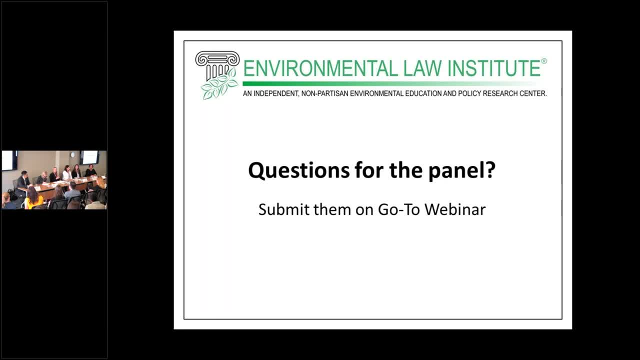 I do want to remind you that you can enter your questions by typing them into GoTo's question box and don't be shy, And our colleague Hannah will come around with a microphone now for anybody who has a question for Kendra Blessings. 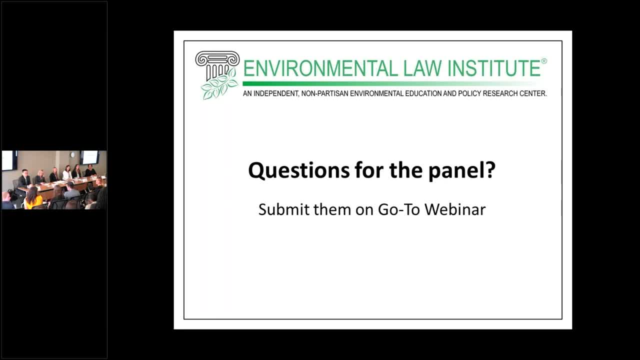 I am Shara Thompson. It's wonderful to meet you. Thank you so much, And, Kendra, thank you for all that you shared And each of you, and since we're asking you questions now, I would say that as a Black woman, 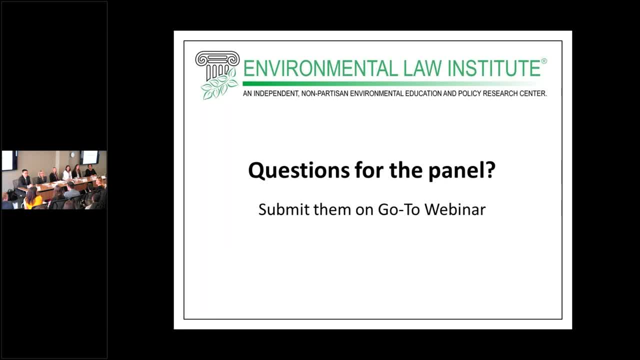 there may have been some obstacles that you needed to overcome in order to establish yourself, And so, while all of us here aren't Black women, some of us are. there may be certain times where we may have to overcome an obstacle, whether that be because of our age. 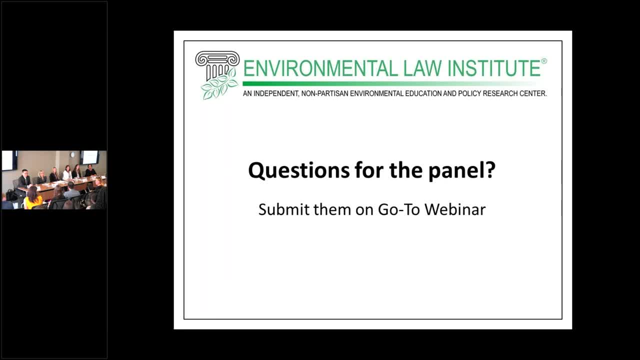 or whether it be because of the color of our skin or because of our gender. What wisdom would you have to share with us? Thank you for that question. Overcoming obstacles is something that is par for the course for each of us. I think that for me. 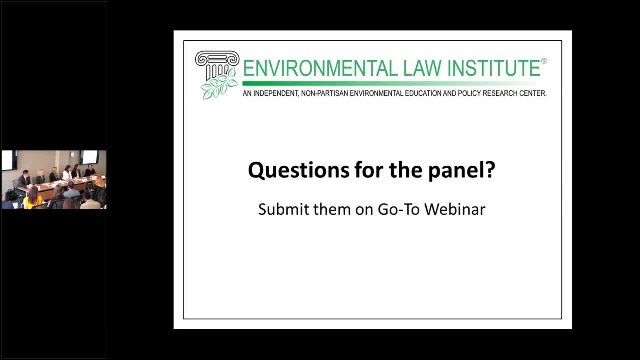 I am first, you know, the daughter of Paul and Dale Brown, So my parents- a lot came with that right. My father was the assistant principal of our high school, So there are pros and cons to that, And so for me, 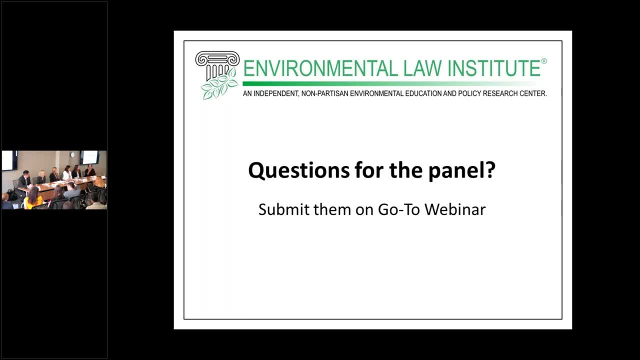 so that's like first Second, who I am as a person And when I was growing up. I don't typically talk about this one, but I will talk about it, So I had a stutter from the time I was about five until I graduated from college. 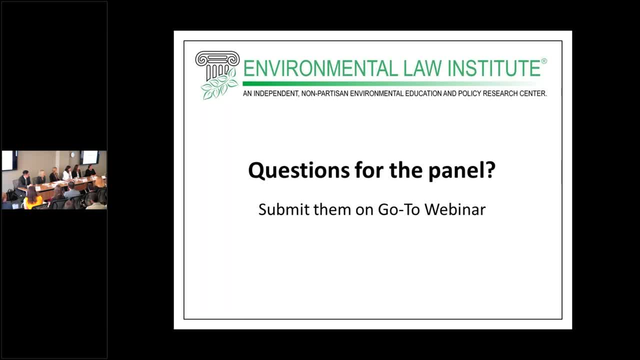 not high school college, And so, in addition to feeling that sometimes, as a Black individual, I did not, I felt that I didn't always measure up to those who were around me, because sometimes that is how the media portrays those who look like me. 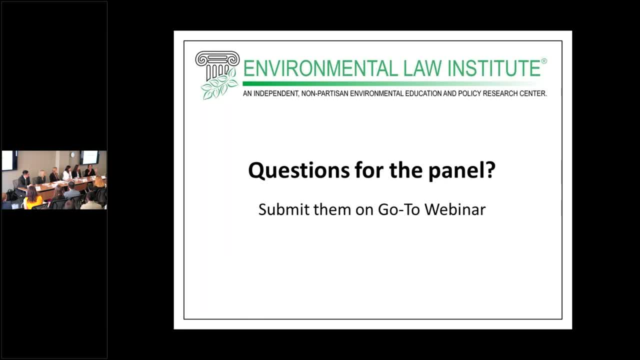 There are lots of images out there that you see, where you feel like that is the normative view of how people are to look, And if they don't look like this, then there's something that you know is amiss or off. 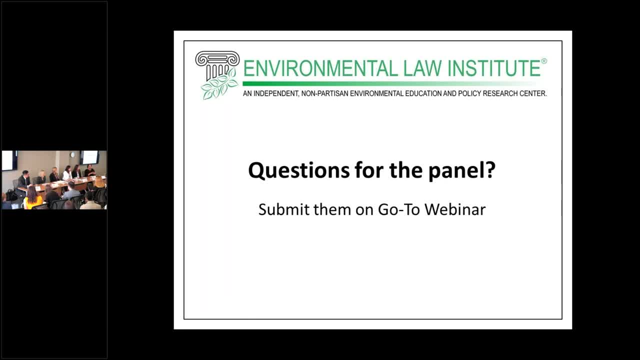 And so for me, I had to one learn how to love myself, You know, as a Black child, as a Black woman. But then, with this stutter that I had, people would actually laugh at me. They laughed at me constantly. 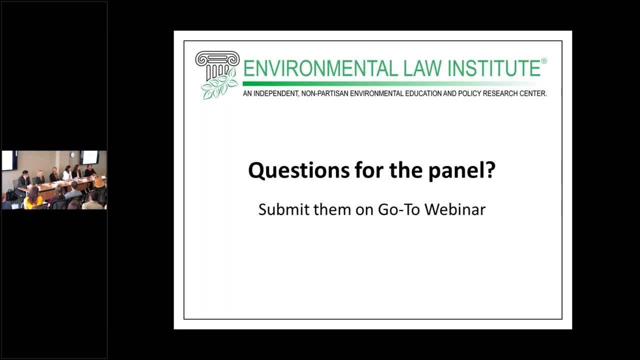 And it was very difficult for me, And so growing up I faced that constantly And so for me that was that really has been the number one obstacle in my life, And it's nothing like being in middle school and like a teacher. 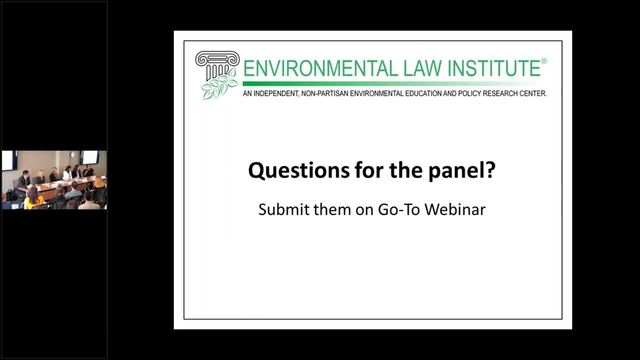 a caller. I felt it that the teacher called on me more. She probably didn't. I felt that she did, And I was always in trouble because I was. you know, when I did respond, it was typically something smart, And for me, 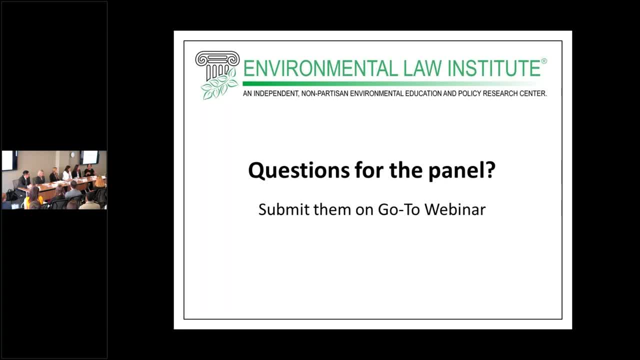 that's how I acted out, what I was feeling and what was happening to me, So that obstacle. ironically, how I overcame that when I was at Hampton University, my beloved historically black college and university, otherwise known as HBCU. 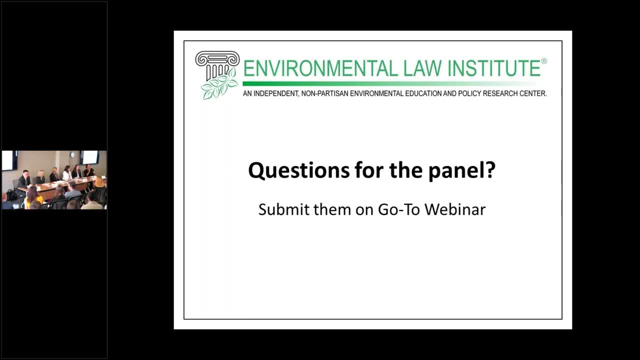 How I am. Okay, how I am. So I went there for my master's. Yes, So it's this rivalry between Howard and Hampton. We can talk about that later. But when I went to Hampton, I worked at night at a telemarketing place. 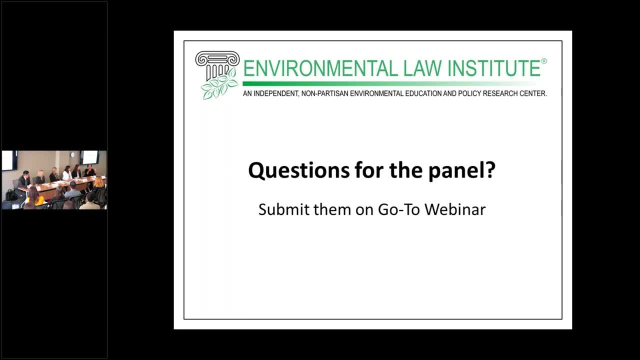 And so when I worked there, I had to read these screens. So it was like, why would I go to a place, Why would I go to a place where I had to read constantly? But I knew that I had to overcome that challenge. 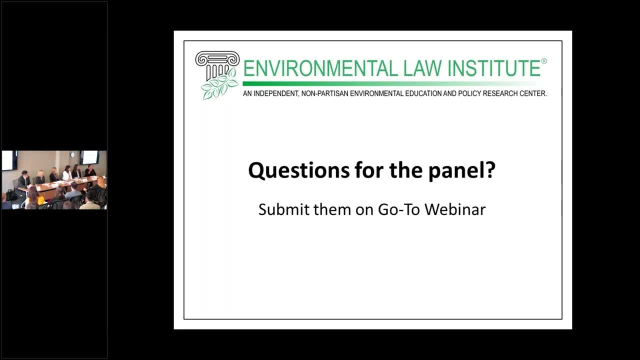 And I knew that there was going to be some way, somehow, that I was going to do this, And so I would sit there and read, And I remember one night a call came in. So it's like those ads you see on TV, right? 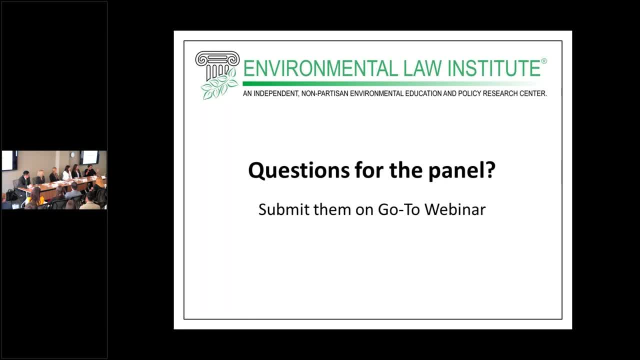 So it's a lot of older people that sit up and watch TV, And so it was an elderly lady that called. She was the sweetest lady And she could tell I was having problems reading the screen, And so she said: just take your time. 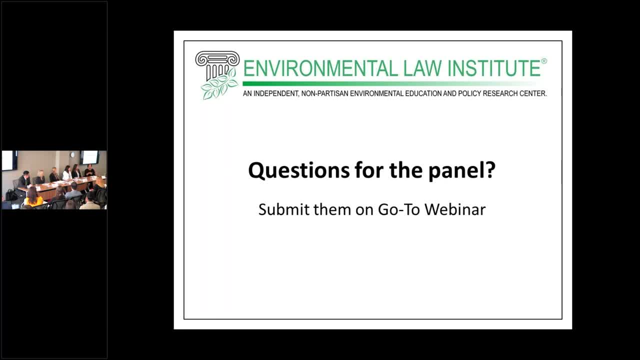 Just take your time. And she really encouraged me to learn how to pace myself. And so, from that job that summer- because I stayed there for that summer- from that job, just in that amount of time. I overcame that, But I overcame it by facing it. 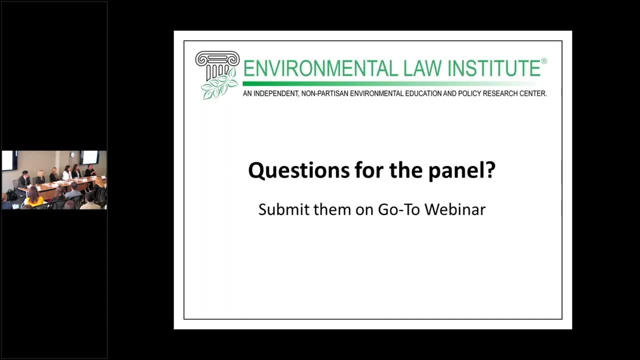 And so I say that to say that oftentimes we will have situations that we will have to face just negativity, issues of, you know, lack of diversity, lack of inclusion, etc. We all see what happened to Kamala this weekend, You know, with the individual, 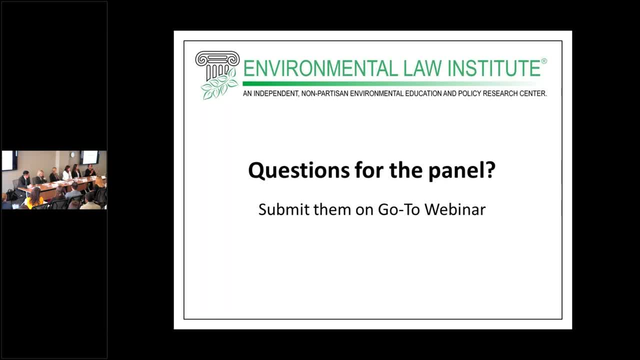 that came on the stage where there will be times where there will be negative things happening to us. no matter where we find our self in life, no matter who we are, there will be negativity, But you just have to understand that. you have to push through it. 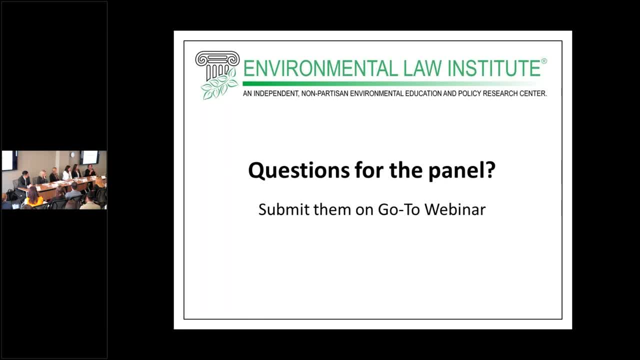 and that you know the storm only comes for you to learn how to navigate through it, And it happens for each of us. Sometimes it's figuring out if you want to, if you want to take another role. I will admit that when I was leaving Earthjustice. 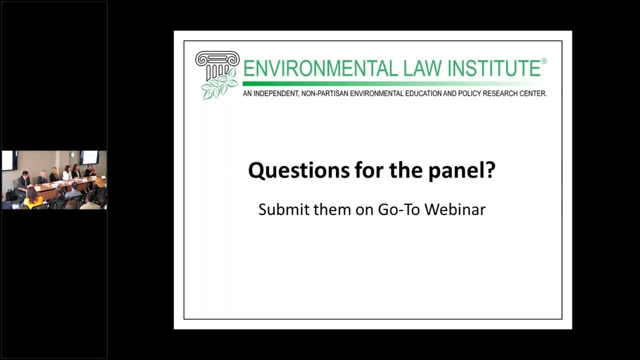 I did not want to leave Earthjustice. It was a wonderful place to work. You should all look up Earthjustice. It was a wonderful place to work, Wonderful balance, So wonderful staff, wonderful attorneys. I did not want to leave, but it was the time that Loretta Lynch 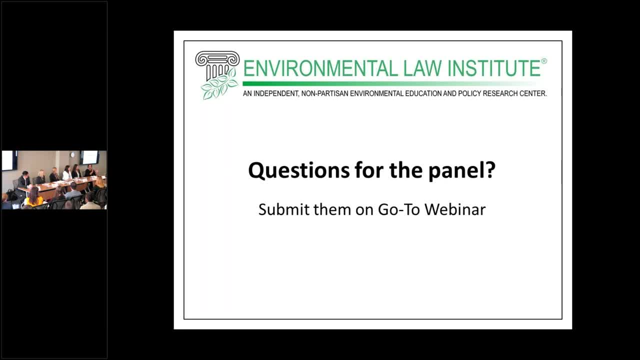 was being confirmed as the Attorney General, And it was that fall, And so there was a lot happening And I felt that for me, for who I was, because I needed to be back on the Hill, because I needed to be in that. 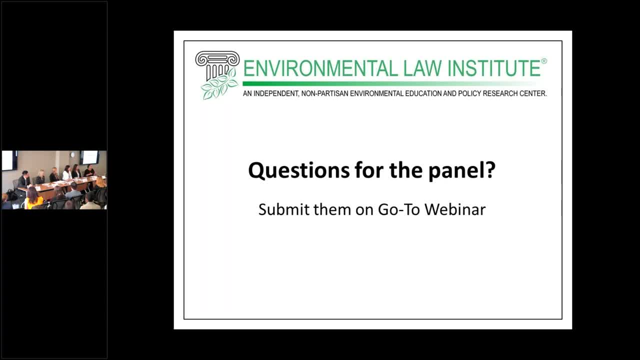 in that turn of ensuring that she got to where she needed to be, ensuring that we were passing legislation and moving things forward that would help individuals that look like me, So that's why I went back to work as Policy Director for the Congressional Black Caucus. 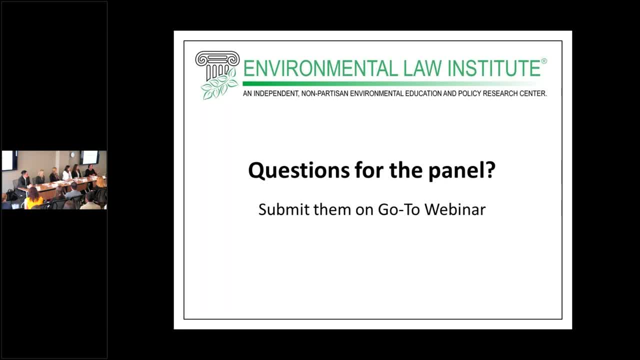 So there will be times in your life where you will have overcome an obstacle just to be in a place where you can help others overcome theirs, And so that's why I went back as Policy Advisor, you know, as Policy Director for the CBC. 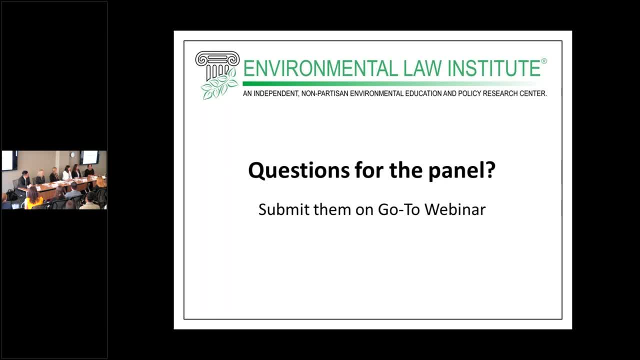 So I say that to say sometimes things that we overcome are just so that we can help others who either look like us or who have been impacted by negative legislation that has been passed that has a disparate impact on the communities. Looking at you know. 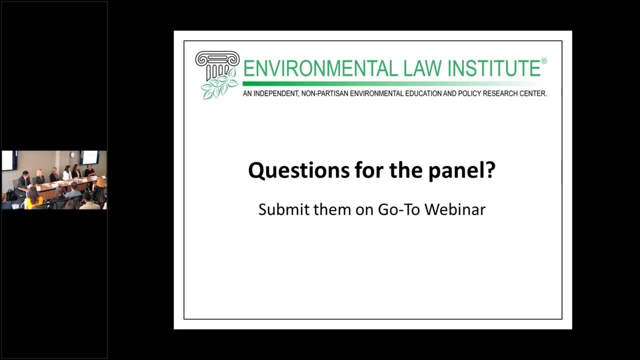 like what the environmental assessments are. you know within, you know communities, just ensuring that those are at hand when there are, when there are companies and things that come into communities, And so I think that that's also one huge way that we can just have an impact. 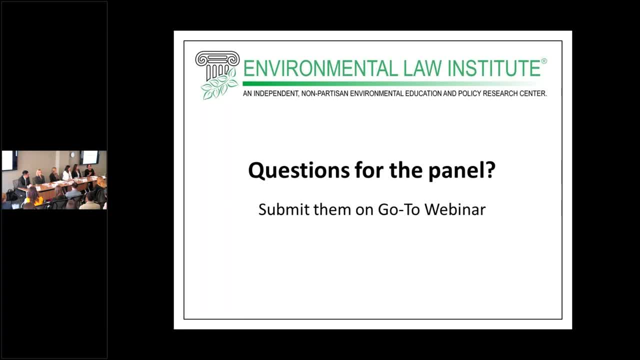 on our communities, because I'm all about living the life of impact. That's who I am, That's why I'm here, And so that's a little bit of how I overcome Kendra. thank you so much. I really appreciate you sharing that. 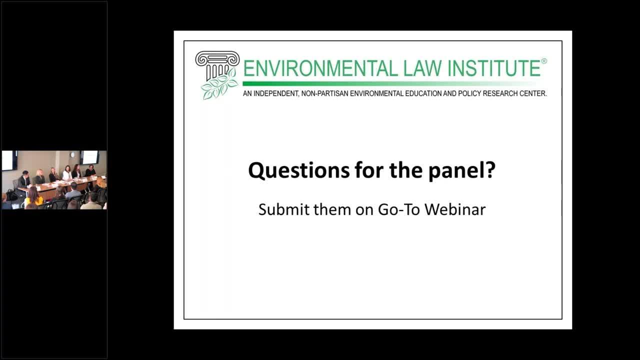 Definitely a great lesson in facing adversity, And thank you for that question. Do we have any other questions for Kendra before she has to depart? Thank you, Thank you so much. We will now open things up for questions for the rest of our fantastic panel. 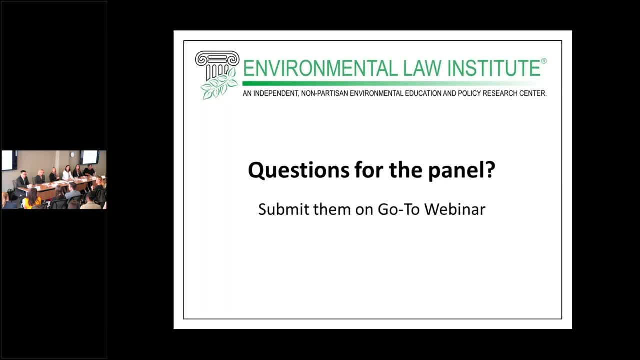 Do we have any questions on the web we can set up? Yes, Actually, we have one for Rachel and Toby in regards to how did you know law school was right for you And how did you know that you were ready to apply and attend law school? 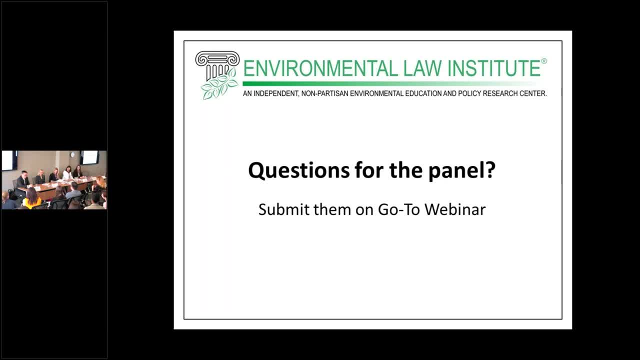 Do you want to go first? Well, I'm probably going to. I'm going to be franker than I probably should be. I just kind of went to law school. I think my mom told me like I should be a lawyer. 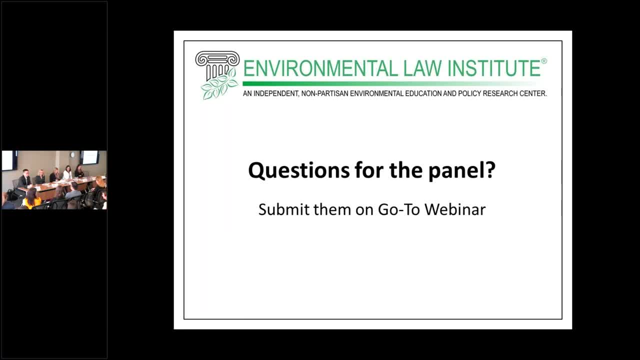 because I argue with her really well. So you know, I again. I think the theme, one of the things in my presentation, is that I didn't really have this environmental career well plotted out. I think I went to law school with the intention. 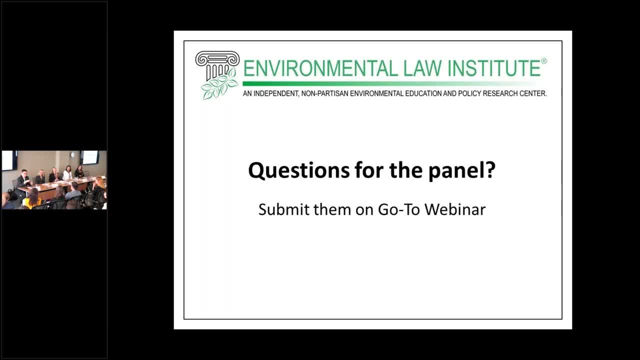 of eventually working in a field with the intersection of law and science and help formulate policy with the understanding of both, And that's not how things you know turned out. If anything I think I had I suffered from a bit of a lemming mentality. 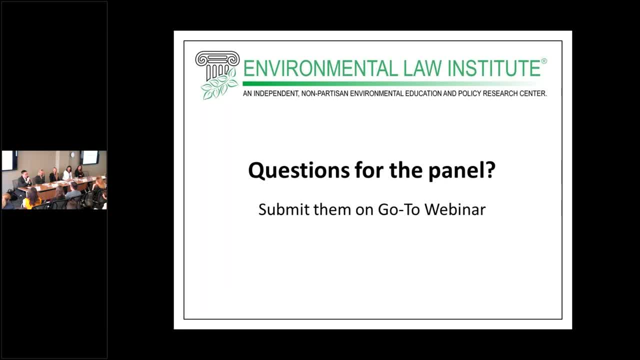 of just sort of like going along, And I would encourage everyone else to just sort of be a little bit more thoughtful and a little bit more intentional and taking more advantages of the opportunities that present themselves, so that you don't have to, you know, spend eight years. 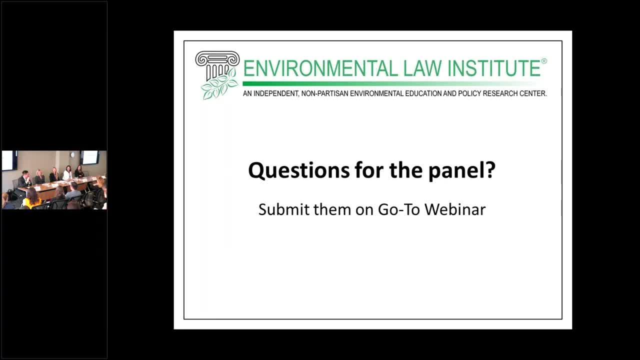 trying different things and figuring out things on the fly. I think I was the opposite. I knew I thought I wanted to go to law school as an undergrad, but I decided that it would be best to take some time off and think about it. 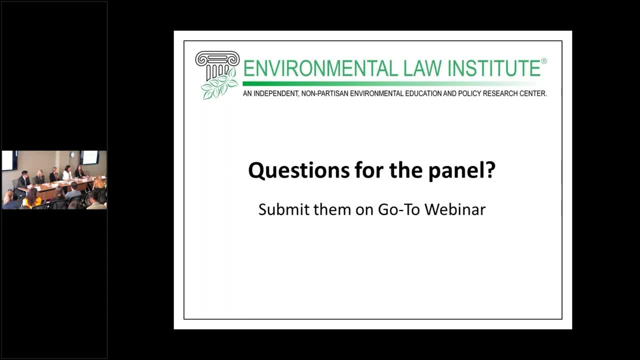 and think about other options. I knew I wanted to work within the environmental world And I knew I didn't want to go like hard science throughout, but I was having a hard time choosing between like environmental policy versus going to law school And in the end, 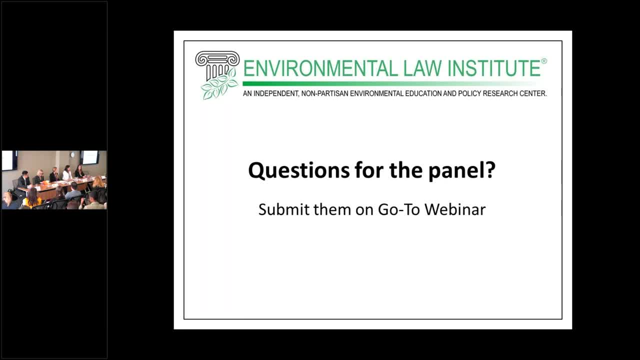 I figured that law school kind of gave me more options of the directions I could take And that it would be a worthwhile investment. because of that, A lot of people go to law school and then go directly into policy or, you know, a lot of people go into urban planning. 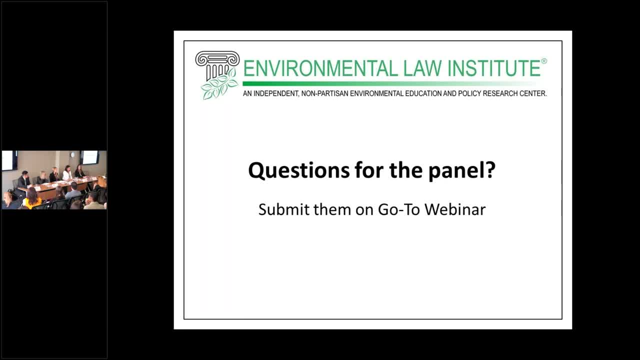 There just was so many more opportunities, I thought they would come with law school instead of going to get a master's in something that was very specific, And so, after taking some time, I decided, you know, that would probably be the best choice for me. 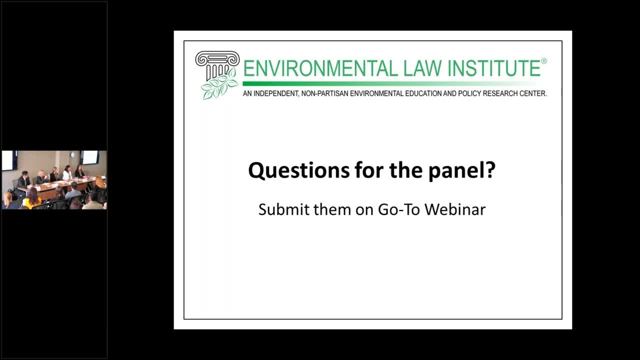 And it is. there's a lot of anxiety that comes with the decision because most schools are really really expensive And unless you're, you know, are very lucky, it's a lot of debt. But I will say that there are quite a few law schools. 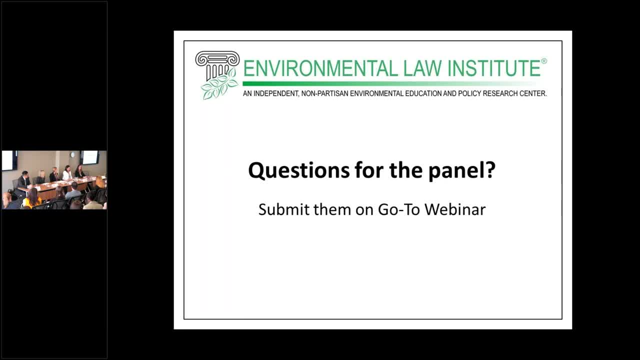 that have programs for people that know they want to do public interest law, Like Georgetown has the LRAP program where if you're working at a nonprofit or an agency, it doesn't have to be federal, it can be state- they will give you money. 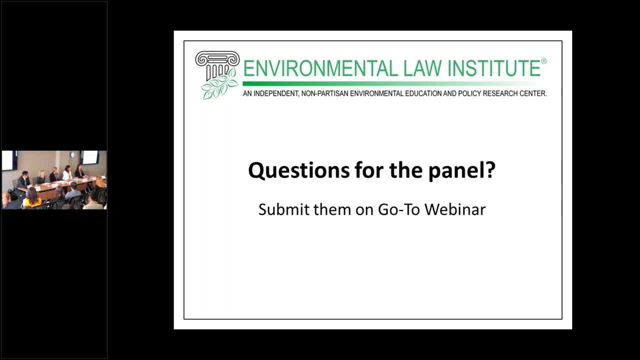 to make your loan payments for you until you make a certain amount of money and then it slowly goes down. It's like a scale, basically, And knowing opportunities like that, I think, is really important before you go to law school, because it is a huge. 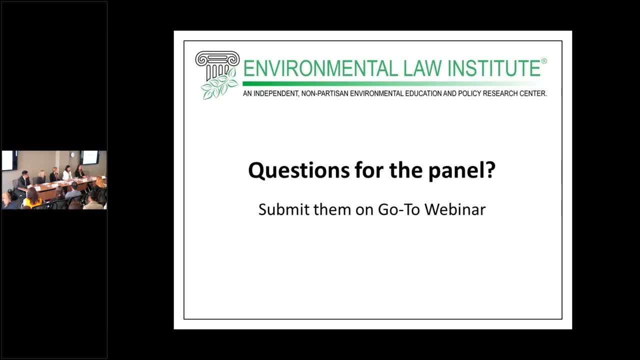 financial responsibility. But I knew that since I wanted to do public interest law, as long as I was able to get a job, I went to a school that would help me financially do that after I graduate. And then I'm also in the federal loan forgiveness program. 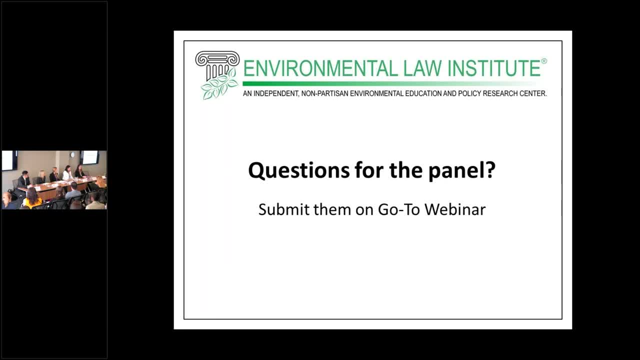 So after 10 years my loans will be forgiven. So just kind of doing that kind of research beforehand I think helps make the decision. I think in Atlanta I'm really happy I went to law school and I think that I had 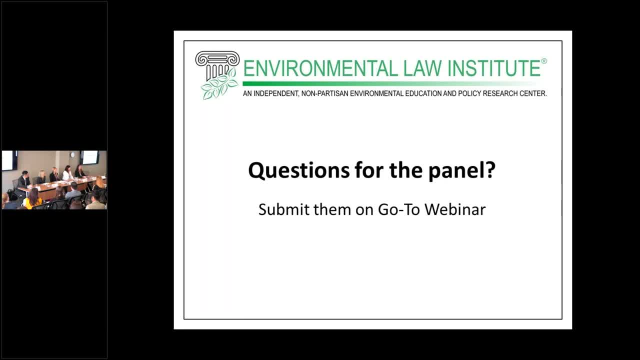 I didn't love law school. I think some people actually genuinely really do- and I found it kind of a hard environment to be in. like cold calling is not great, But then as you get past your first year and you're able to do stuff, 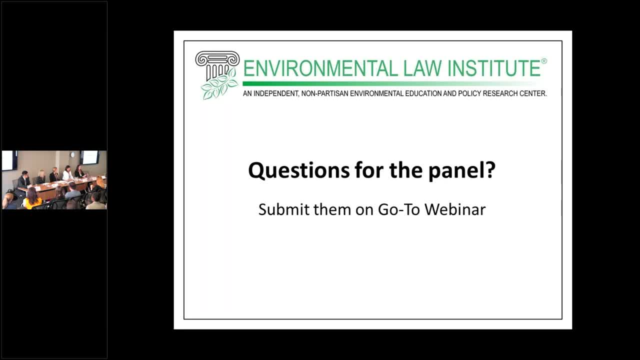 that you're more interested in, like clinic and internships, and you find your group of friends. it's not. it's, you know, I don't. everyone has different experiences, but it's not like the first three years is absolutely horrible. 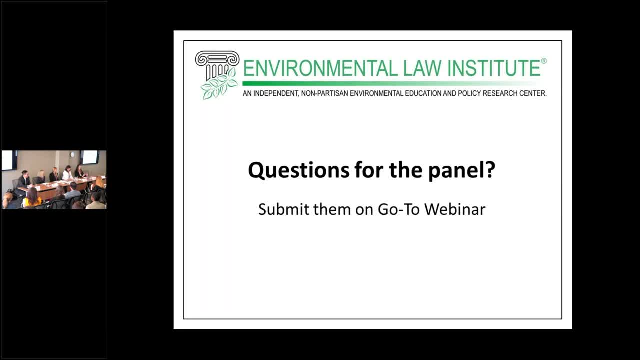 If it's something that you know that is you're, you are interested in, you think about the financial side of it. I think that it can be a really good, worthwhile decision And it's given me a lot of different opportunities and career paths. 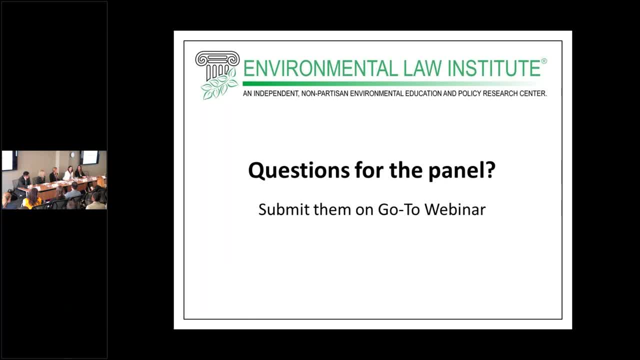 that could potentially go down. Yeah, Weirdly, I'll actually comment on the question And I think I've been in and out of, in and around lawyers for most of my career And I think that well, it's not that you can ever know. 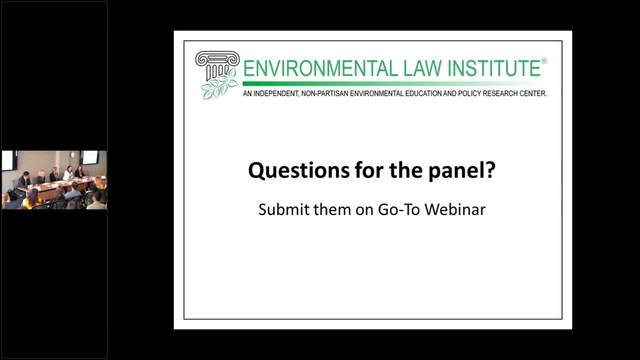 what you want to do at 22, unless you're Rachel, But I think the only thing that I've ever found has been closed off to me by not having a law degree is technically being a lawyer. I will never be general counsel And I generally have. 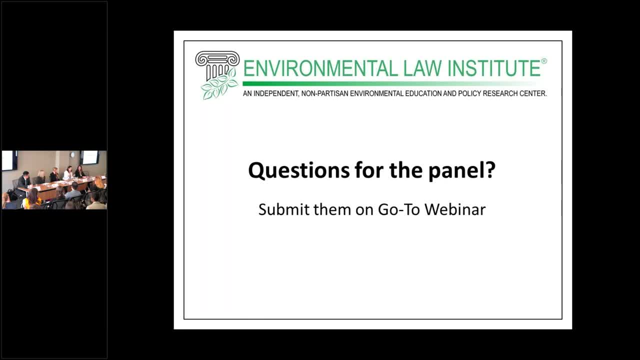 you know, any legal briefs I write are, you know, reviewed by a lawyer and that's good for everyone involved. But I think that kind of those technical like, if you like, Toby's friend, if you know you want to be a litigator- 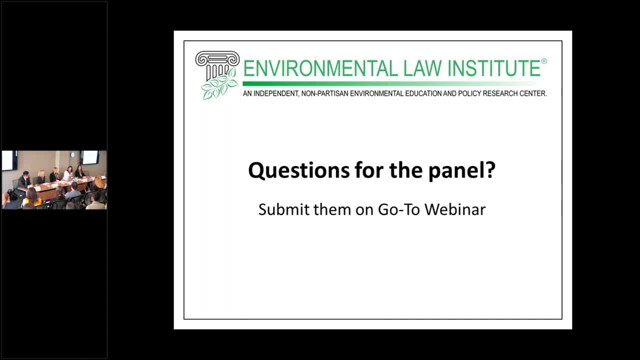 you probably have to go to law school. If you know you want to be a lawyer, you probably have to go to law school If you know you want to be a lawyer. if you're just generally interested in policy, you know, try it out for a while. 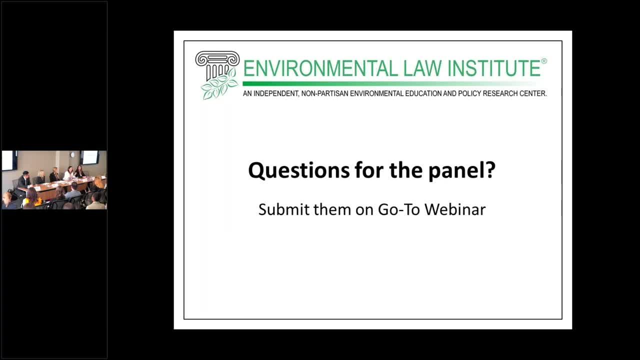 Like: go work on the hill, Go, you know, intern at Earth Justice apparently. But I think that that's one thing that, for better or for worse, was mis-sold to a lot of people of Toby's and my generation. is that to do policy? 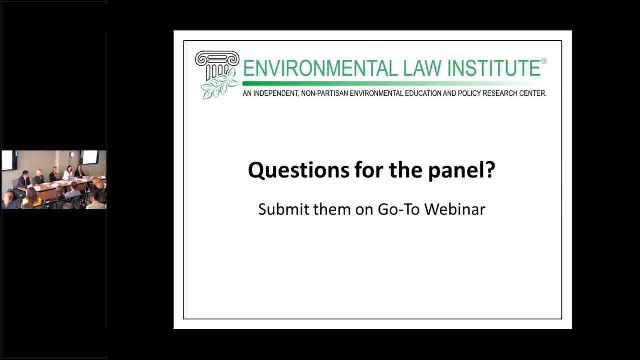 and to be in the world of making law. you had to go to law school and I just didn't have the money. but it turns out that's not true. Thank you all. Do we have questions in the room? So this question is for Toby and Kathleen. 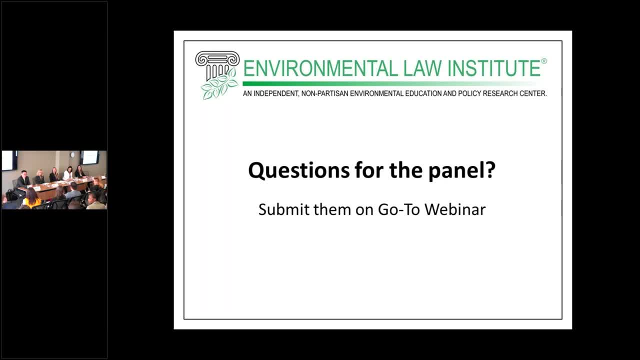 When you're working with clients or co-workers that have corporate or business backgrounds that may not have historically considered the environment as their primary as they're making decisions, what advice do you have on how to encourage those people to consider either environmental risks, what you do? 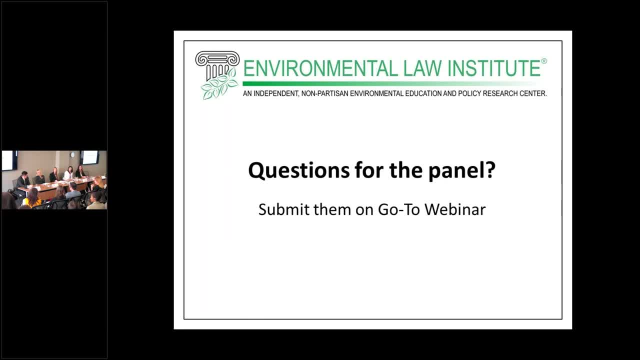 or environmental incentives. The short answer is: put it in money. I mean, I obviously work with a lot of people who, you know, wouldn't know it for sure if you smacked them with it, but I think being able to, and that's a really 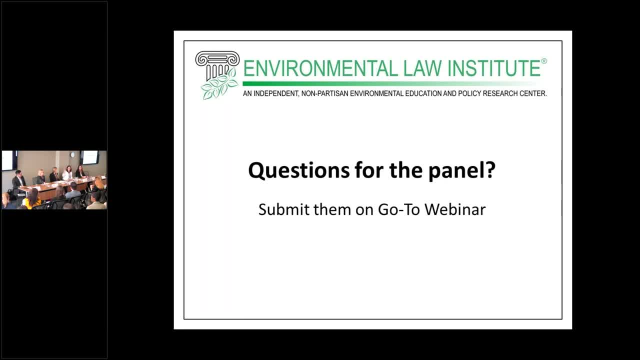 it took me a while to learn to speak it, but like changing how I would say we should have a, you know, EPA should have a rule that regulates carbon, because the sky just doesn't resonate with everyone but saying EPA should have a strong rule. 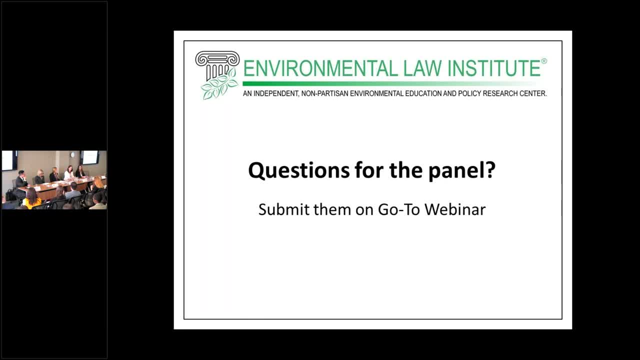 that regulates carbon, because we'll make a lot of money is. you know? I don't think that's the right way to do it. It does catch the kind of the business, the investment, like those types of people's attention and just learning. 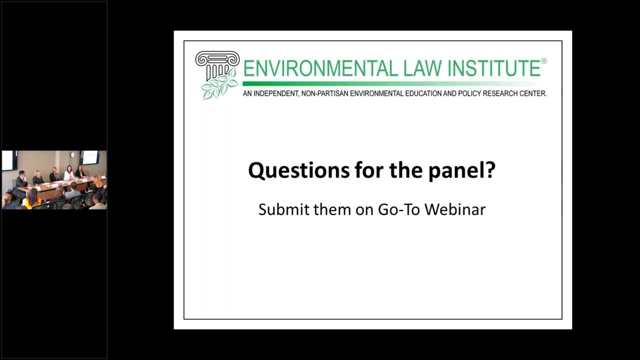 how to take. you know learning how to raise your audience and put it in terms that you know matter, not that you know money's all that matters. but in the corporate world, if you can't put it in dollar form, 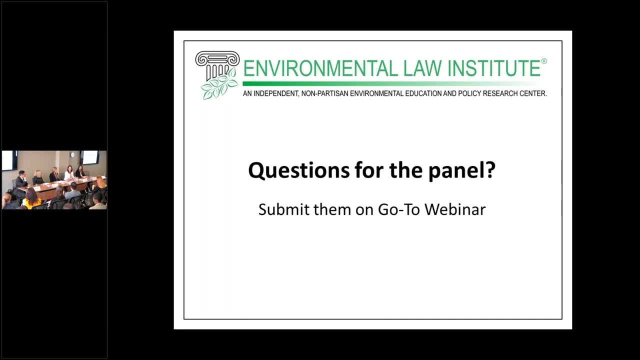 it doesn't matter. So saying that, like future generations and the atmosphere and everything you know, does resonate with some people, but a lot of other people you have to put it into. you know in terms of you know what's the value. 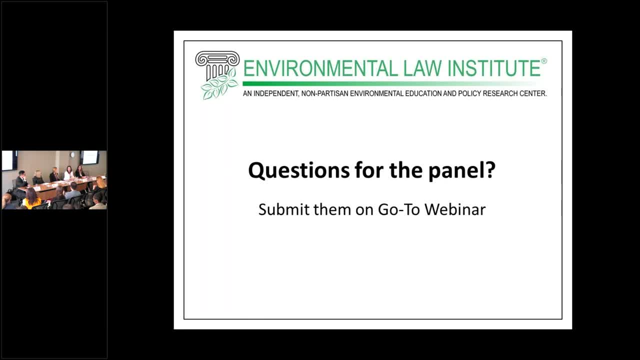 of a chair which I've learned to speak. That's been very hard. Don't discount the value of an MBA, but just essentially being able to put it, figure out what their metrics are and put it in those in them. Yeah, 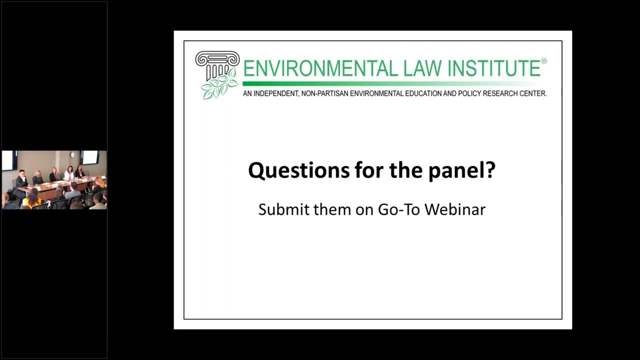 I would. I would agree. I think your ability to read the room and understand who your audience is and what their motivations are is very important. It doesn't matter if you think if something's important. it matters if you know they think it's important. 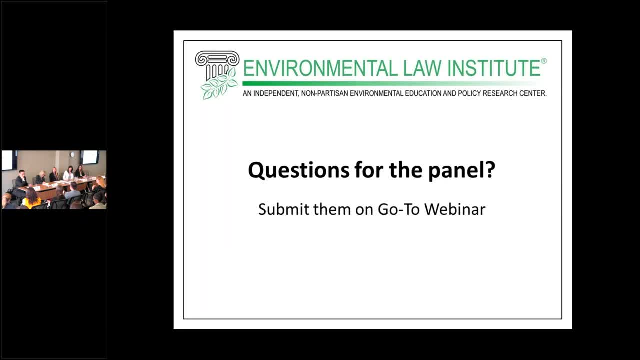 So one thing that I'll say is that, like you know, obviously on a, on a very environmentally intensive deal, on a, you know, a manufacturing target that uses a lot of hazardous chemicals and its processes, then environmental, you know. 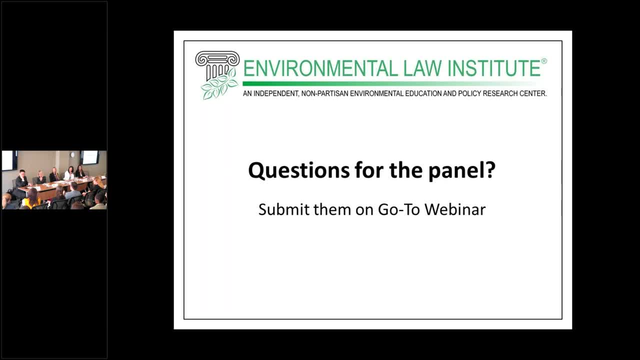 the environmental specialists are going to be very front and center and they're going to, you know, be on a lot of calls and negotiations and a lot of direct contact with the client. So our firm is also really good at staffing us on the deals. 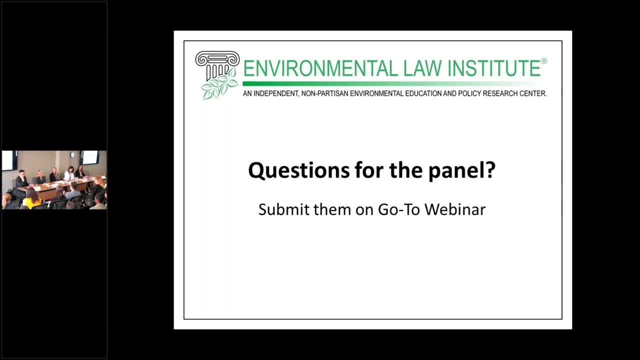 that don't appear to be that environmentally intensive, for the most part because sometimes you there, you don't expect there to be an issue, but sometimes there can be an issue. So, for example, I had a deal where it was a software company. 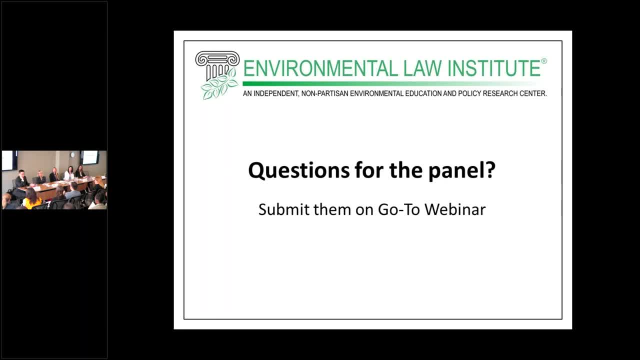 and just administrative operations and leased office space, and you know you wouldn't think that there's any environmental concern on that one, but it turned out that their headquarters was a former manufacturing facility that had been redeveloped into office space, and so you know. 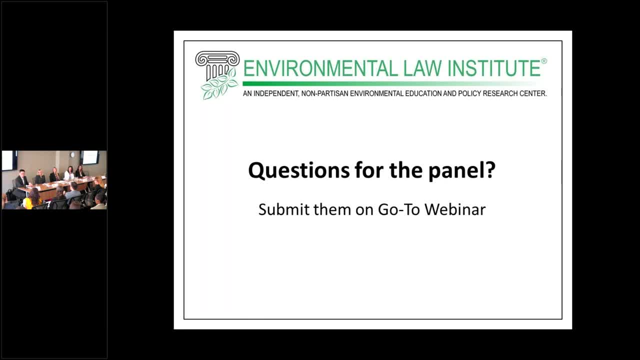 we're there to kick the tires and when you go into that kind of exercise you cannot bring your normal huge litany of all these environmental questions that you would ask, because either your client or even your own deal team are going to kind of get frustrated. 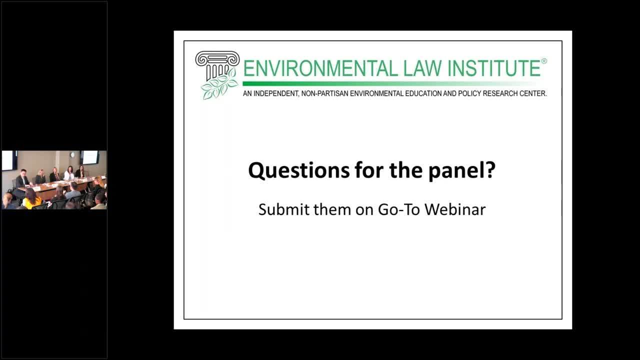 with you and say: you know this is not the right approach. but so you scale back, keep it very focused, you're kicking the tires and you're asking just as many questions as you need to in order to confirm that there aren't any surprises. 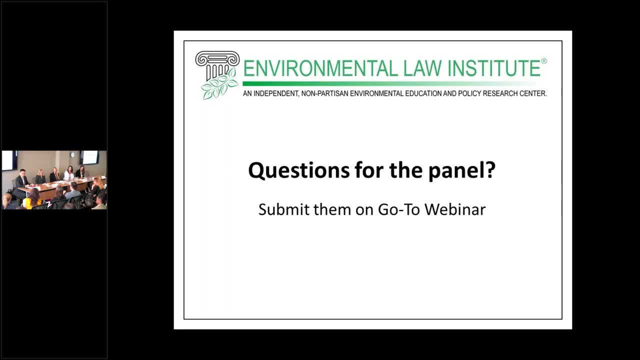 So I think you know it's very important to sort of tailor your approach. One other example I'll give is ESG. ESG is becoming a very hot topic these days and you know for the most part it's not. 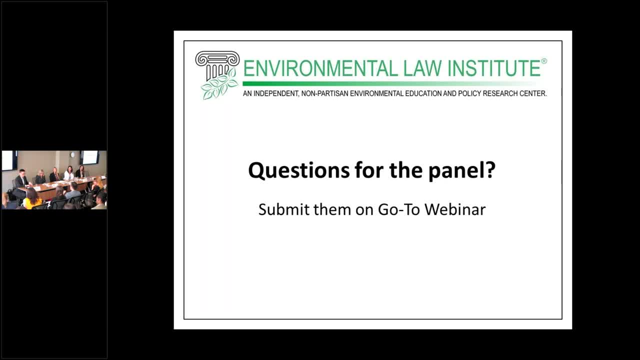 a growing movement, but it all sort of started where you have these. the private equity funds care about it, primarily because they have investors who care about it, and the investors will say: what are you doing in terms of evaluating ESG of the businesses and what are you doing? 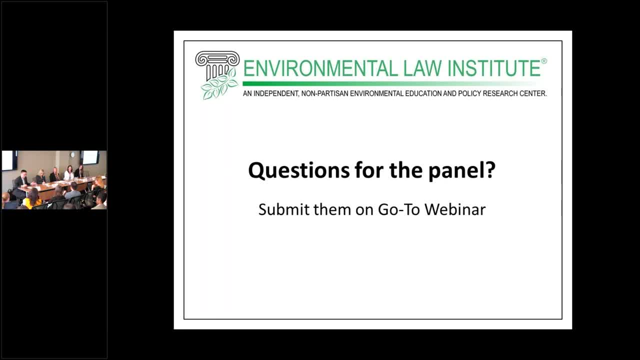 to improve it. So it's been largely again kind of like: you know, money talks really, and so I think you know that's what I think is really important. So, Shannon, you've had a lot of experience. 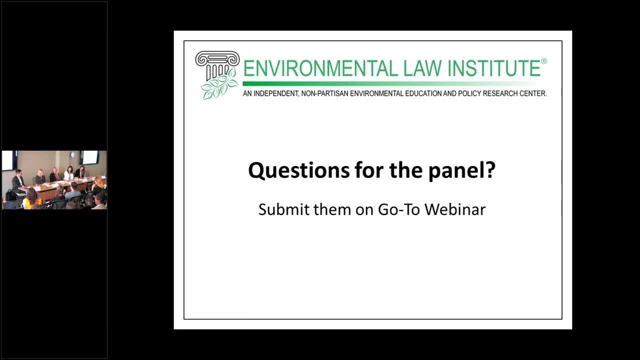 with you know, a huge variety of corporations. What would you add to this? I had the pleasure of going from a large publicly traded company to a much larger private company, and that company was able to create sustainable practices and really not have to worry. 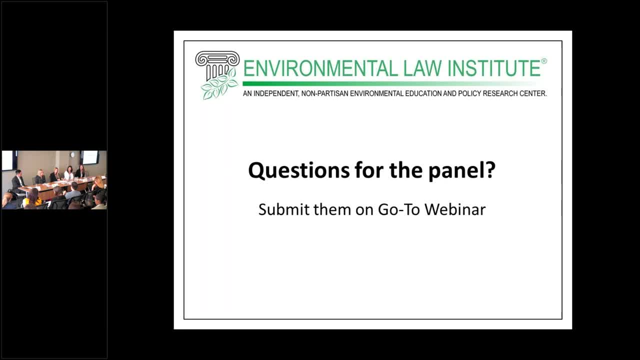 about the bottom line, which I think helped me understand both what a great opportunity that was for that company but also what a challenge it is for publicly traded. So in everything that company did, they really put you know. you talked about the motto. 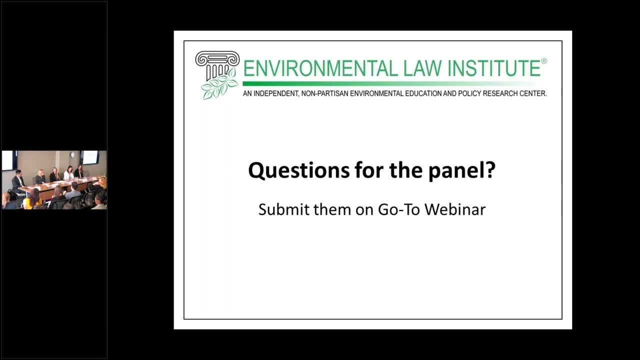 of ELI being people- similar phrase- and they really did that, but they also didn't have to worry about that. the shareholders are three people, So it was a quick conversation about what's the right thing to do. let's go do that, and 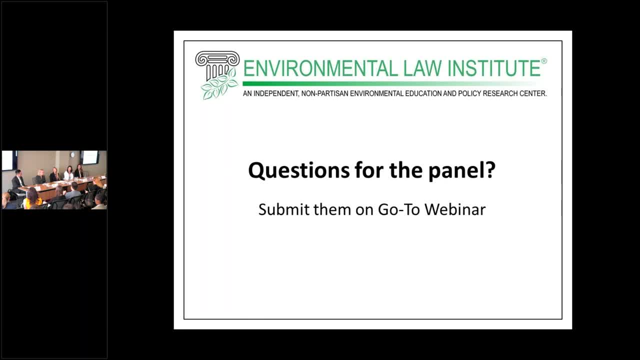 you know, bottom line be damned. we're going to be here in 50 years and we can take the hit and we don't have to worry about it. but it really helped instruct for me what a challenge it can be for publicly traded because you've got. 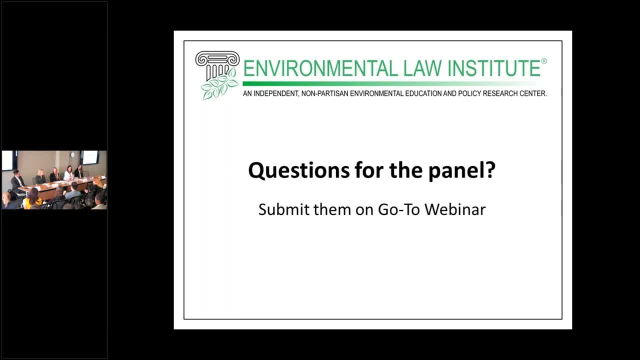 quarterly earnings and people you know yelling at you because you didn't make your numbers. Yeah, but we're trying to, you know, have healthier customers or do better things for the environment. and it's such a short, it's just a really. 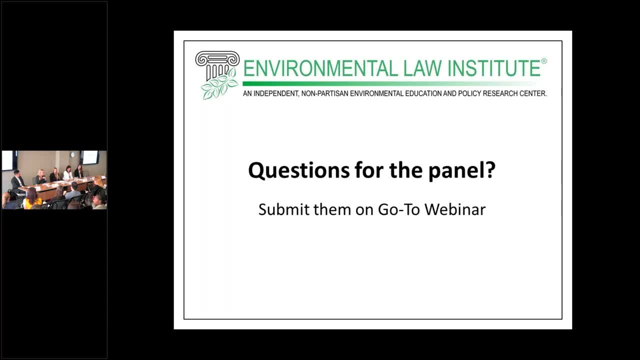 striking difference between a very, very long view of you know, 50 and 100 years to the next quarter. It was an interesting time And then, when you were with the group that was also very internationally based, did you see a big difference. 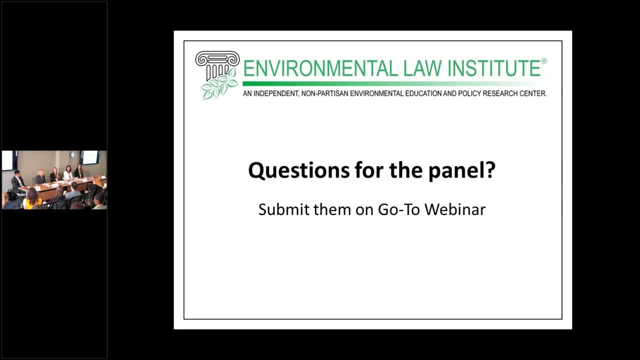 between kind of your experiences that were more domestic and a more international approach. The company had a very global approach overall and I did not really have line of sight into how the company dealt with specific policies in other countries because, again, because we were global. 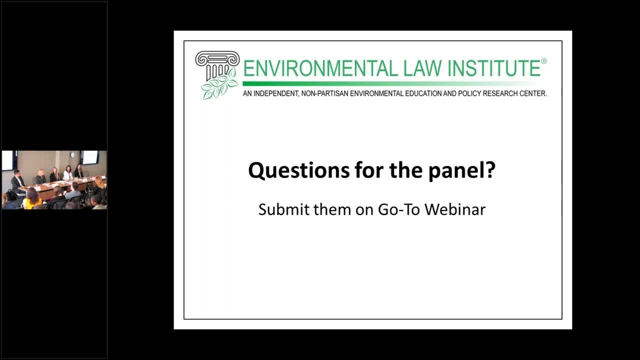 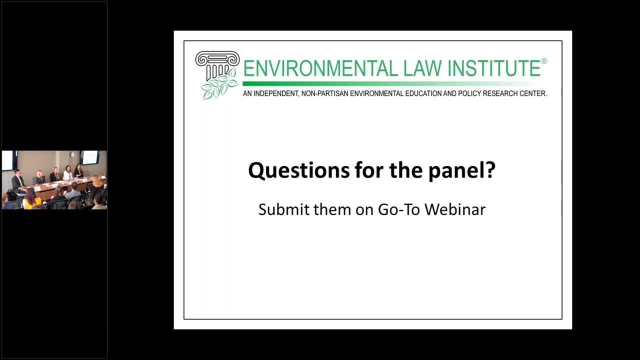 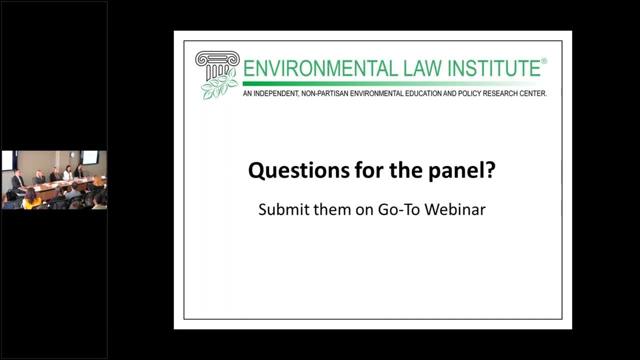 of sites, all of them in Latin America, So it was an international grand competition. I'm an environmental anthropologist and I also have a law degree from the UK, So I can't practice international studies or work with other countries because I don't. 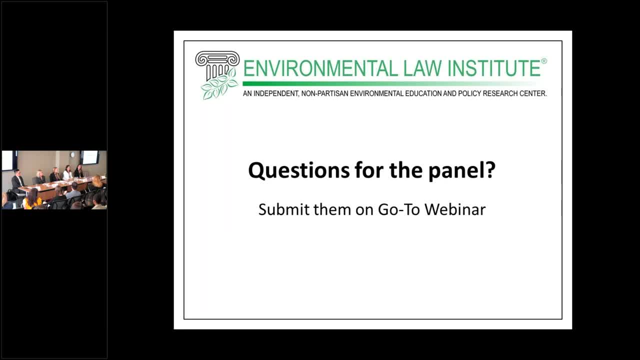 have the opportunity to do that. So I think that there are opportunities that are more internationally oriented. It's not doing something in that respect. I know that some of the programs that I've been involved in in the past have been really important to me. 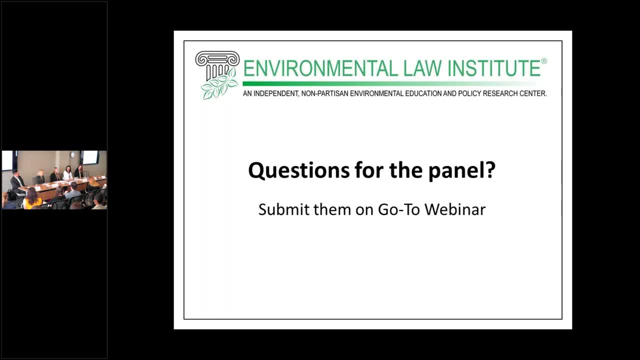 So I think that there's a lot to learn from the world and the environmental space. I think that there's so many NGOs with international presences that are also based here. There's UNEP and World Bank and so many different presences. 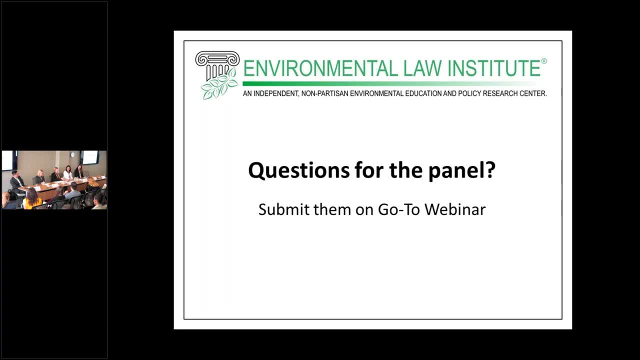 that we're really fortunate largely have such a big presence here. So I think that's really unique to- not completely unique to DC, but it's definitely a bit easier here. Yeah, one thing, not quite unique to DC, but better. 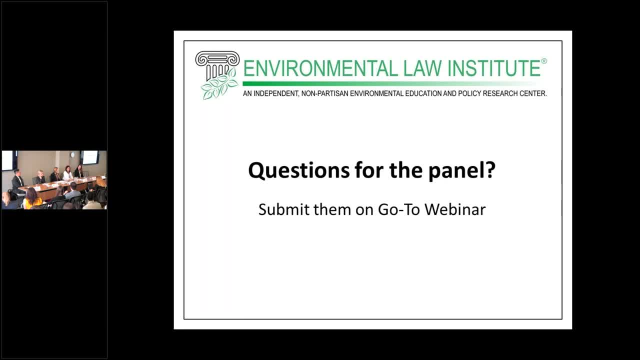 in DC is. I feel like our company has a lot of opportunities in the world that are dragging US companies forward on a lot of this issue. So I think international companies that have footprint in DC are another opportunity There's. 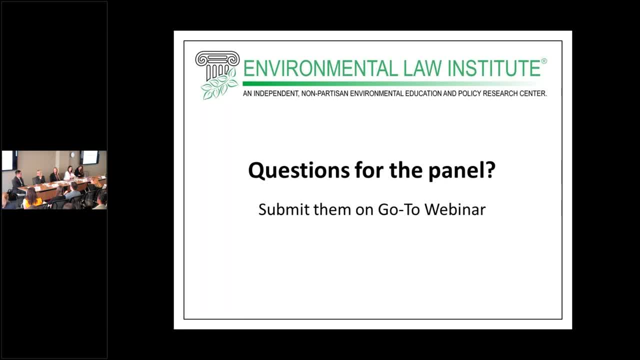 definitely an international environmental consultants that have usually local auditors in just about every jurisdiction and there's also often like a network of foreign counsel. So we'll be handling mostly the US issues, but then if we've got other organizations who are also available, 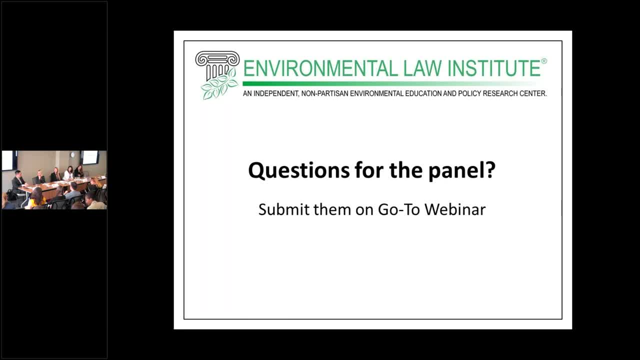 and we'll try to look at the big picture. but if there's something, a specific question in that particular foreign jurisdiction, you know obviously we're going to try to leverage the expertise of that local law firm to try to get an answer to. 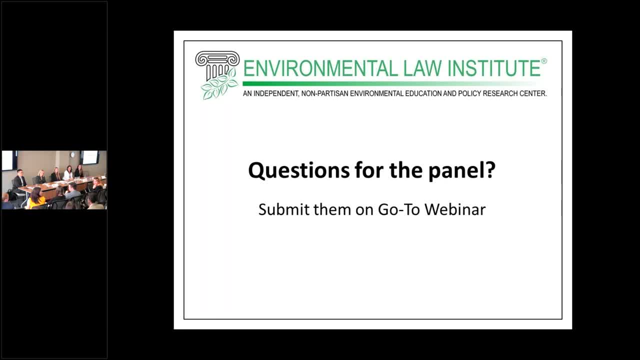 that question. So I'm going to ask a question from my fellow this year legislator. So thanks to Noah, But my question is for you, Shannon. I am from Alabama. Actually, I'm at the University of Alabama, about to get. 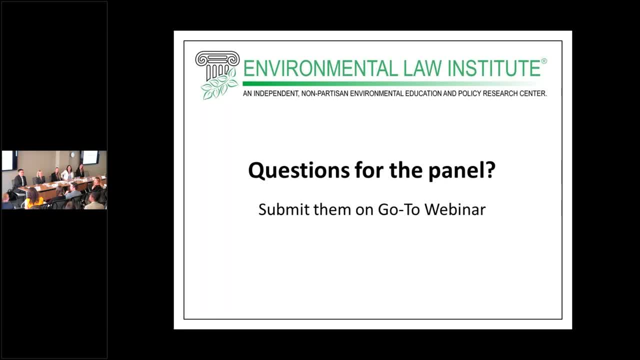 my doctorate to defend myself. I don't know if I'm going to get a law school, but I am interested in you know, the environment and helping like Toby and stuff like that. First, let's have lunch, Okay, of course. 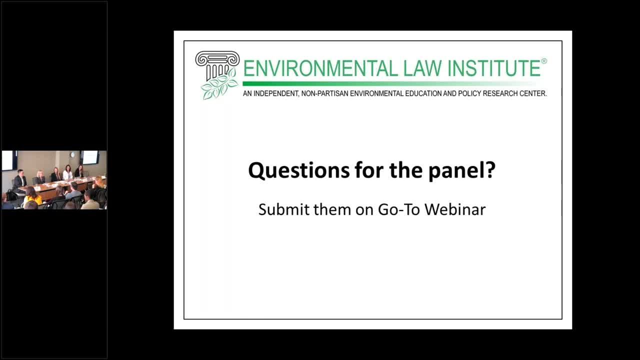 So I attribute it to just not being a jerk or anything like that. So you know, Kendra was talking about the different people in the office. So from the staff assistant that you made and you're a legislative fellow now, 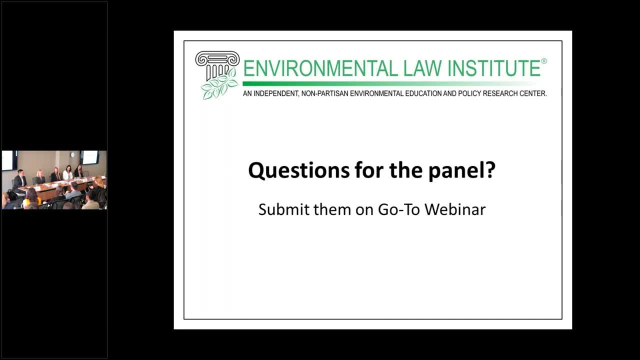 Okay, yeah, So you're making lots of friends. So it's from everybody, from the staff, to tell people. you know, here's my position, here's my client's position, here's what you'll hear from the other side. 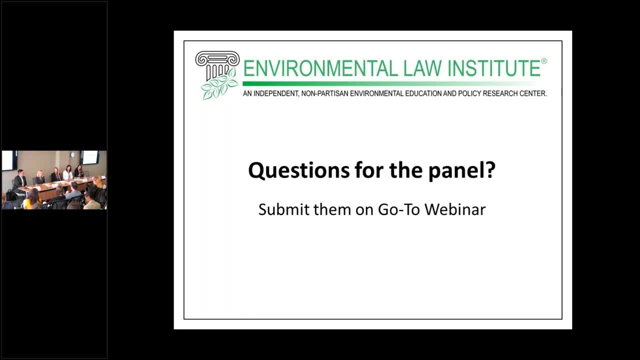 here's why I think we're right. You know, try to be as transparent and open and honest and friendly and nice and accommodating and not annoying as possible. and it you know I'm not particularly partisan, You know I happen to be. 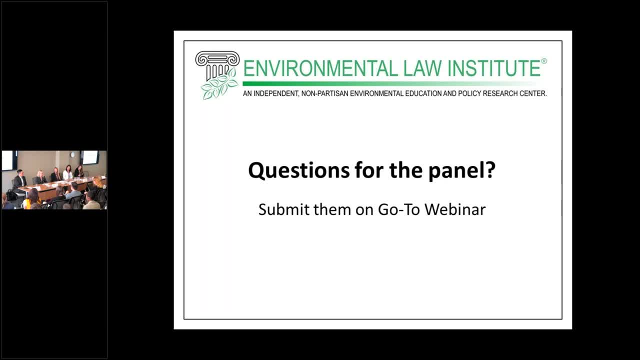 of one party, but I've had some of the best success of my career working with members of the other party. So you know I'm kind of post partisan like my party. when I worked at Safeway I used to say: 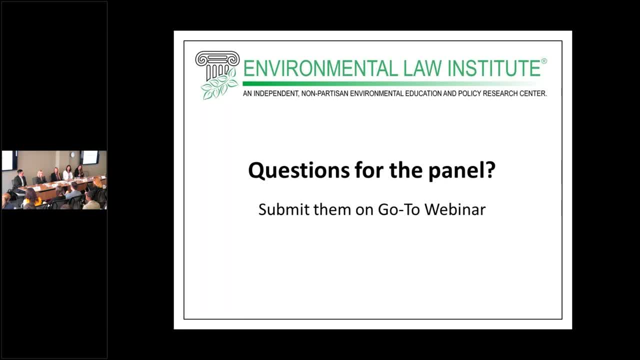 that you know, if there's an issue that you're lobbying that's purely partisan, it's usually geographic or has to do with some other issue. So I think that's, you know, just kind of longevity and sticking it out and hanging. 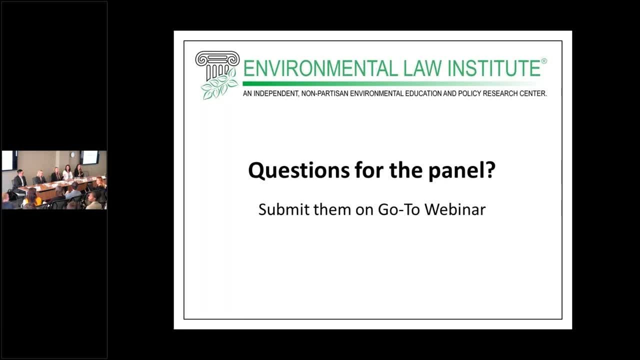 around is a good thing to do. Thank you, Sure Great Hi. So I think that some of you guys said that the general trend is that if you want to do environmental work, you don't necessarily have to go to an environmentally. 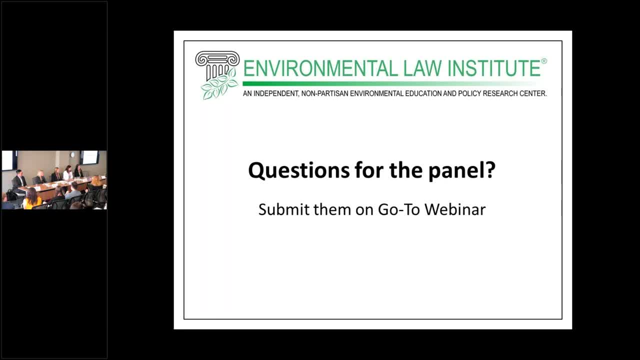 focused organization. There's private practices that care about the environment. So I think it's really important that you actually do meaningful environmental work. Well, who wants to start? You all do meaningful environmental work. I mean, I think some of it is. 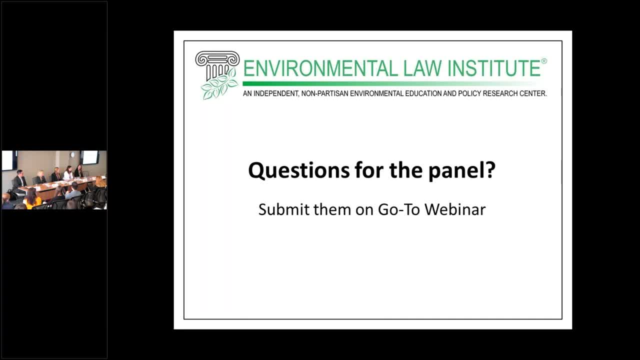 just you can't get exhausted. It's for better forest environment is often a popular guide. You can do anything with that And just I mean I'm definitely my parents are going to love that I was on this panel because my career. 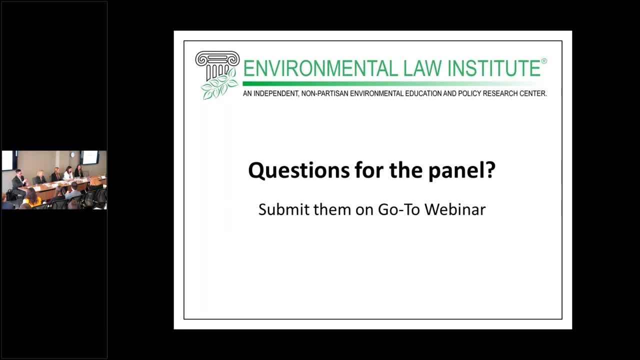 path did not look like a line, like more like a ball of yarn at the beginning. But just like you know, figure out, you know, get two years of experience if no one will hire you because you don't have two years of. 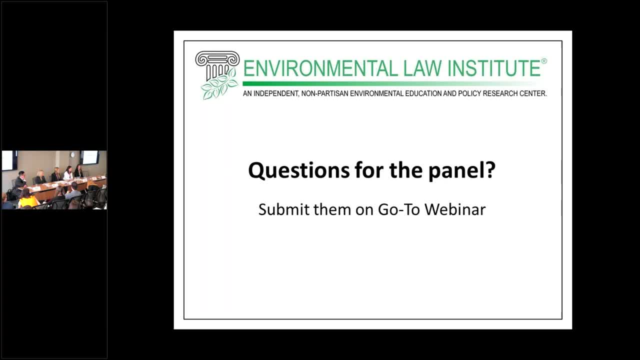 experience. It's a real feeling, you're not wrong. So you know, the hill is a really good place to start to get a little bit of everything If you can get in there. get in there young, they don't pay well. 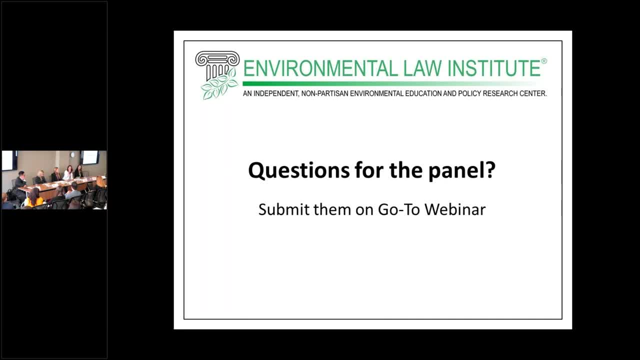 But I would add that everyone, for the most part, that you meet who's doing any sort of environmental work is passionate about the environment in some way or another, And if you can really let that fuel you and inspire you and be tenacious, as Shannon was saying, 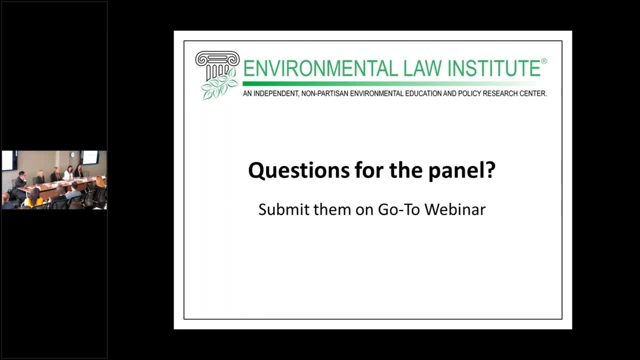 about finding opportunities and being honest and kind, then those characteristics will you know, you get to learn about all these different you know job opportunities you didn't know existed. I think that was really helpful to me right after I graduated- was just talking. 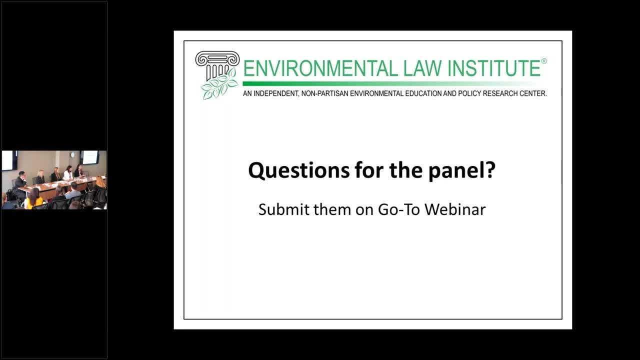 to a lot of different people that had different careers that were kind of tangibly related to what I was passionate about, And as you talk to more people you see a lot of different experiences that you had when you were in law school even probably. 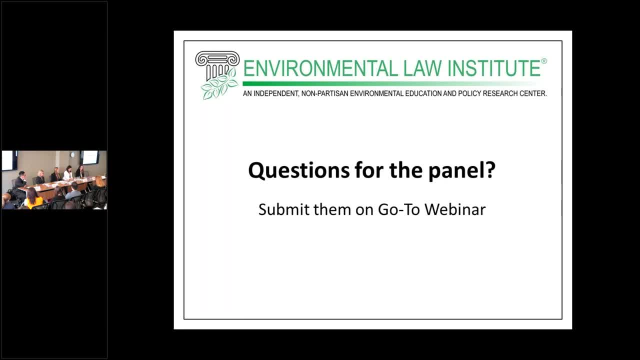 So I would say that I think the best thing you could do is just to continue to talk to people and learn more about just different experiences too, Because I think sometimes when you graduate, you're like, oh, it's really really hard. 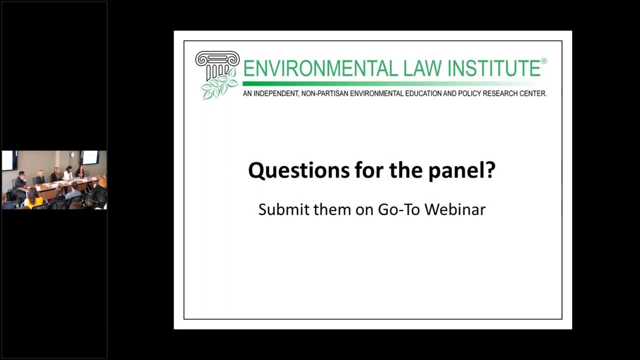 And so I think everyone around me was like: well, screw it, let's defer this pain and just go to more education, which I don't know. it's necessarily always the best thing to do. because you're not focused, It's hard continuing to. 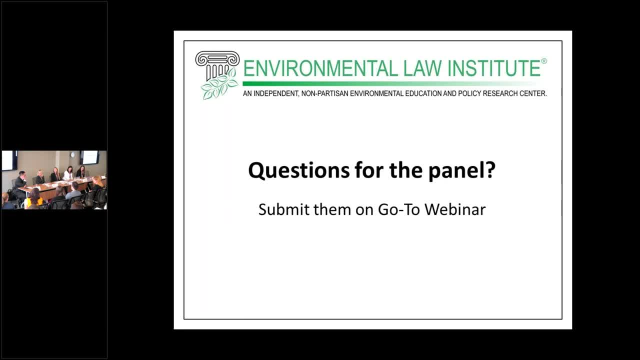 go to school. It's expensive. So I think the best thing you can do is just really you know, I think one of the traps that I fell into was just, you know, just try to be just very achievement focused, you know. 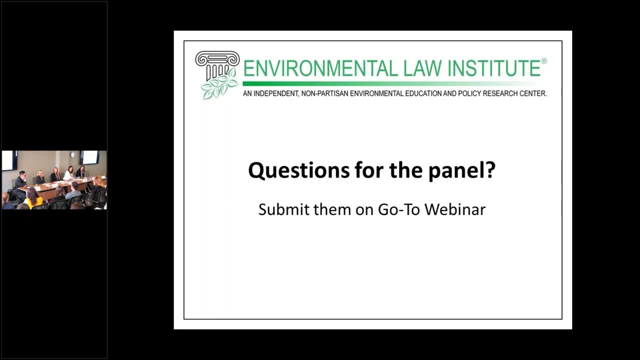 go to the best school you can get to take the best job that you can. But you know, I think, as we've talked about the tremendous variety of careers in the environmental field, there's no one thing that's going to change the way. 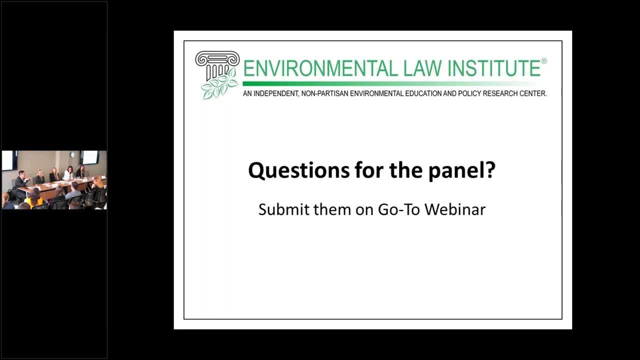 that you think about law, And I think that's one of the biggest challenges that we face in our lives, And I think that's one of the biggest challenges that we face in our lives, And I think that's one of the biggest challenges that we. 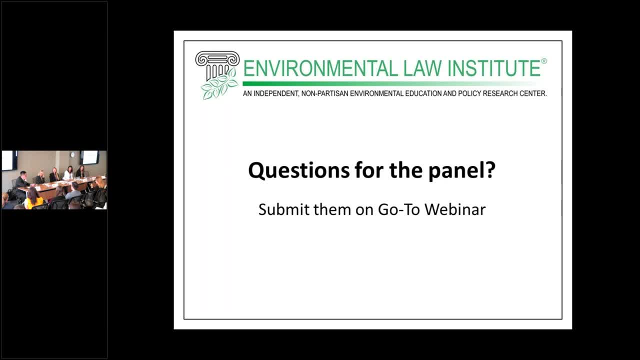 face in our lives, And so I think that's one of the biggest challenges that we face in our lives, And one of the biggest challenges that we face in our lives is that we don't have into that realm, because one of my classmates in grad school, um knew that her old firm had a job. 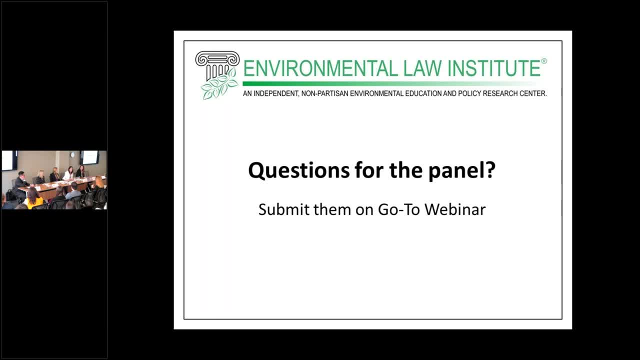 opening and put in a good word. for me, that's just. that's really how it, how it initially happened. um, and to make it also networking and light stocking: um. my last job in the pre the consulting firm i worked for before this. um, it's very small. it's one of those niche worlds where, in energy and 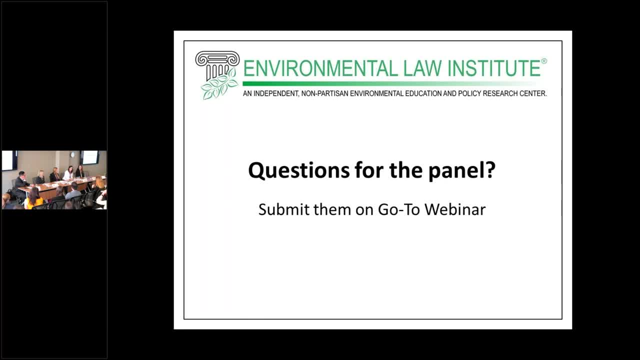 environment. everybody knows this company step, you know step, one foot outside of there. nobody knows this company um, but i found out who they were because i was living in boston at the time and had met a really interesting woman that had just been appointed to the puc there and was 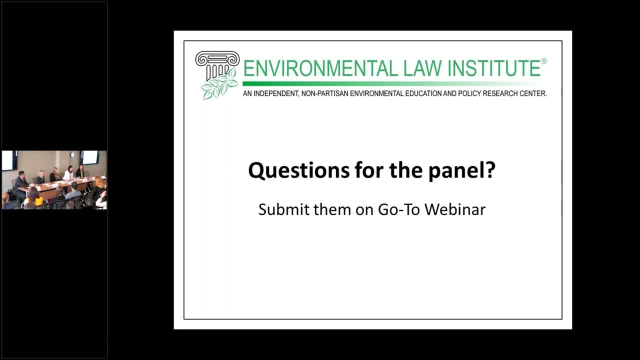 curious how she got to there in life and went through her bio and saw a company name i didn't recognize and googled them and they had a job opening and i got it and that's how i met all the people at exelon and made that move. um, which is definitely not something they ever teach you. 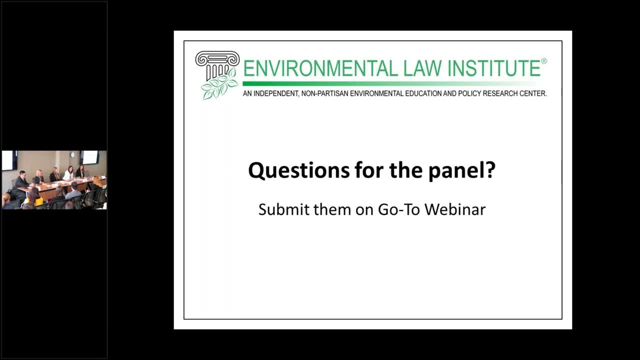 at the career center to. you know stalk people, but in some ways it is of like looking at some where someone that you think that is either doing something interesting now or somewhere you would want to be. you know, either ask them how they got there or the internet's awesome. 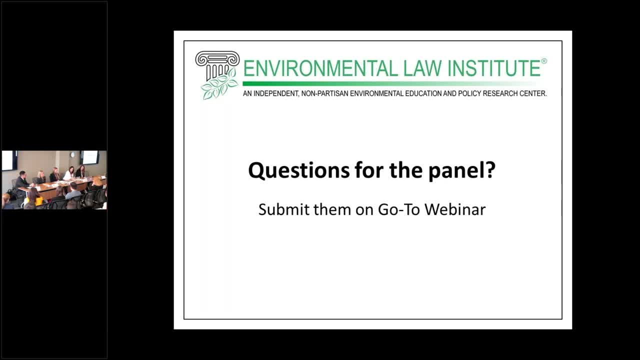 well. thank you so much to our participants for joining us today here in person and on the web, and for your thoughtful questions. we do hope that you will continue to think about the many opportunities and facets of careers in the environmental sector. we're grateful for your participation in the eliza annual summer school series. i hope that you have some fun and here's